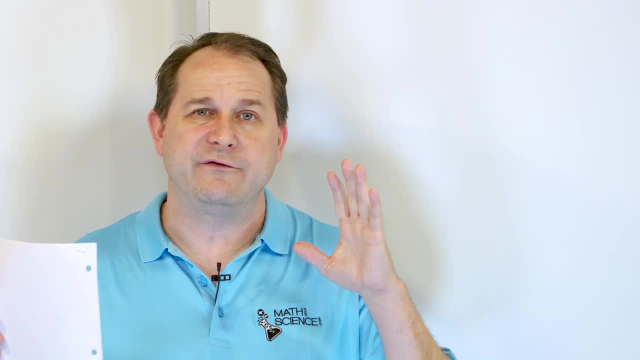 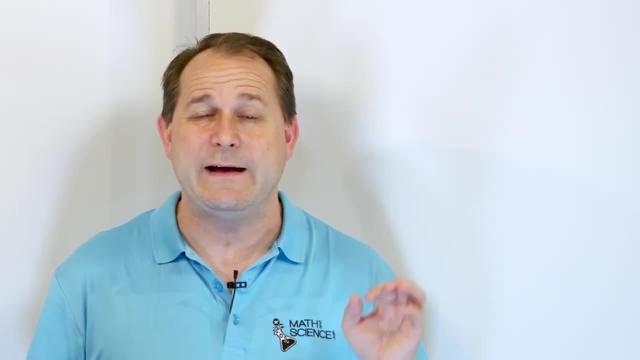 for sine and cosine, And then we'll come back into the board and describe a little bit of the theory and do a little more drawings to shore up our understanding, and then we'll solve our problems. The last thing I will say before we actually go and do the computer demo is: remember. 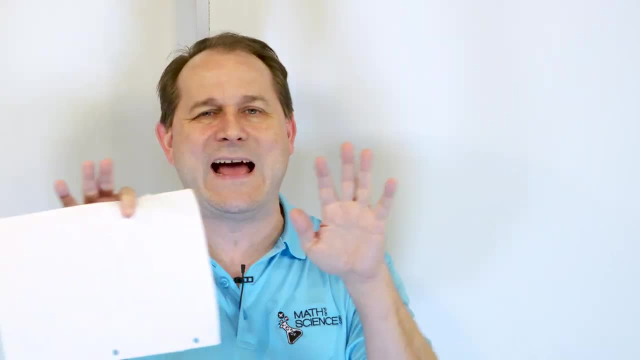 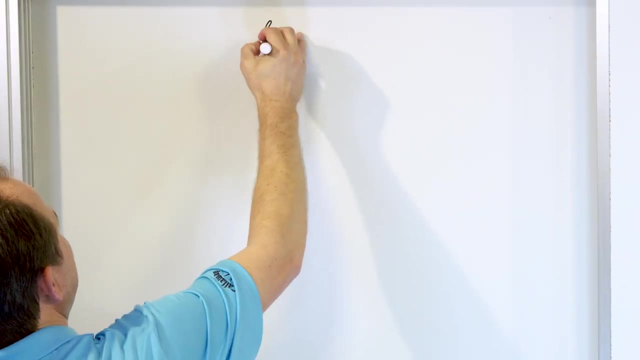 we already talked about how to shift any function we want along the x-axis. We've done that before, even a function like x squared, For instance. I'll just tell you real quick: if we have like, f of x is equal to x squared. 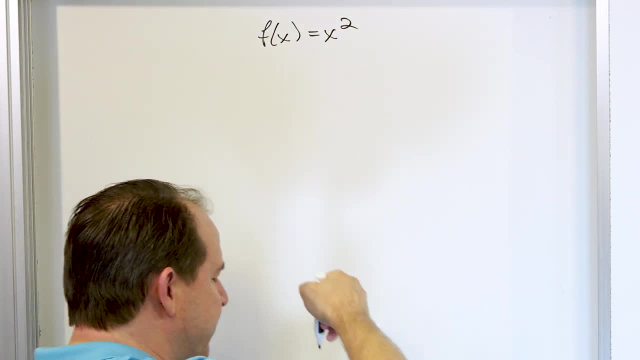 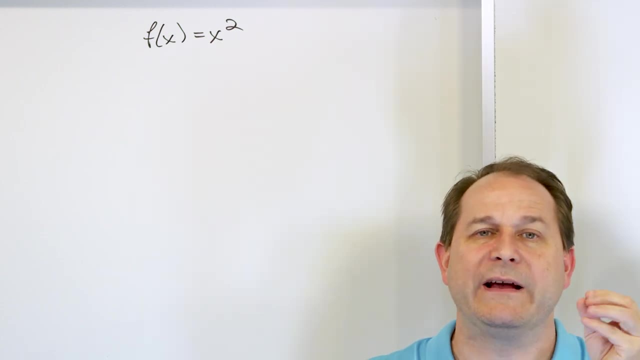 how do you shift that function? What you do is you replace the x variable with something. If you replace it with, you know, x minus a number, then the thing is shifted to the right. If you replace it with x plus a number, it's shifted to the left. So we're going to review. 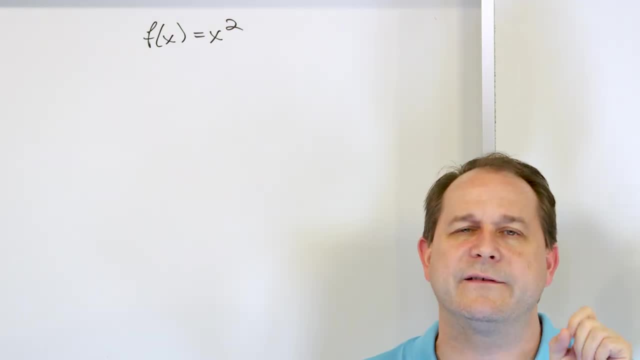 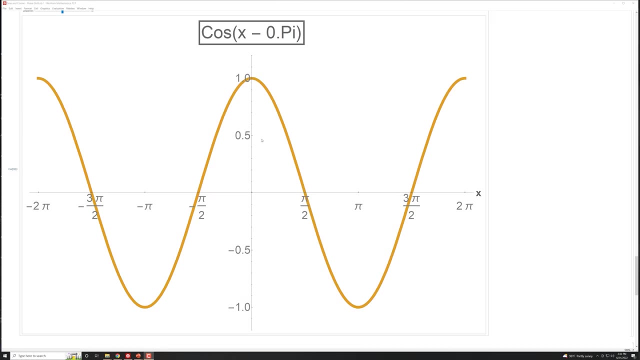 that as well. So for now, let's go ahead and just keep those thoughts in your mind. Let's go to the computer and learn how sine and cosines can move and propagate in space. All right, here we are in front of the computer. We have a standard cosine plotted, Starts at one. 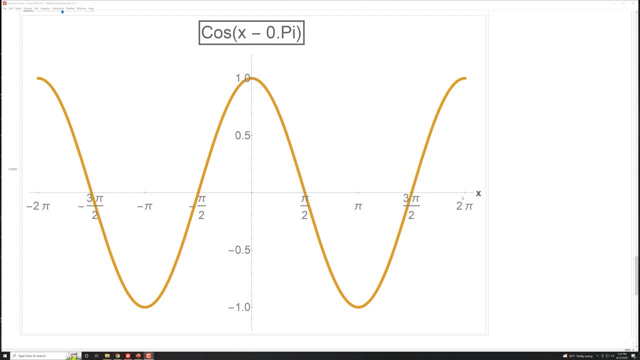 goes down to negative, one goes up again to its starting position over a two pi interval. So this is one cycle on the right, one cycle on the left. The function I'm plotting is the cosine function, but I've replaced the variable with x minus something. Now what I've got here is subtracting. 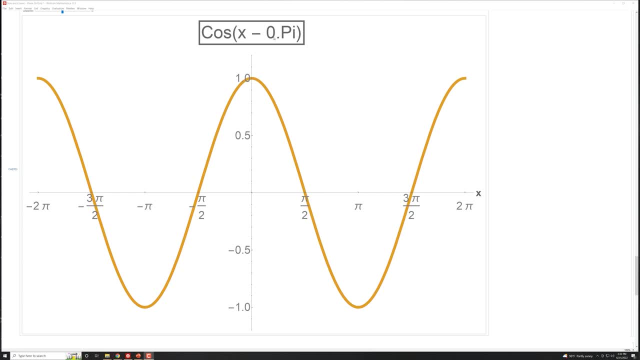 zero times pi, So really it's just subtracting zero initially, And so that's why it looks like an unchanged cosine function. So let's go ahead and do that. So let's go ahead and do that, Because this just goes to zero. Now let me just show you graphically what happens. 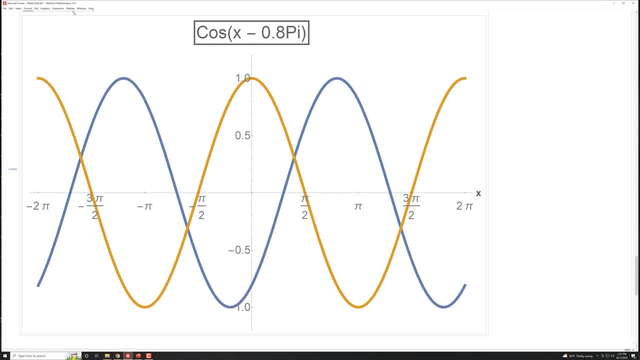 As I change the number inside of the cosine, the blue curve is plotting the result And as I continue increasing this number, you can sort of see the wave sliding to the right. And if you put your thinking cap on and really just like visualize it, if I drag my mouse with a constant 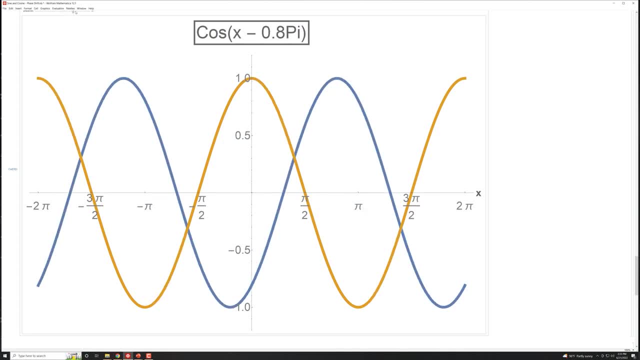 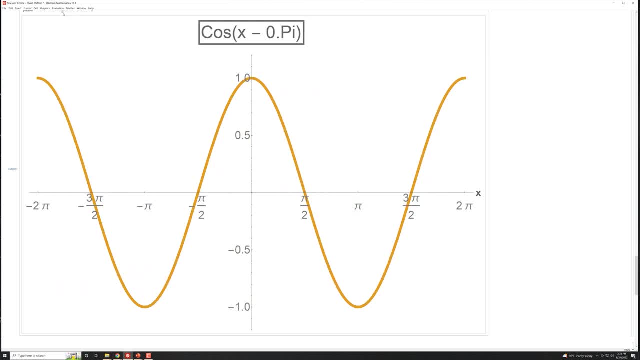 what it is. Now I'm going to show you how to write that down in a minute, But that is the reason we learned this: to be honest with you. So look at what's going on As you take x, and the argument of this thing is x gets replaced with x minus a number. Let's take a look at what happens If I 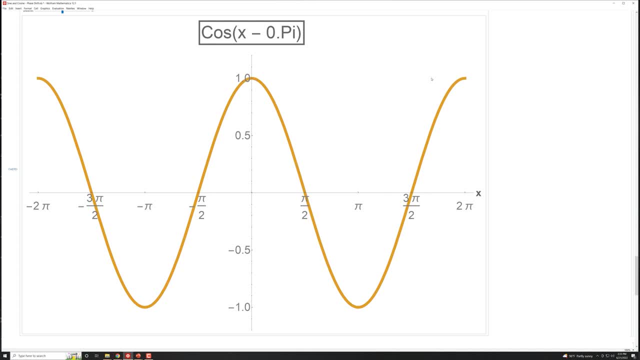 could grab this gold function and shift it all the way to the right by two pi. notice: two pi is a period of the function. If I could shift it right by two pi, then I would end up with a cosine that would look exactly like this one, because I would be shifting it. 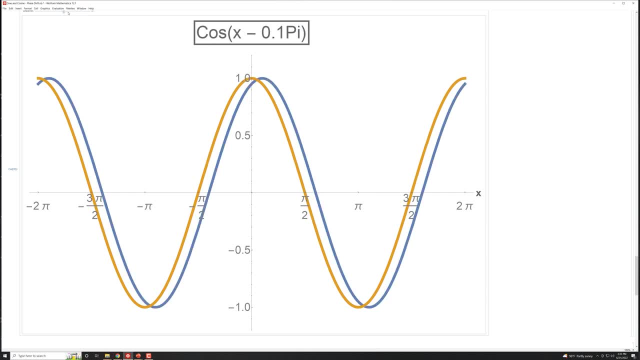 One period And so everything would line up. So, as you see, as I go through these intermediate values and end up where I shift it by two pi, notice we have x minus two times pi. Then we have shifted the cosine one complete cycle. So it lines up with the original function And what you 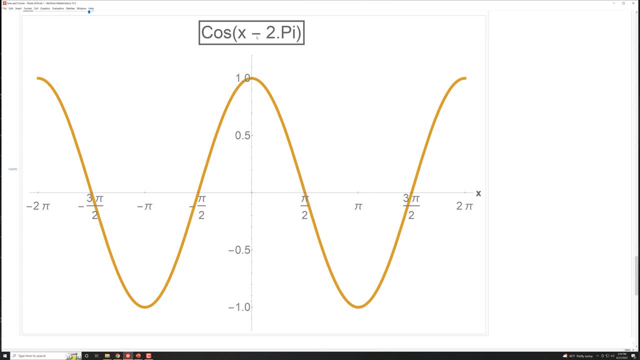 have is basically what you have started with. So when you shift the cosine to the right by one period, then you get exactly what you started with. Now let me go back to zero here. And what If we shift the other way? So when you have a minus sign in here, it shifts to the right When 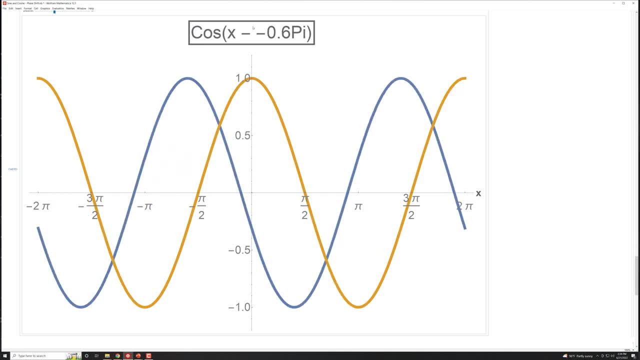 you put a plus sign in here like this. way it shifts to the left. Now notice the way I've written here. is x minus a minus zero point six pi. So this becomes a plus. So this is like x plus point six pi. And if I keep going to the left and shift it to x plus two pi, then again I get. 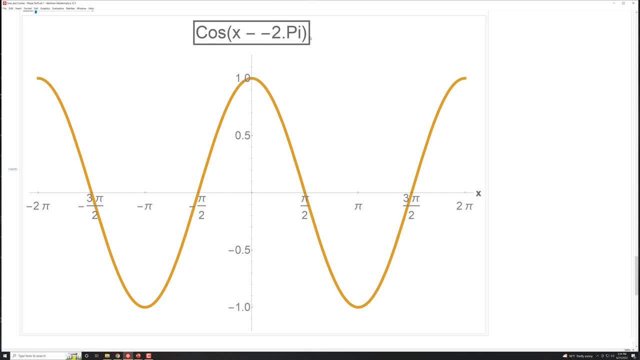 exactly the function I started with. So isn't that kind of neat The way the cosine and the sign work. if you shift it one period, either to the left, like it is here, or to the right, like it is right here, then you get exactly what you start with. Now let's go back. 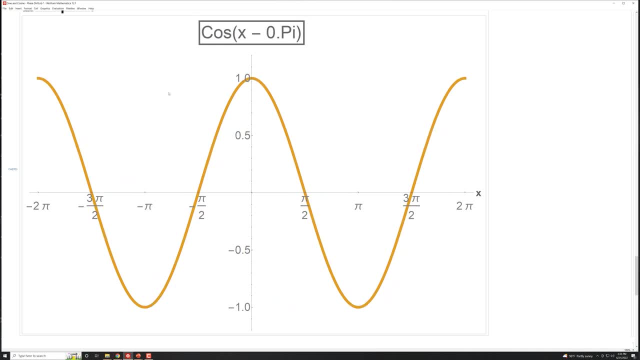 to the zero point. Instead of shifting it, one full, complete period. let's take a look at what happens if we shift it half of a period. So if one period is two pi, then half of a period is just one pi. So if I shift it, there's point one pi, point two, three, four, five, six, seven, eight. Let's 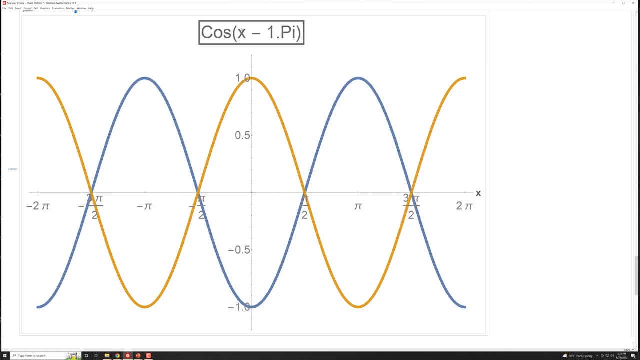 go back. It looks like I passed it up one pi, So here I've shifted it x minus one pi, So x minus pi. So I've done a phase shift where the blue curve is shifted to the right by exactly pi units. Notice: 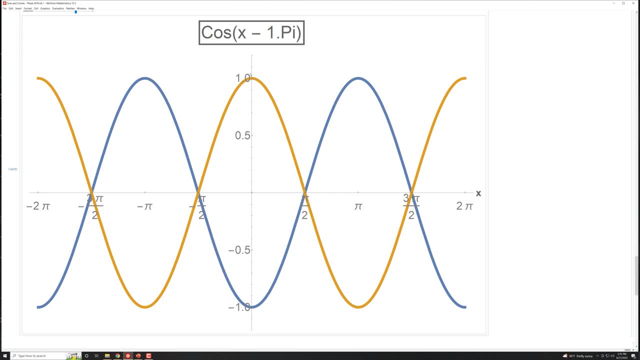 how it kind of like it becomes an inverted version of the original cosine function. Notice, the original cosine has a starting point here, but now the inverted, the shifted version, is exactly the mirror image reflection over the x-axis, So it maps everything down The gold. 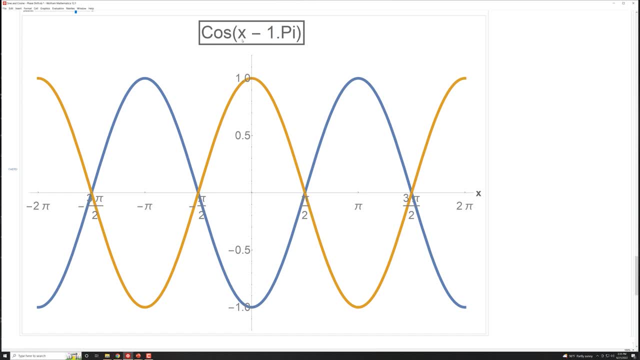 down here becomes the blue up here, and so on. So when you shift a cosine or a sine by half of a period, then it's the same thing as inverting and kind of flipping the cosine over. I guess is what I'm trying to say. So if you shift the cosine by a complete period where we shift, 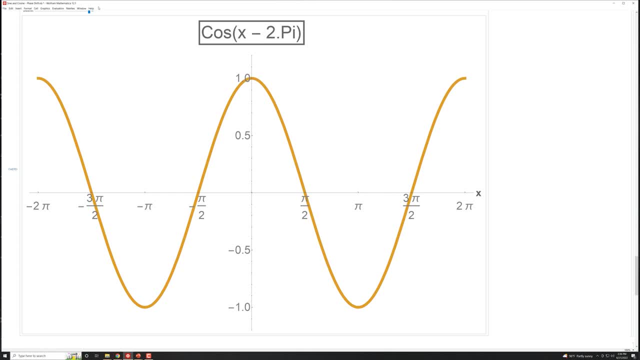 by x minus two pi, or two pi shift to the right, we get exactly what we start with. But if we only shift half of a period which is shifting by one pi, then we get this inverted version of that. Remember that, because I'm going to talk about that in the lecture. Now I want to show you. 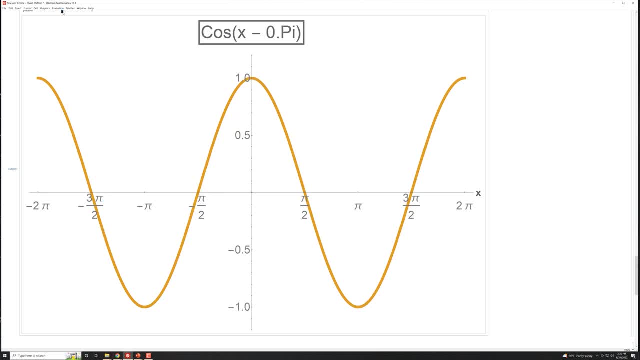 something else very, very interesting: If we go back to the zero point, let's say that we don't shift by pi or two pi, and we don't shift by pi, let's shift it by pi over two. Look at this right here: If I shift like that, that's point one, pi, point two, pi, point three, point four. 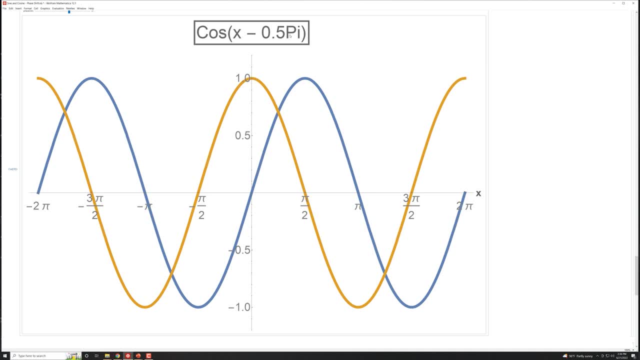 point five pi, That's shifting by pi over two, which is the same as point five pi. Notice the blue curve is shifted just a little bit to the right by exactly pi over two, because originally the cosine curve was a peak right here at the origin. But when I shift it by pi over two, 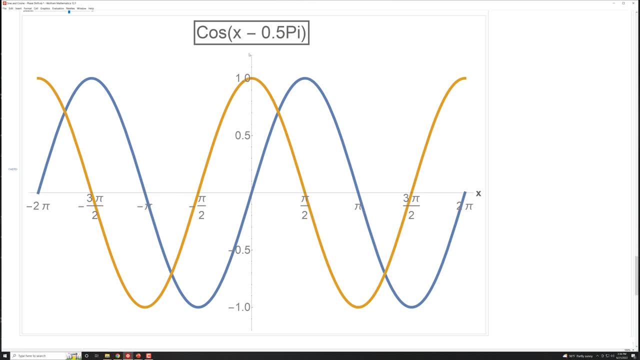 it's right here, at pi over two radians. So the blue curve is the shifted version when we shift by pi over two. But I want you to stare at this and look at this blue curve. What does it look like to you? See, the gold curve is a cosine because it starts up high, But the blue curve 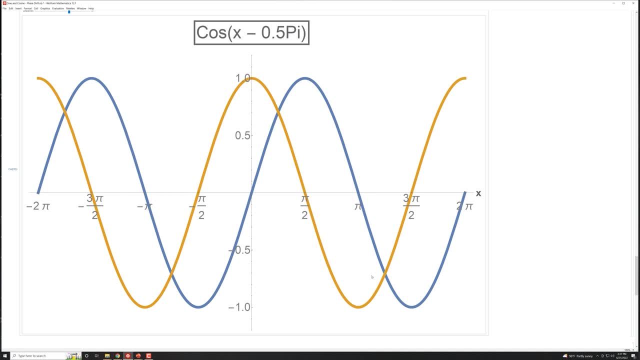 starts at the origin here, goes up to a maximum down and then again completes a cycle in two pi. The blue curve is a sine function. So you see, because the cosine curve and the sine curve have exactly the same shape, then if I shift it, 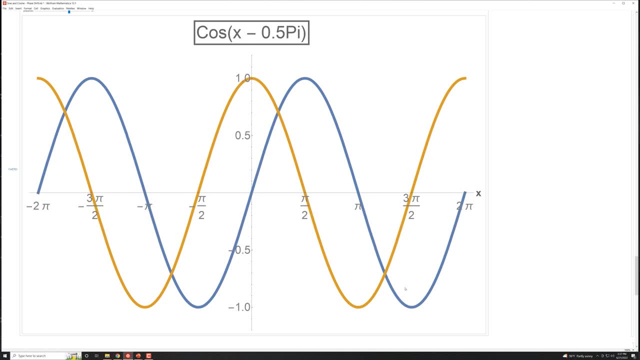 just enough, I can actually change a cosine into a sine function. Cosine and sine are very much related because they have the same range of values, the same shape. They're just a shifted version of one another. So really any wave that's actually propagating or traveling, you can write. 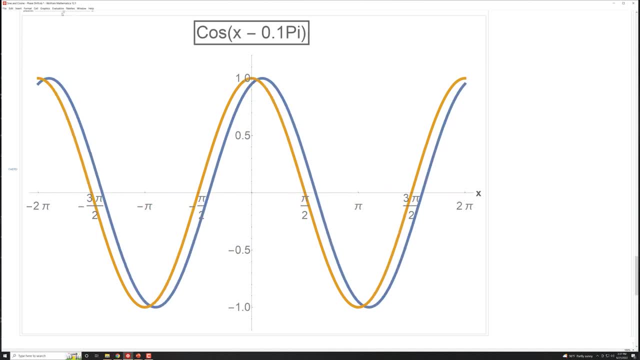 it in terms of a cosine function. You can also write it in terms of a sine function. Neither is going to be incorrect, because sine and cosine are cousins of each other. The only difference is that they're shifted relative to one another, so much so that I can. 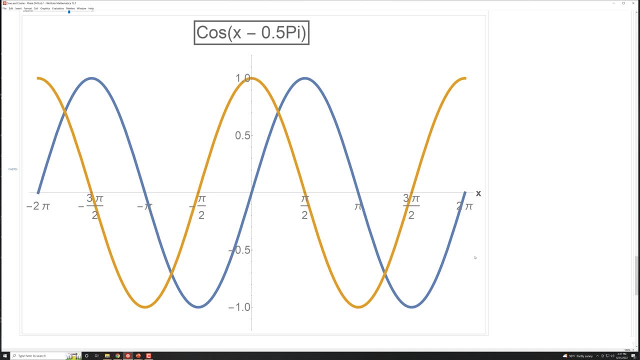 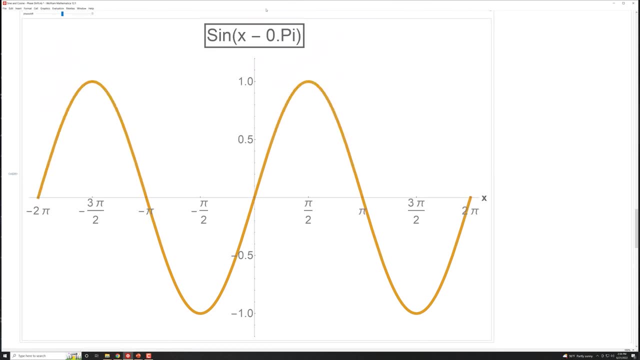 literally shift it and turn it into a sine function. Alright, Now what I'd like to do is go do the same exercise with the sine graph, which is what we have here. Here I have the sine of a function. It starts at zero, goes up, then down to its minimum and then back up into pi period. 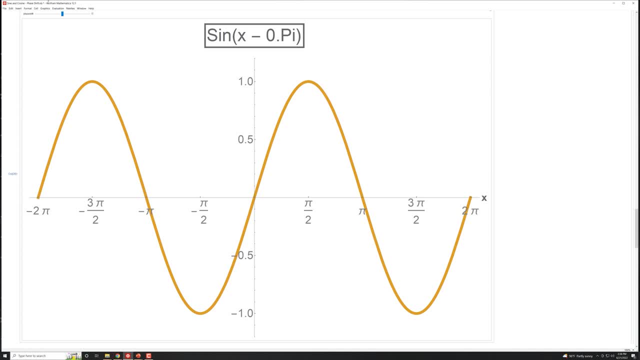 So it's x minus zero times pi, so x minus zero. There's no phase shift happening right now. If I shift this thing to the right by inserting a subtraction in the phase there and if I go all the way to shift, it's going to be the same. So I can't really get any of the 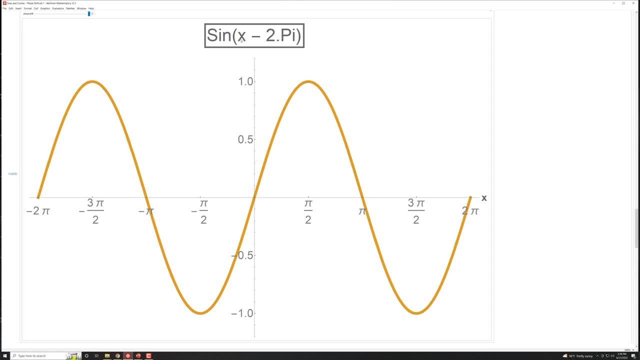 shifting it by two pi, then I've shifted this sign exactly one cycle forward, So I end up lining up with exactly what I started with. If I shift, shift by two pi, then I get a curve that is unchanged. If I go and do the same thing, let me go back to zero here. Here's the zero point. If I 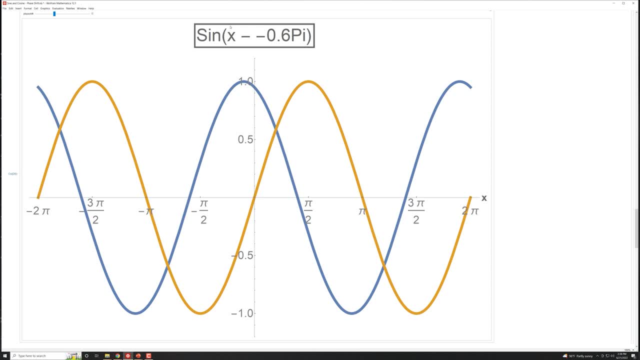 shift to the left, I have it as minus, minus, but this is really X plus a phase shift. Then it shifts the curve to the left, And if I shift the curve to the left again by two times pi, then again the curve I get is exactly the same shape as the curve that I started with. So I shifted to. 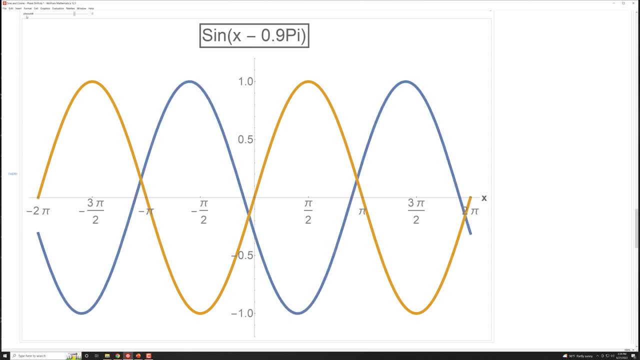 the right by two pi, I get the same thing. I started with a sign. If I shift it to the left by two pi, I get the same thing. a sign, same thing. that's happening with the cosine function. Now let's. 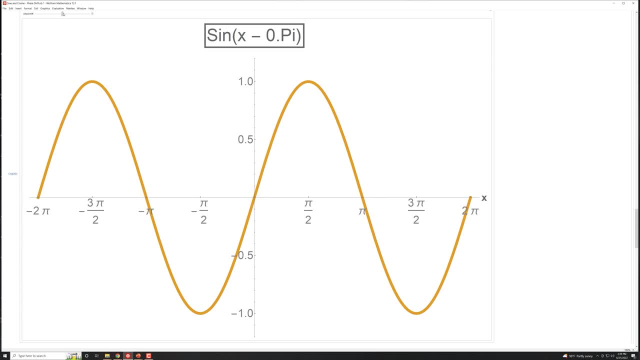 instead of doing that, we start with our regular sine curve. Let's not shift it by two pi, which is one cycle. Let's shift it by half of that. So we're going to shift it by one pi, which is half of a cycle. So if I take a sign and shift it by 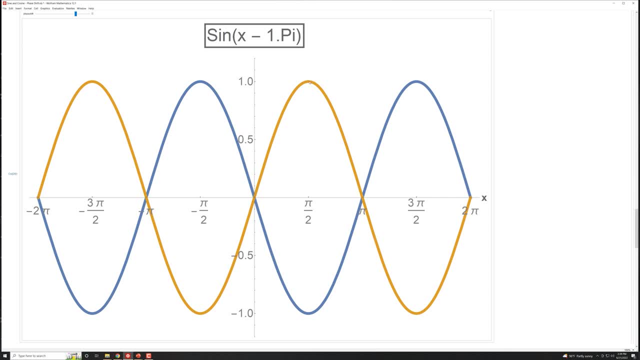 pi to the right. look at what happens. My sign becomes an inverted version of itself When I shift it- pi units- to the right. what happens is this peak goes over here and this goal peak down here goes to this peak right here. And so now, since you shift by pi, it's a mirror image, reflection. 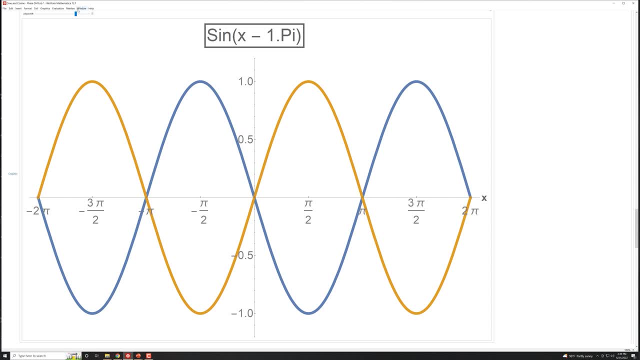 over the X axis. exactly the same thing the cosine was doing a minute ago. And then, finally, if we go back to the zero point where they're lined up, here is my regular sine wave. Now I'm going to shift this guy by pi over two, And what I'm going to get. 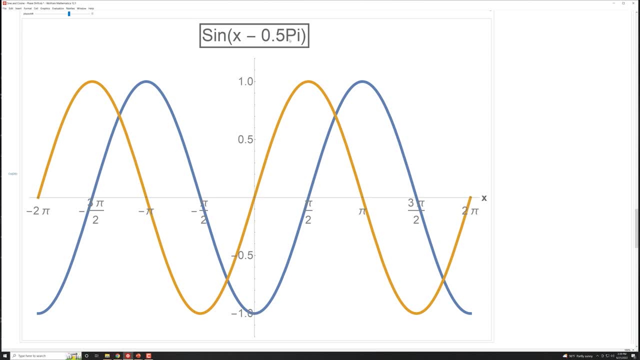 is this? because this is shifting by X minus 0.5 pi, which is pi over two. Then the blue curve is: what is the blue curve now? So we start with a sine and we shift it. It turns into a cosine. 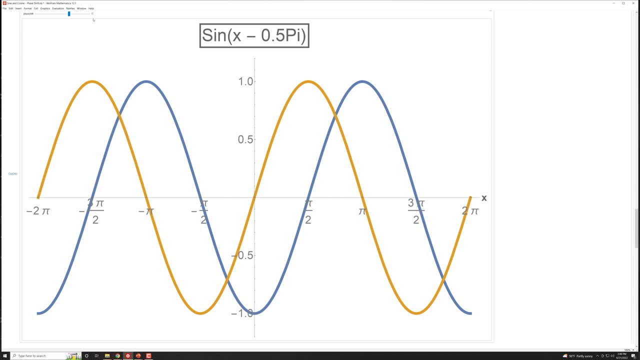 but sort of an inverted cosine down here, because it starts on the bottom end. If we actually go the other direction like this, if we shift it the other direction, so it becomes X plus 0.5 or pi over two, then your sine curve becomes a cosine. 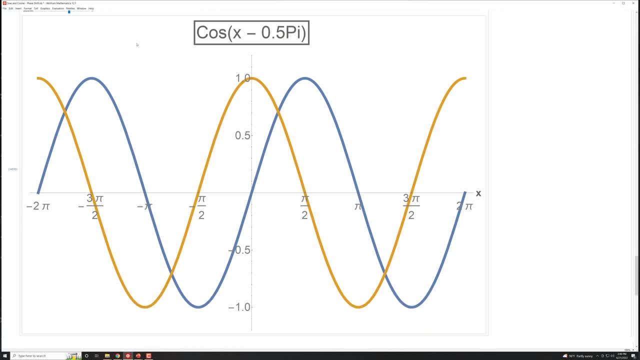 So the bottom line is that I really want you to know is that if I take a cosine function like this and I shift it to the right by pi over two, then I can turn it into a sine function, which is the new, the blue curve. 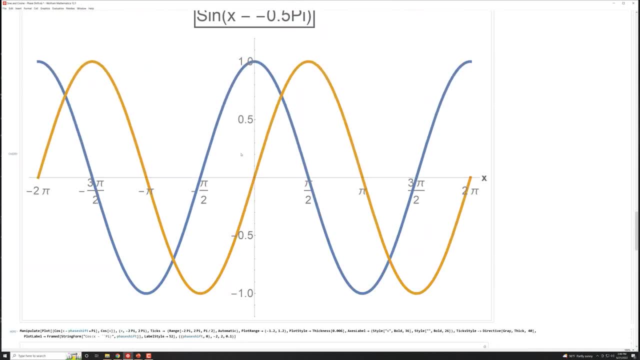 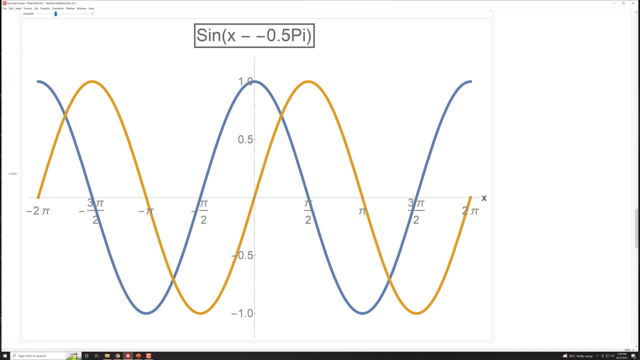 turns into a sine function right. And then if I start out with a sine function and if I shift it to the left- to put this peak right here on the axis, the left by how much? by pi over two- then it turns into a cosine. So the punchline is you can turn any sine curve and write it in terms of a. 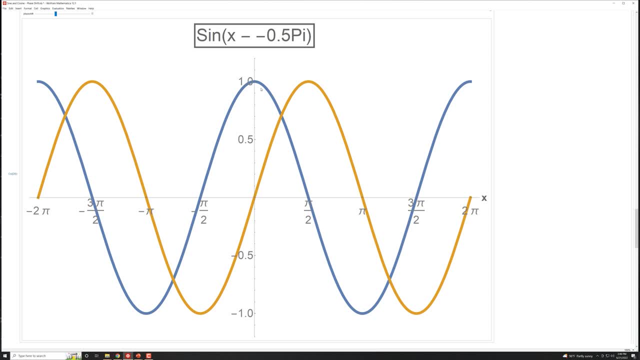 sine, but you have to put a phase shift in order to make it slide and turn it into a cosine. And you can take any cosine and you can write it in terms of a sine if you do an appropriate phase shift right Now. the last thing I'll look at, let me slide here. I wrote a note to myself. 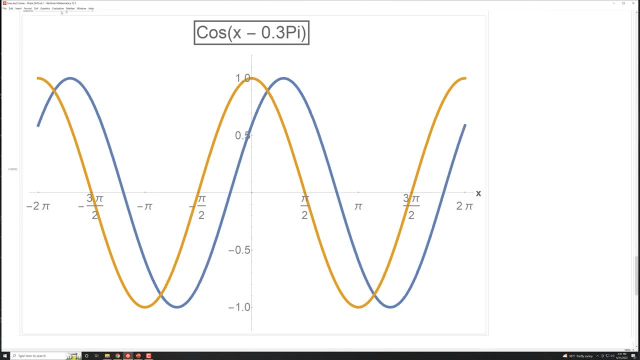 Look at what happens before you read that. Look at what happens to this cosine here. If we start here, if we want to envision, what do we use these sinusoids for? We use them for a lot of things, but one thing we learn is we can write down what a wave looks like when it's traveling through space. 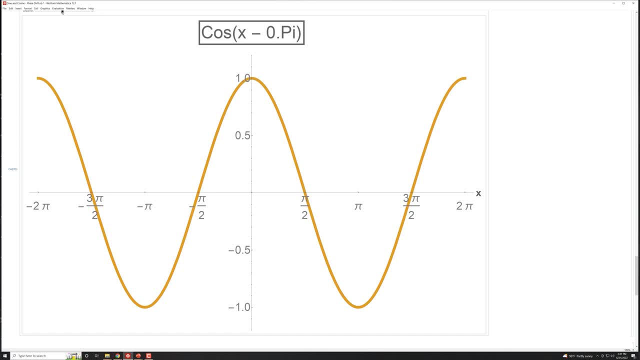 like a light wave, or an electromagnetic wave is another word for it. So if I increase the phase a little bit, then the wave is displaced to the right. But if I keep displacing it in time, so that this number over here, the 0.7 pi. 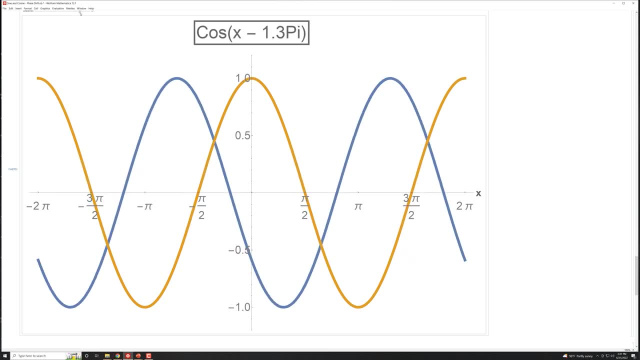 it keeps getting bigger and bigger and bigger in time. then what happens is the wave is propagating to the right. The crest of this wave is constantly moving and carrying energy in the direction of motion. So when a wave hits you, it's carrying energy. 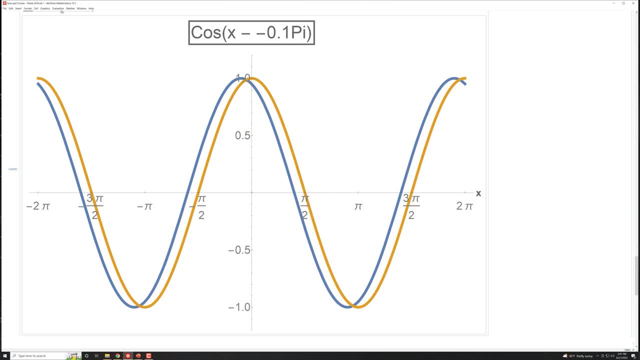 because the crest and the trough are slamming into you. The whole wave is slamming into you, but that's one way to visualize. it is the crest and the trough is moving in time. But in order to get this illusion of the wave moving, 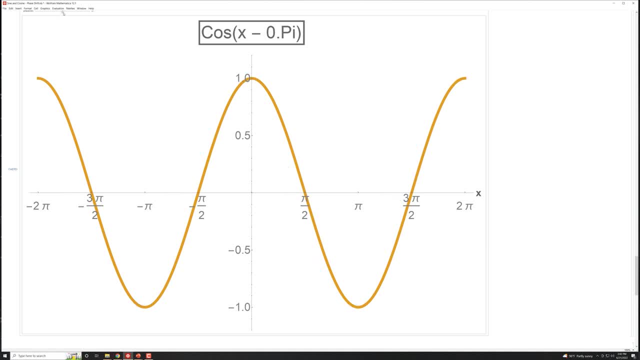 I have to kind of constantly shift the phase. So in other words, here the phase shift is zero, Here the phase shift is 0.1 pi, then 0.2 pi, and 0.3 pi, 0.4 pi, 0.5, 0.6, 0.7.. 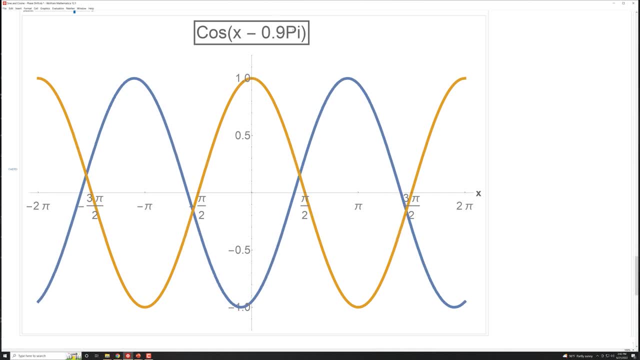 I have to constantly increase it So as time goes up. if I replace this number with something that goes up with time, then if I put a new number, a new variable time in there and keep increasing it with time, then the wave will be always propagating to the right. 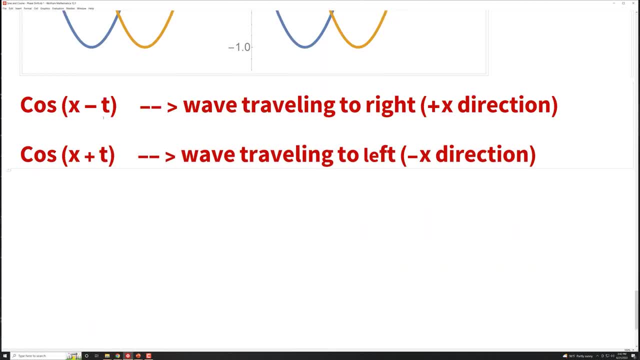 as time goes on. So that's what this note is down here. If I write down cosine of X minus T, where T is time in seconds, then this will represent a wave traveling to the right because the phase shift. notice it's X minus T. 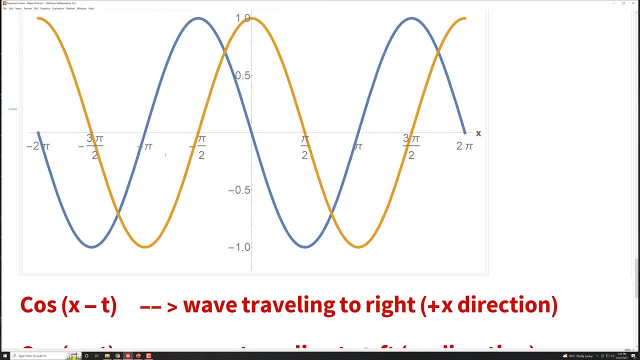 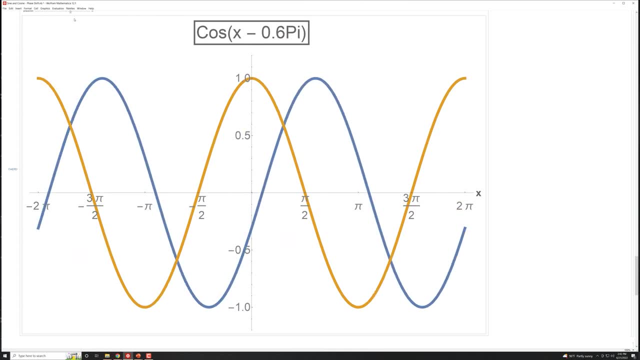 the phase shift is time in seconds and will constantly be going up, And that it will manifest itself when you're graphing the thing. it'll manifest itself as a wave propagating to the right If you make the phase shift always go up with time. 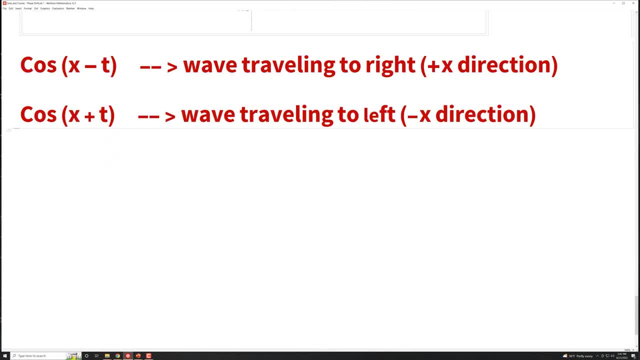 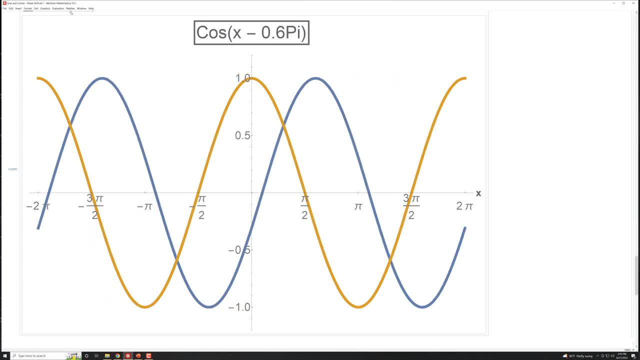 So if you just stick time in here, then as time goes on, the phase shift gets bigger and bigger and bigger and the minus sign means it goes to the right. So in that case, when the time is going up all the time, the phase shift is going up all the time. 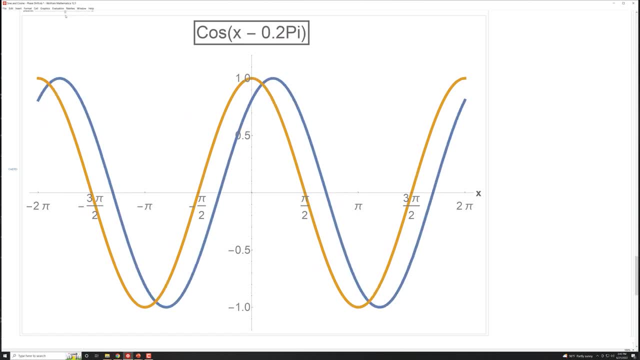 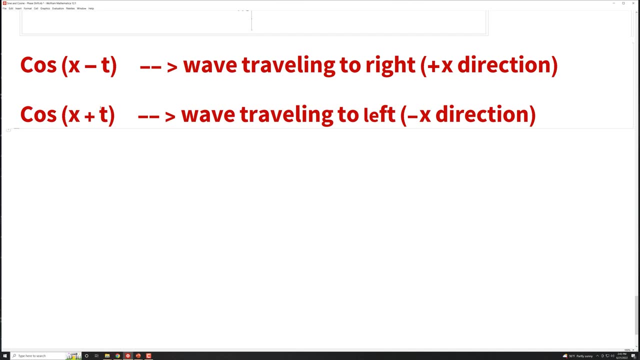 the wave is propagating to the right. Okay, let me reset my starting point. The second note under there is saying: if you write the wave as cosine of X plus the time in seconds, then what you're doing is the plus means it's shifted to the left. 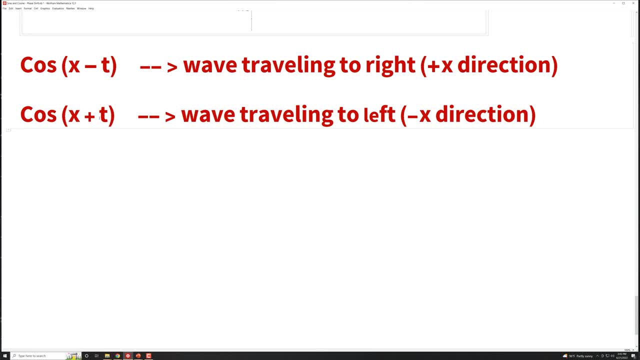 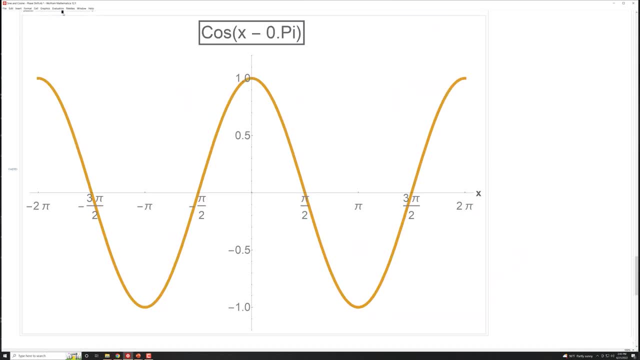 And since T is in seconds, as time ticks on, the phase shift is going up and up, and up and up. but because it's a plus sign, the wave will be traveling to the left, And that is illustrated by what I'm saying here. 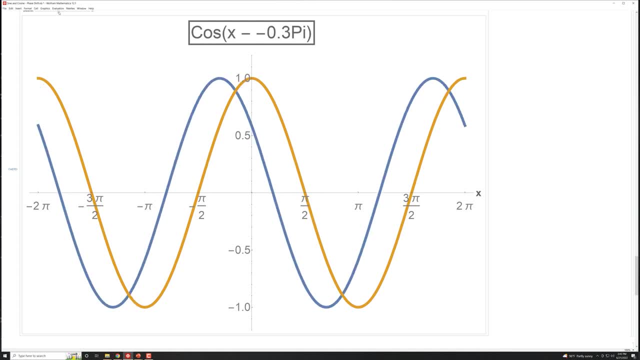 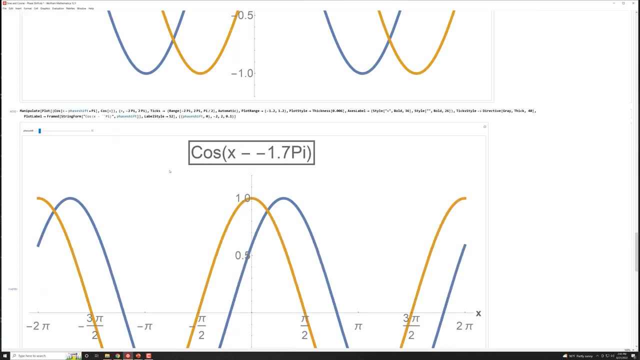 that here is a no shift at all. but as I start shifting and adding a phase shift constantly with time, every second that goes by, increase the phase shift. then the wave will propagate to the left. So that is a wrap up of what we have here. 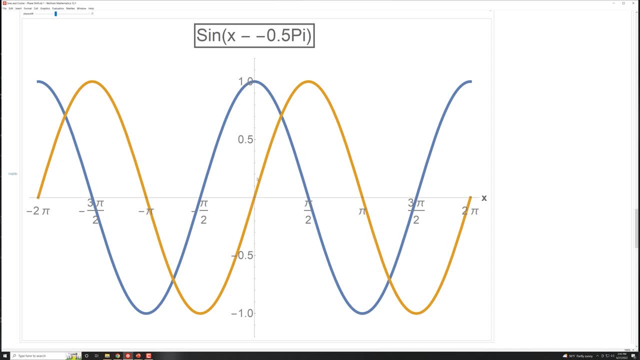 We can turn signs in the cosines with phase shift. We can turn cosines in the signs with phase shift. We can invert a cosine or a sign by shifting by a period, by a half of a period, in this case pi. 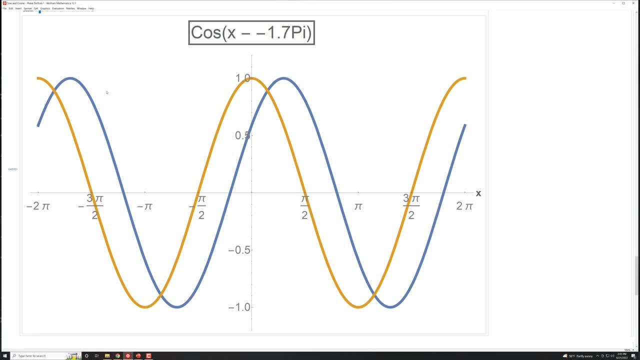 And we can also create the equation for a traveling wave moving in the plus X or the minus X direction by allowing this phase shift to always increase or decrease in time, And that is how we write. This is the way we write When you take physics or engineering. 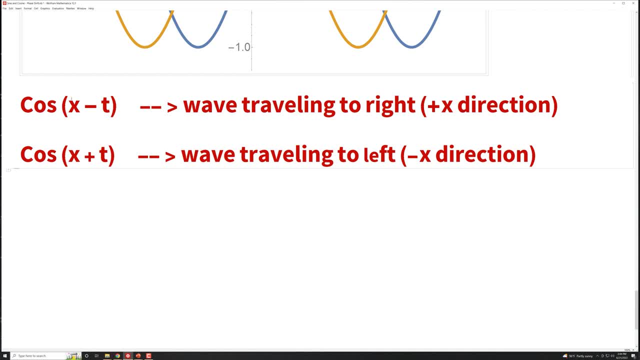 you will write down a traveling wave as a variation of this equation X minus T. inside of the cosine You could also write the wave in terms of a sign. You could write it a sign X minus T also, and it'll be the very similar shape. 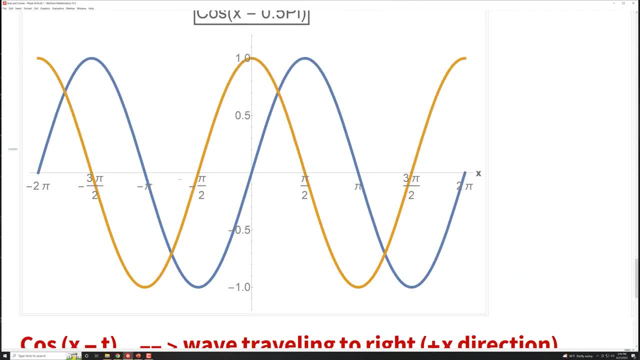 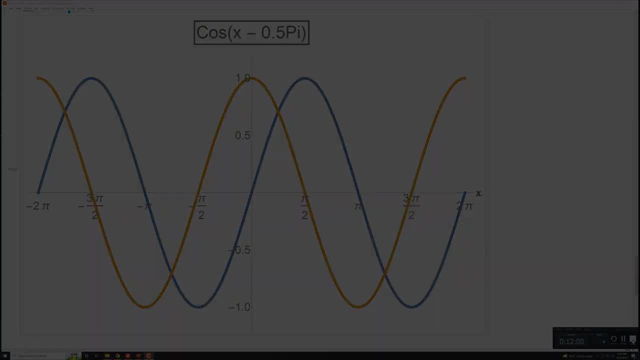 but it will be shifted a little bit relative to this. So now let's go back to the board and continue solving our problems and learning how to sketch these guys. All right, welcome back. I hope you enjoyed the computer demo. I think personally that. 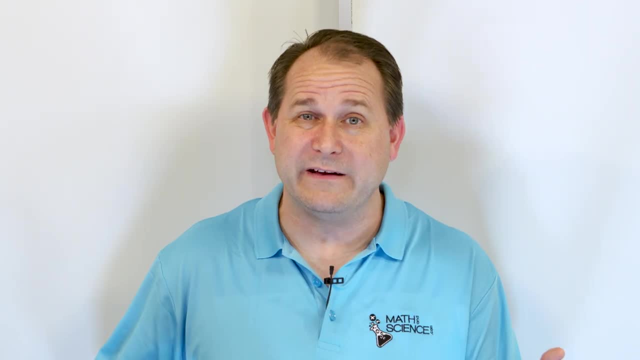 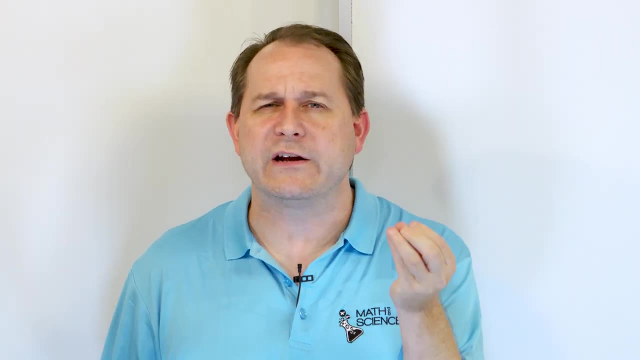 uh, you know, a picture is worth a thousand words and a movie is worth a million trillion words. So when I was animating and showing you what was happening with the graphs, I really hope that that brings it home how you can take. 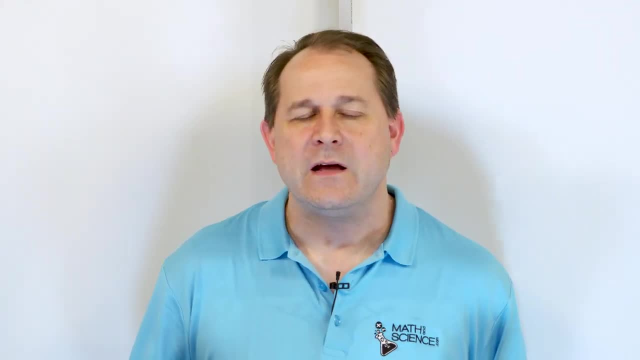 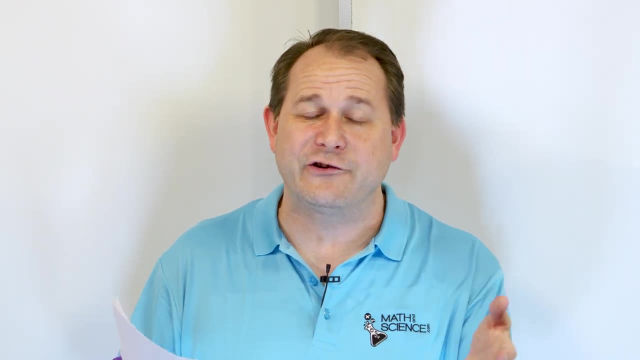 a cosine or a sign and write down and traveling wave. Now, of course, when we get into physics and engineering, you know the equations are a little bit more complex than what I wrote there, but the bones of it is actually what I just wrote there. 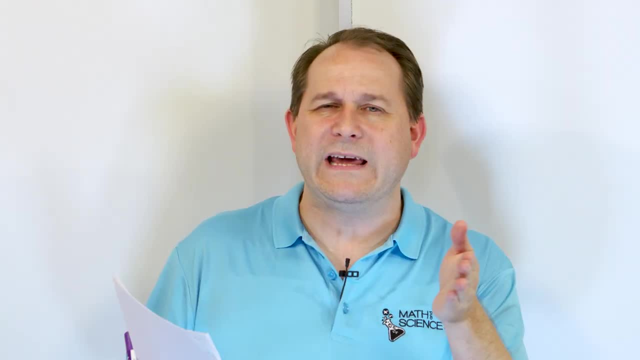 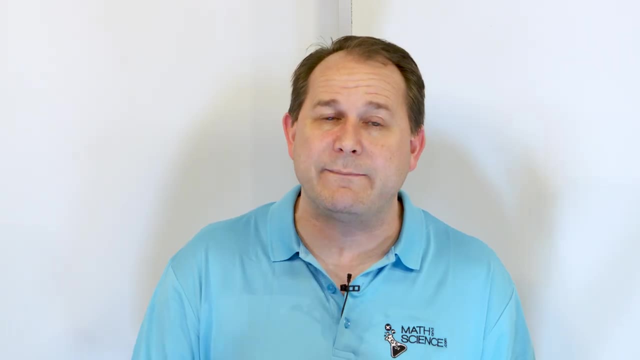 So you now know the fundamental. you know, when you open up a book in electromagnetic wave, like an antenna book, an antenna theory book or a microwave transmission book, the equations that we use to describe them. they look a little different. 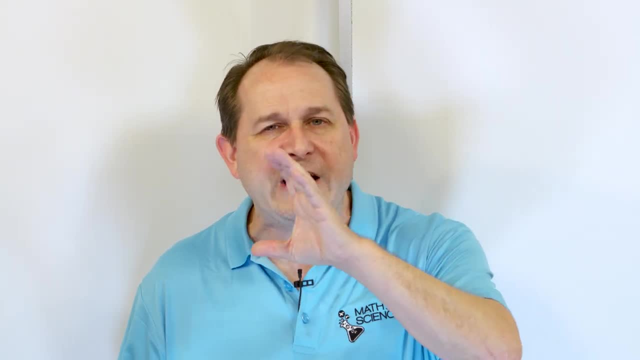 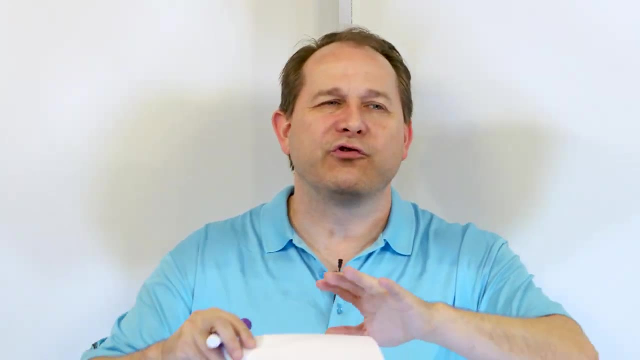 but the bones of them are basically what I showed you in the computer. When you change the phase and allow the face to always increase, uh, increase- with time, then you write down a traveling wave. Now, before we get into drawing pictures of face shifts and all that, 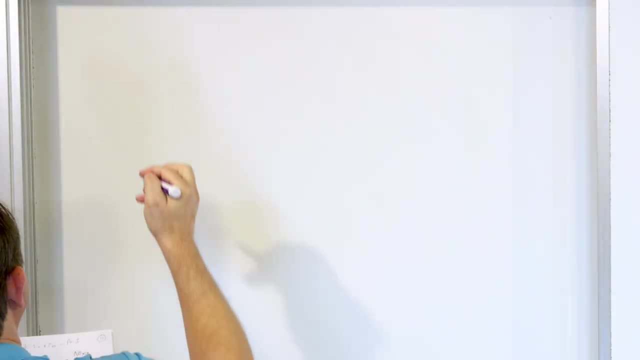 let's start kind of at the beginning. let's take a look and graph the following function- And we already did it over there in the computer. but let's talk about it a little bit more: F of X is negative sign of X. 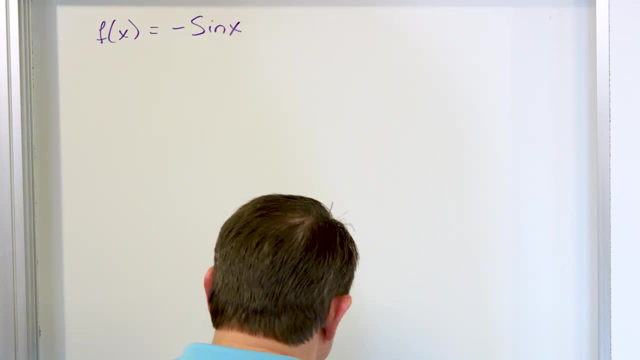 What does that look like? All right, What do you need to think about? This is you need to think about the base function and how what I've written on the board changes the base function, right? So, for instance, if I wanted to sketch this guy, 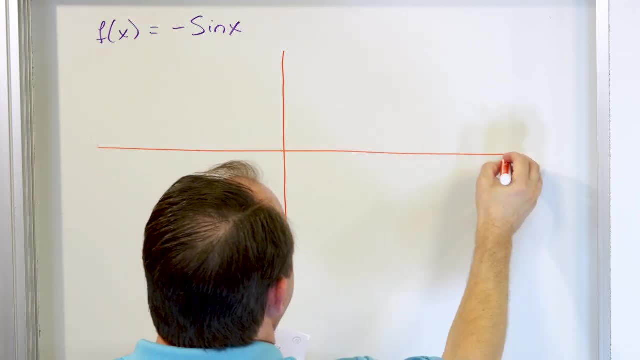 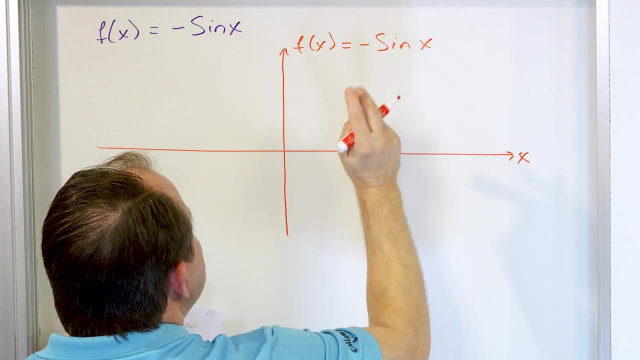 then what I would do is I would just draw some coordinate axes right here and I would say X, and I would say I'm going to graph F of X, which is equal to negative sign of X. Now the base function is just the same thing without the negative sign. 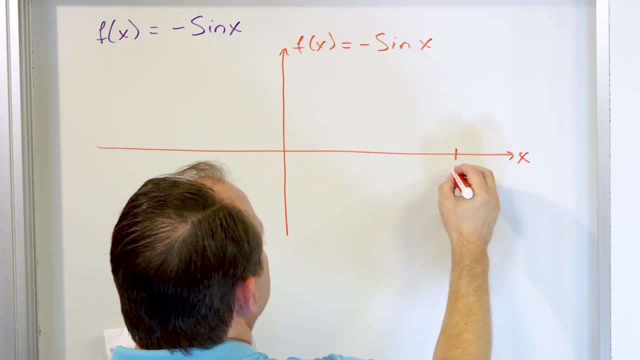 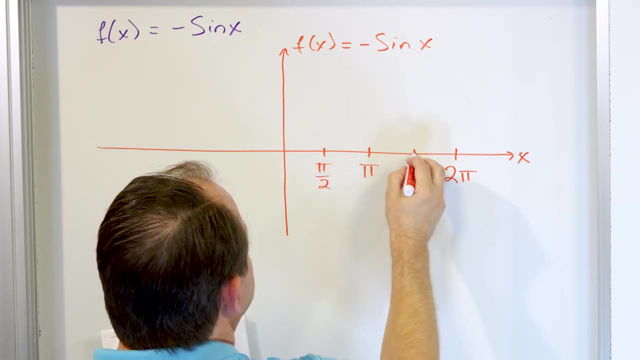 So sign of X. I already know what the period is. The period goes to two PI, and so that means half of the periods right here at PI, And so half of this is PI over two, and so this is PI over two to PI over two, and then this will be three PI over two. 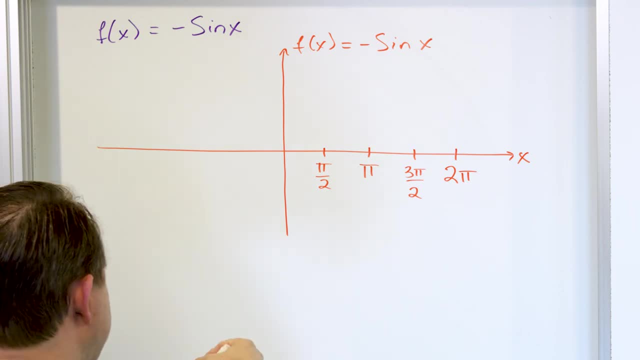 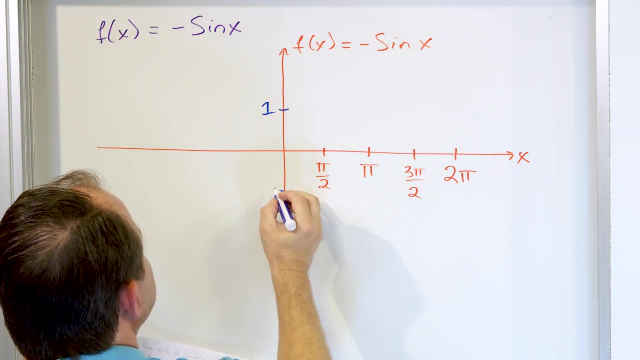 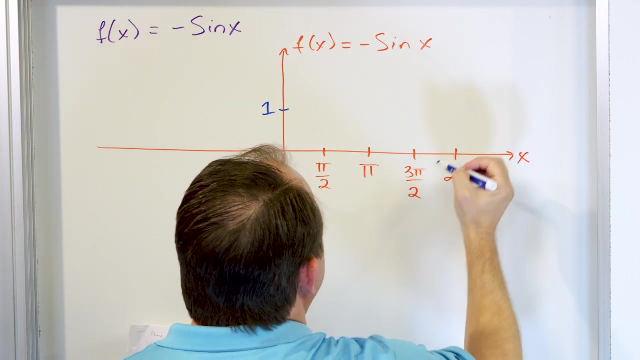 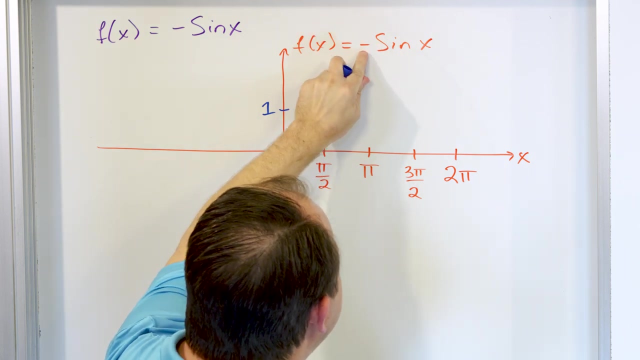 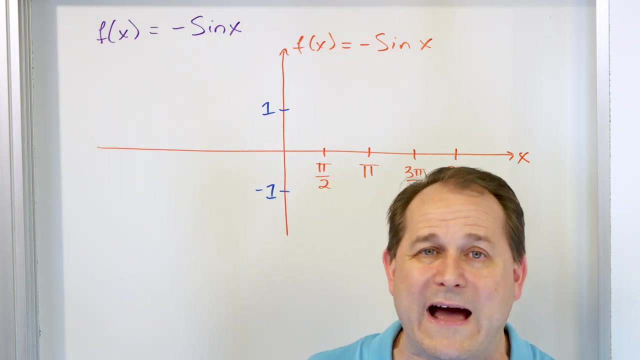 And so you can set your axis up, as if I'm going to draw This guy right and since, for again, forgetting about the negative one. since it's a regular sign function, we know that it's going to go up to a maximum of one and down to a minimum of negative one. and if it were a regular sign function, it would just start here, would go up, would come down and it would go up like this one cycle in a two PI region. so that's what would happen if I didn't have this negative sign here. when I have this negative sign here, when I have this negative sign here, how does it change if I was going to create a table of values to graph this? 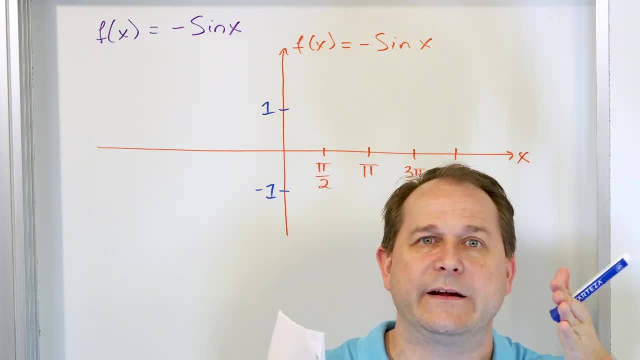 thing. then what I would do is I would calculate a negative sign of X. so what you're going to do is you're going to take the sign of the angle, you're going to get the answer to that and then you're going to stick a negative sign on the, on the, on the number. so if sign gives you back one half, then what you really plot on here is negative one half. if the sign gives you, you know, a point 852, then you actually put a negative sign. so it's negative point eight, five, two. likewise, if you get a negative answer, if the sign returns, you know, negative, point four, six, then we do the same thing. 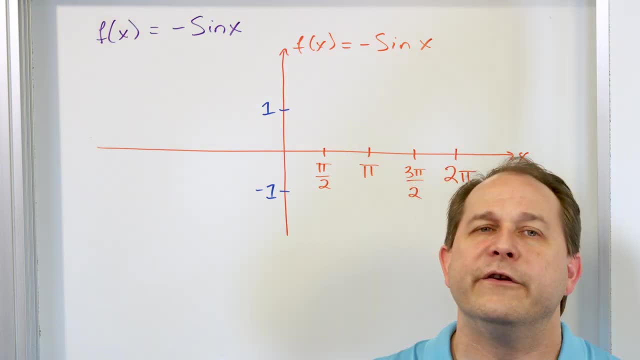 you put a negative on front, it changes it to a positive, 0.46.. So for every number you get back in your original sine curve. really, what you're plotting is the negative version of that. That's why it's a mirror image, reflection over the x-axis, as I showed you in the video there. So again, a. 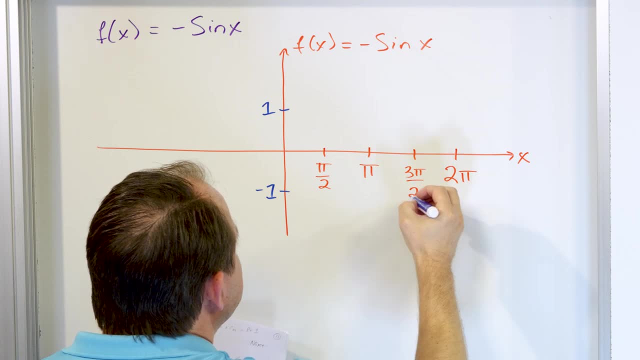 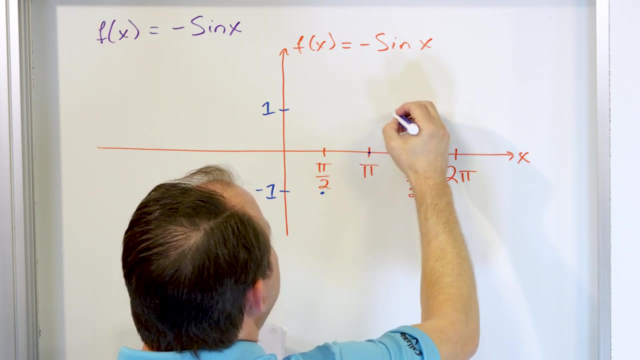 normal sine function would go up to a maximum and then down to a minimum. but because this has a negative sign, really, this one is going to start here and it's going to go to a minimum here and then up through here, and a maximum is going to be right over here and then back to zero, right here. 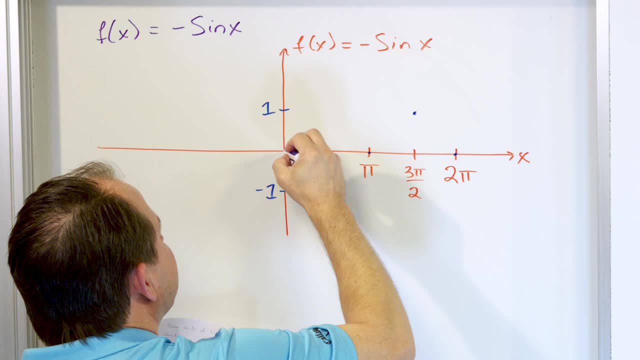 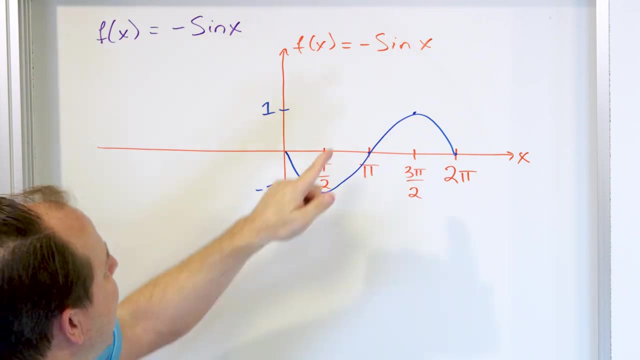 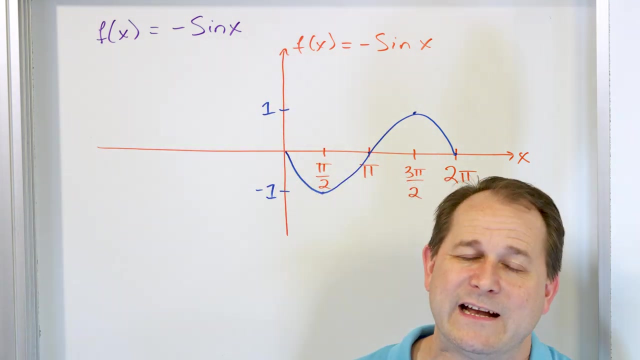 So whereas a normal sine would go up, down up, this one is going to go down and then up and then down again. So when you have a sine or a cosine with a negative sign on front, what it does is it flips the thing upside down. but instead of memorizing- I don't want you to memorize it- it flips it upside. 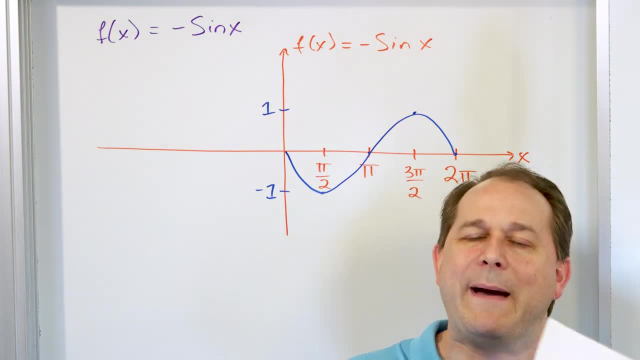 down. I want you to think about why. because any number you get back from the sine function is just going to be a negative sine function. So if you have a negative sine function and you have a negative sine function, it's going to be negated. So if it gives me normally a value up here, I'm going 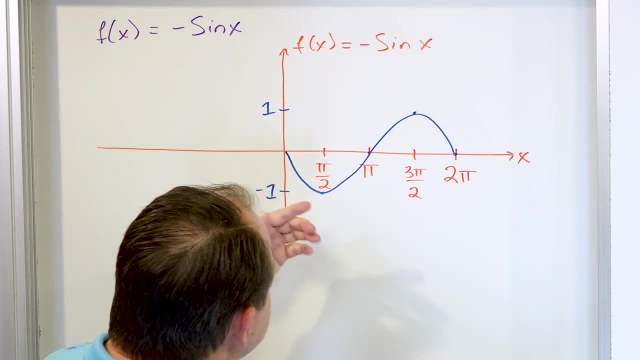 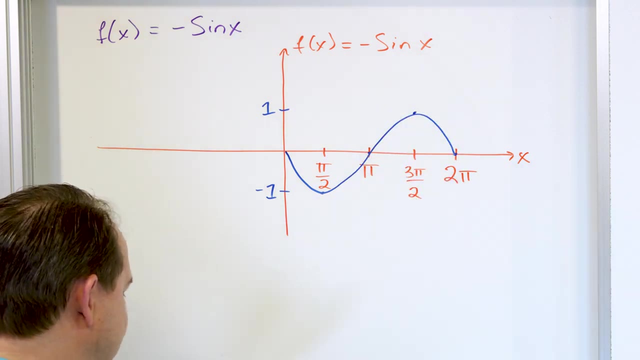 to immediately negate it, so it becomes down here. If it usually gives me a number down here which is negative, it's going to put it up here, and so that's why it's plotted upside down like this. Okay, so putting a negative sign onto a sinusoid, simply mirror image reflects it over the axis. 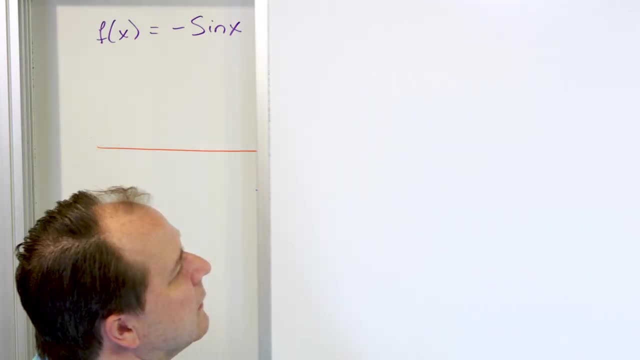 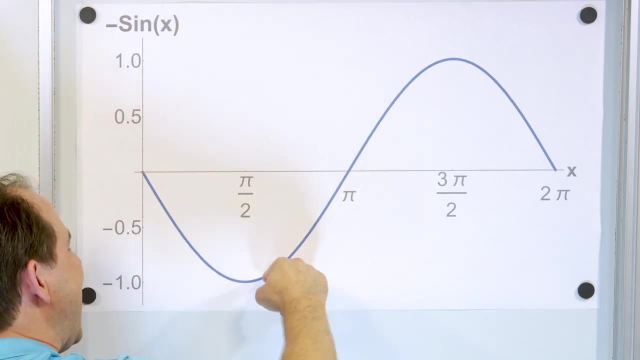 like this. Now let's just double check that. So we plotted this function, a prettier version of it, so you can see, negative sine of x is going to be negative sine of x. So if I put a negative sine, of x does exactly what we drew on the board. it goes down to a minimum of negative one, and then 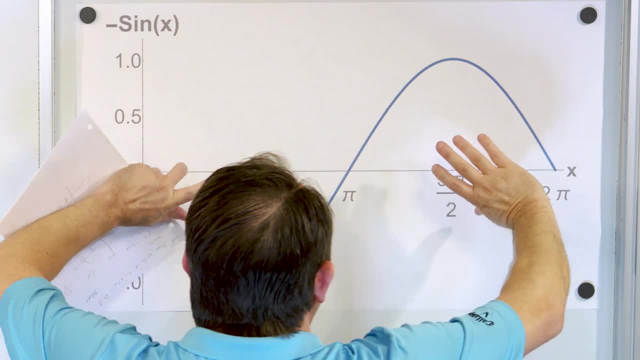 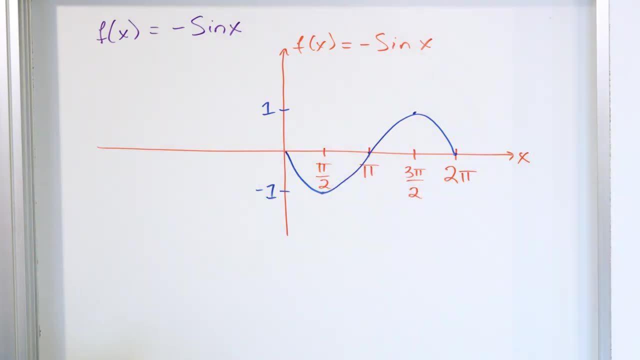 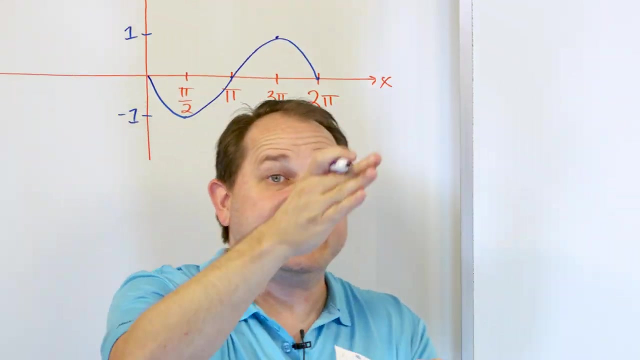 the maximum goes over there, over a two pi region. So it's literally as if I just rotated this thing and flipped it about the x-axis. Now we just did a lesson on phase shifts. Okay, we are kind of combining multiple things here. We already know that sines and cosines have the same shape, and we 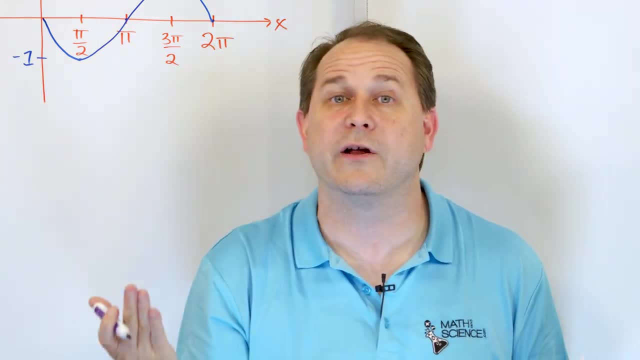 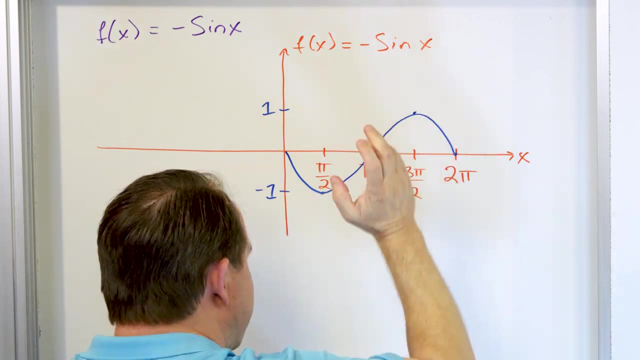 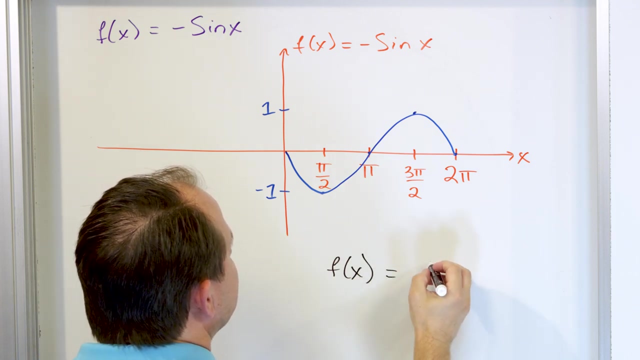 know now that we can slide them back and forth by what we execute what we call a phase shift. So, even though what we have plotted here is the function negative sine of x, just for giggles you could write this thing differently. You could say: f of x is going to be equal to sine of something, sine of x with some. 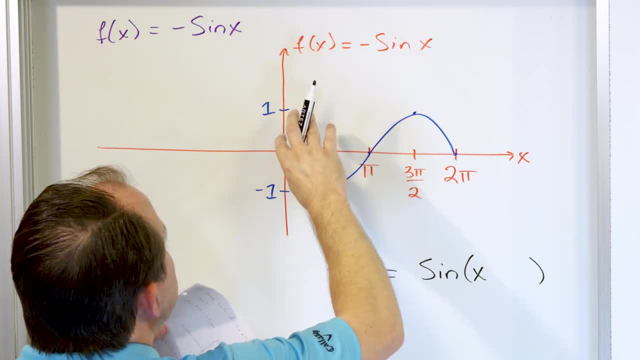 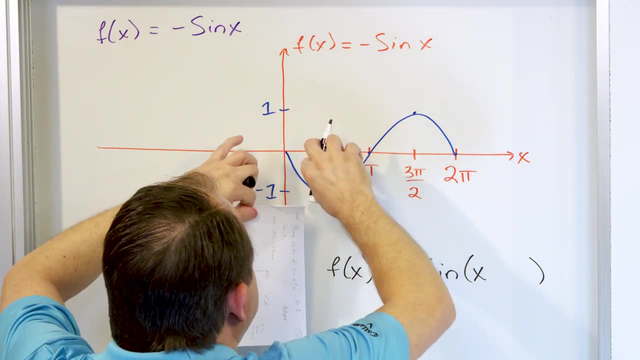 phase shift. So where is the normal sine function? The normal sine function is right here, All right. so if you need to visualize this with me a little bit, here, the normal sine function goes up, down, up If I shift it and then of course it's going to go down this way, right? 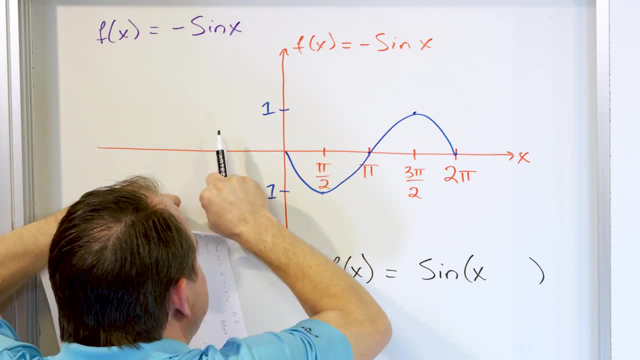 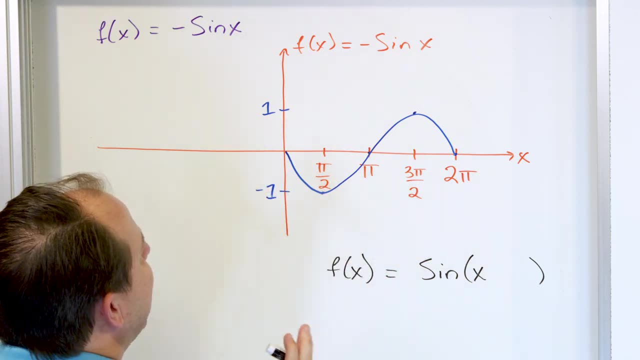 So it's going to go like this and then up like this. If I were to grab it and slide it to the right, then the trough that would have been here will then be here. How far do I have to shift it? We just saw it there. Since a full cycle is called two pi, by shifting by a half cycle, which is in. 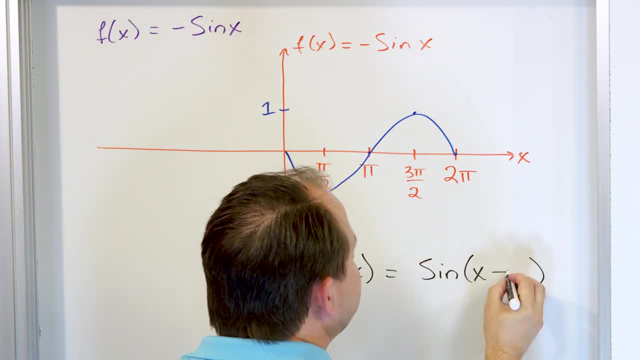 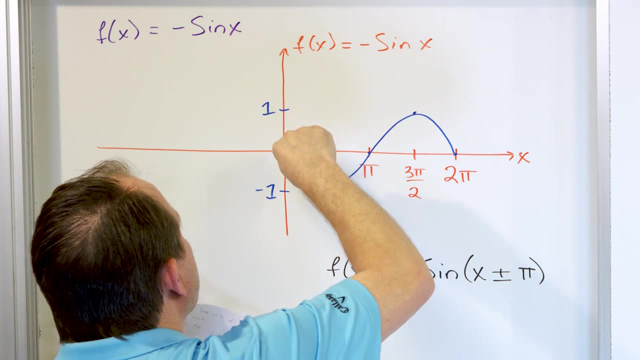 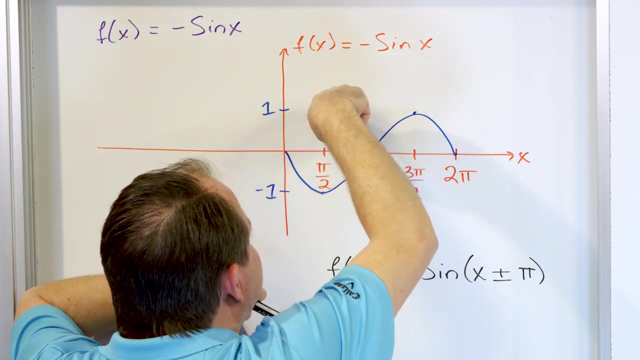 this case pi is what's going to do it. So you could basically shift it by plus or minus pi to basically reproduce this graph here. So if you take a normal sine, which is this a crest right here, shift it to the right by how many units, then this point would go here, The crest would become: 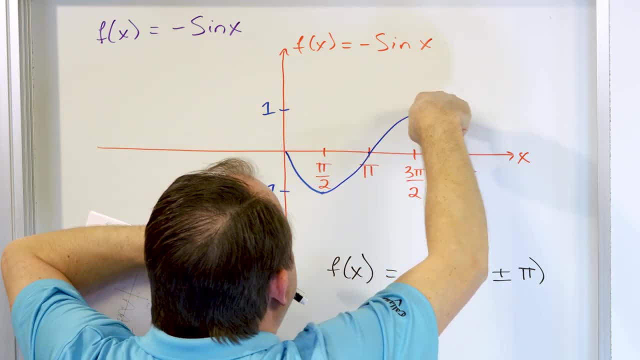 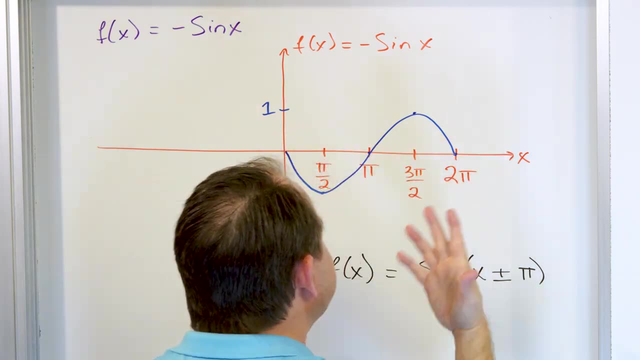 here and notice the crest was here and the crest was here. This is a shift of pi. This would become here After it goes down here. this one would become over here. This is a shift of pi in the positive direction, But since everything is symmetrical, you could shift it in the negative x direction. So 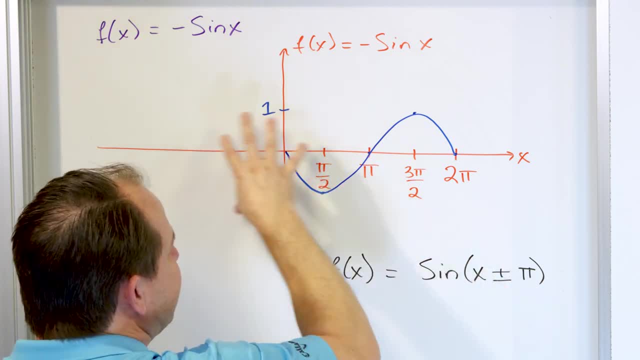 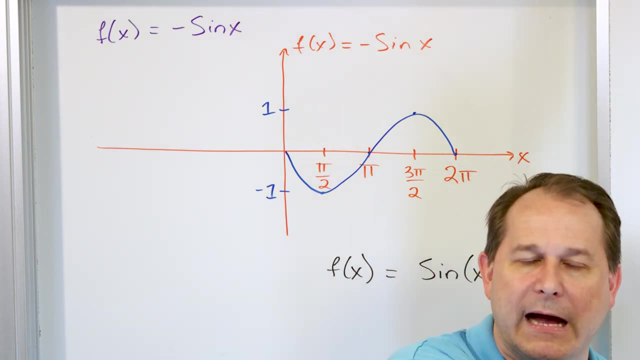 the plus sign shifts it to the left, The negative sign shifts it to the right, But it doesn't matter if you you could write it as a phase shift of sine of x plus pi. So you could write it as a phase shift of sine of x minus pi, because the thing is symmetric, no matter which way I move, if I move pi. 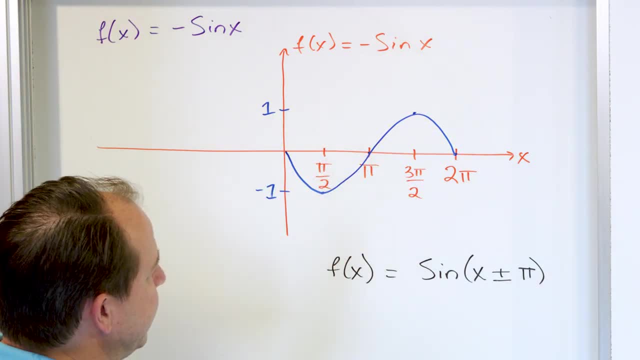 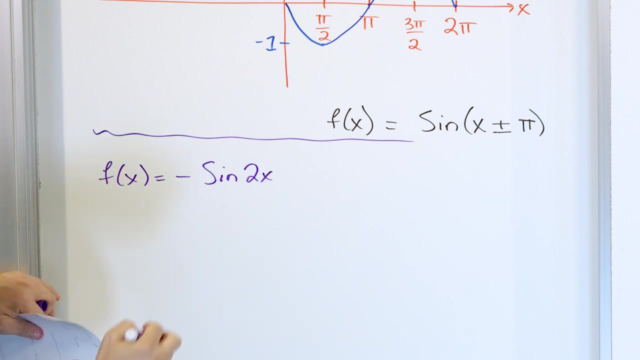 units. that's half a cycle. it's going to line up with this right here. All right, Now let's move along to problem number two. Right, Let's plot: the function f of x is equal to negative sine of two x. Now, what's going on here? And of course, the two x's is wrapped in parentheses and the 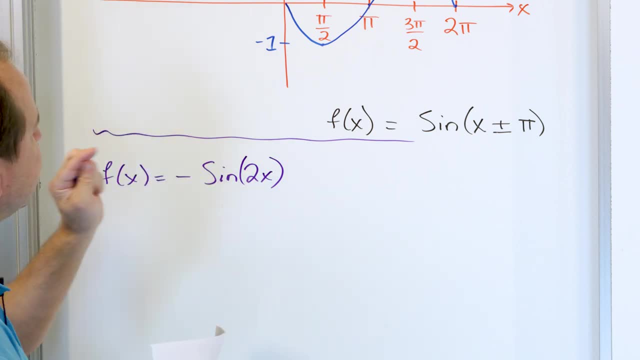 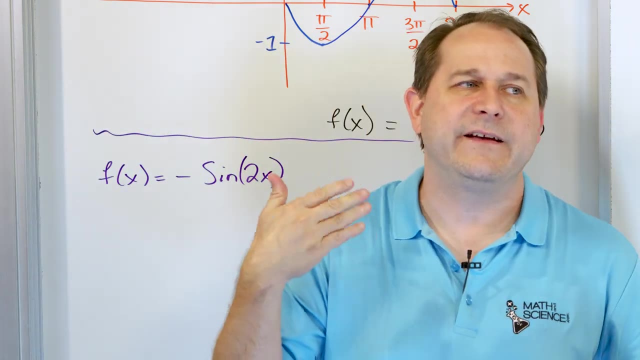 sine is what's acting on this. This is exactly the same function as before. The only difference is that we now increase the frequency. Remember the number in front of the variable inside of the sinusoid. that is what we're going to. what we talked, talked about in the past, called the frequency. 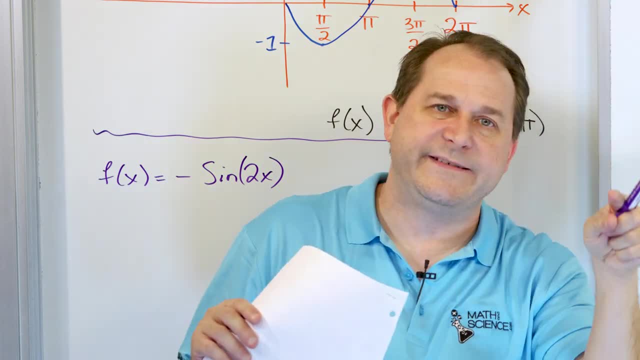 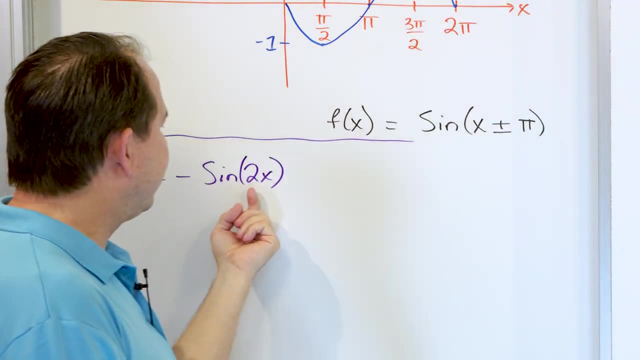 And what it means is, instead of a regular sign making a cycle over two pi radians, we must now have two complete cycles in the same window. So this is like your speed multiplier: It wiggles it faster, which means higher frequency. Now we have to have two complete cycles of this function. 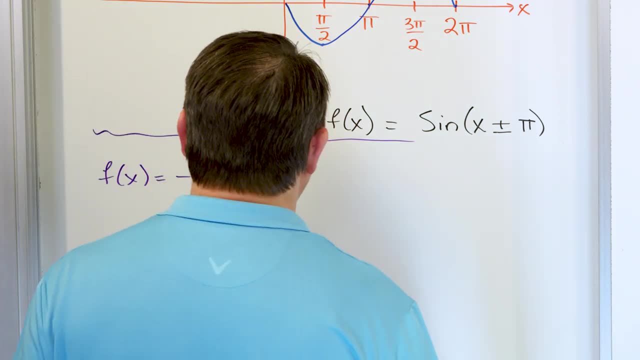 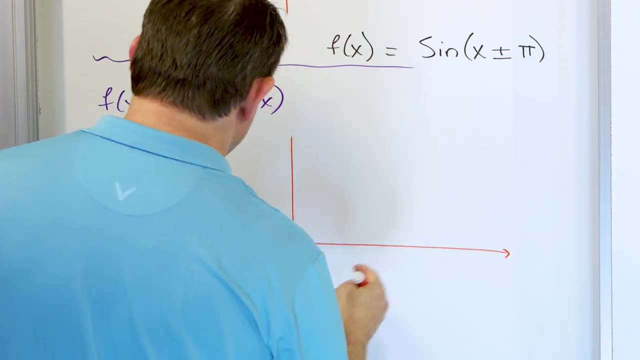 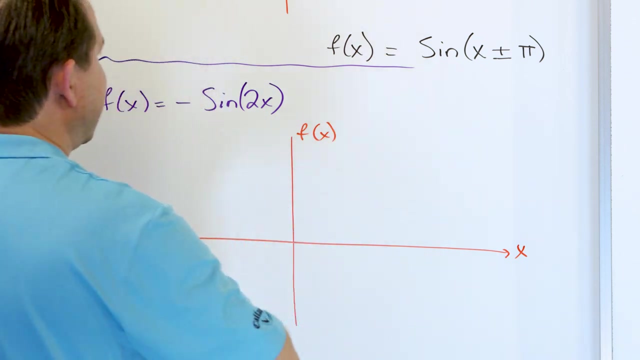 inside of a normal two pi period For that guy there. So let's go and draw and see what this looks like. Like this, All right. So what we're going to say is: here we have x and here we have f of x. All right, Now let's think. 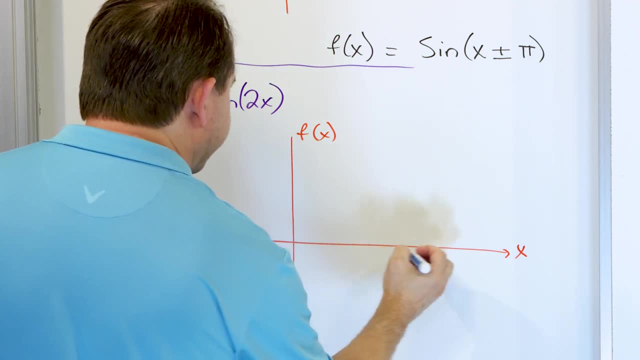 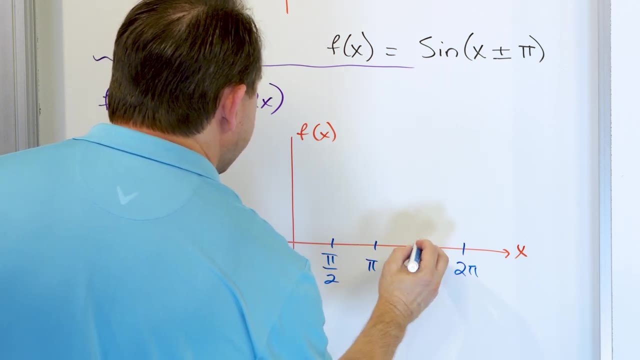 about this for a second before we get to trigger happy Let's go and draw our thing. So let's put two pi. We know that's going to be important. This is going to be pi, and this right here is going to be pi over two, and this is going to be three pi over two. Now this one has a. 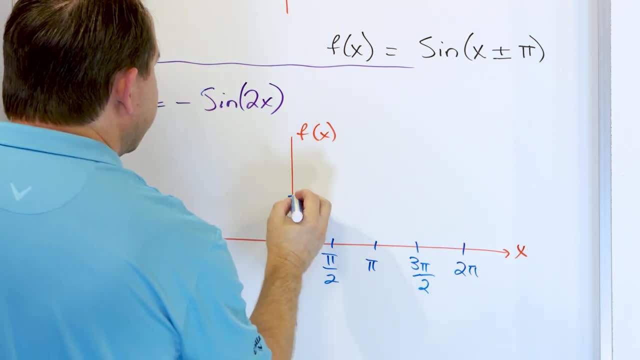 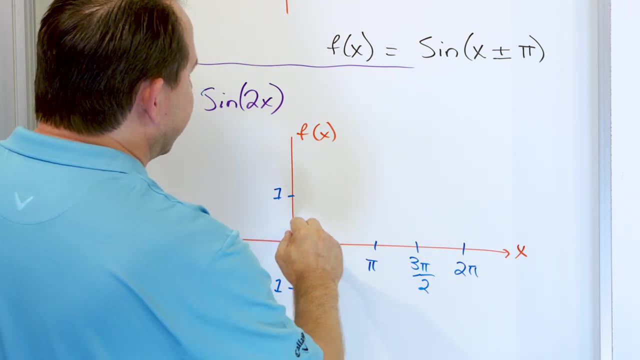 there's no coefficient change out there, So we know it's going to go up to either plus one or minus one. Now a normal sign goes up and then down and then it goes like up and then down and then up where one period is in a two pi window. But since there's a two there, we know there has. 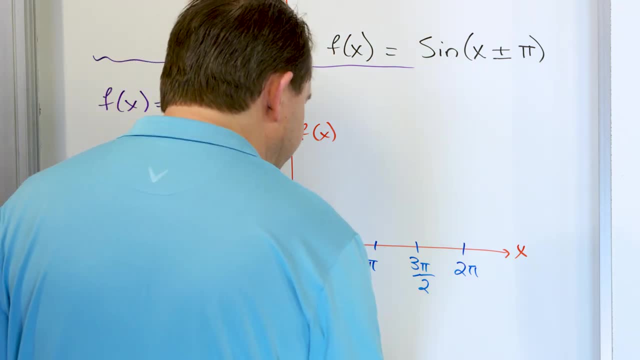 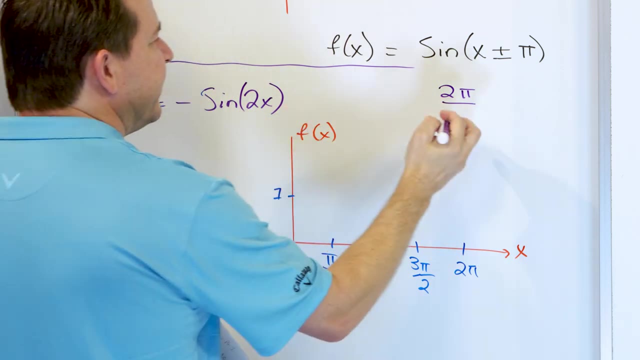 to be two cycles in a two pi window. Two cycles in a two pi window, And if you're not sure about that, what you could do is you could just take this number. We could say two pi over the number that's here- This is how we did it before- is equal to the period of time. So we're going to. 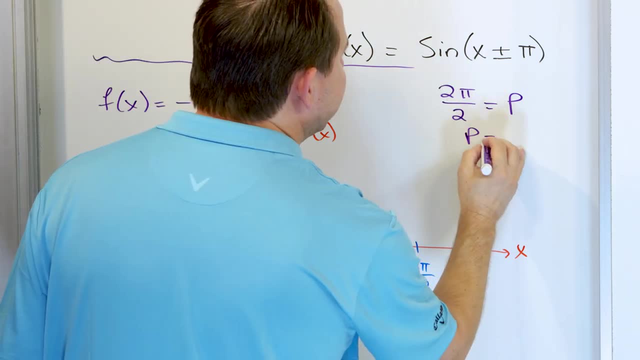 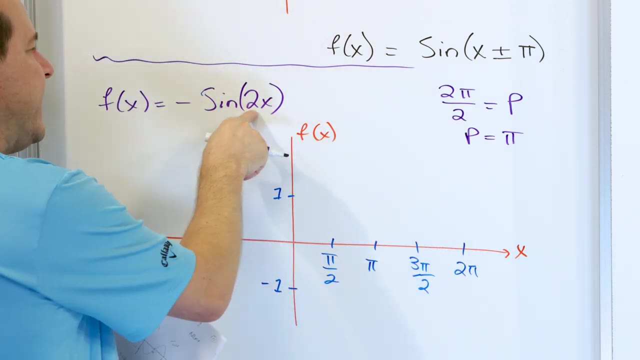 take the period p, Right, And so then we cancel this out and the period p is equal to pi. So now the period has to be pi to get one cycle here and then another cycle right there. So knowing that this means we have to have two cycles in a two pi window, or actually calculating the period is 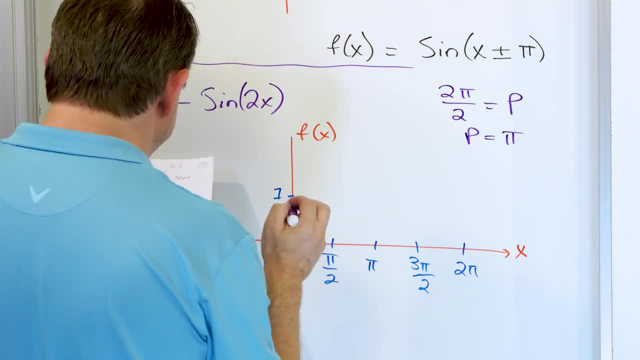 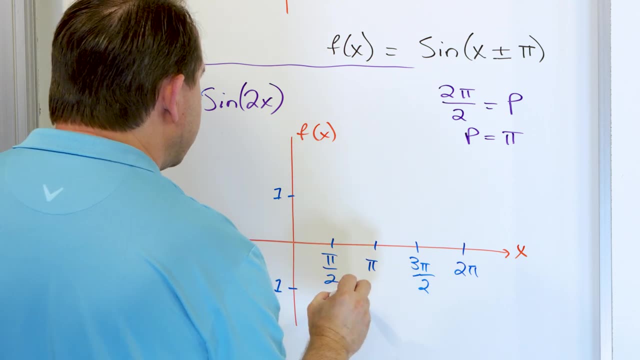 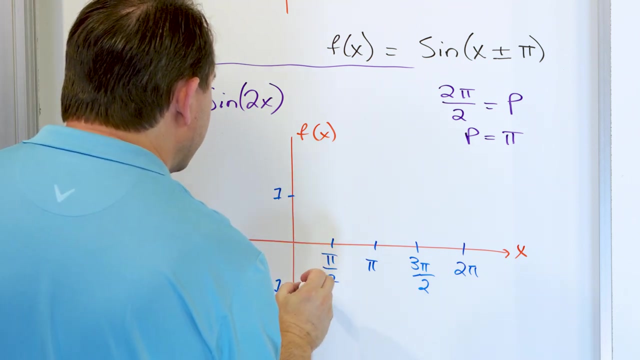 fine either way. So to actually to actually make progress with this, what we know is that normally it would have to go up and then down and then up, But that's a normal sign. Here we have a negative sign which flips it over. So what it means is it has to go with a minimum there. 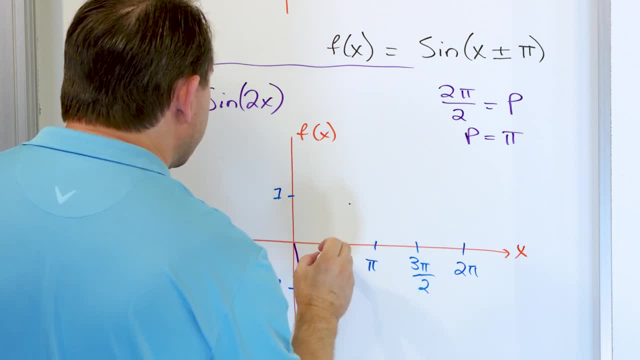 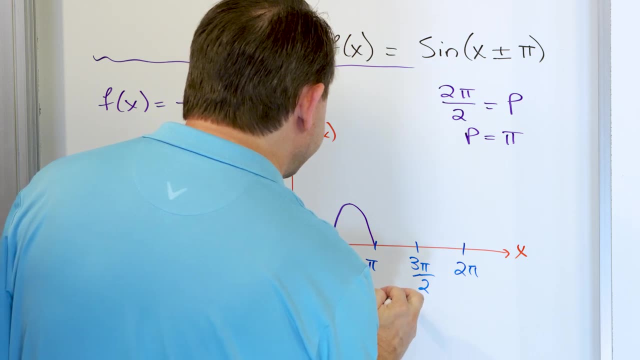 and a maximum there, It's going to have to go down, hit this one, then go up, then get this one and down, like this: Now we have one cycle in a one pi period And then the same thing: here It's going to be down, here It's going to be up here. So it's going to go down, then up and then down, like 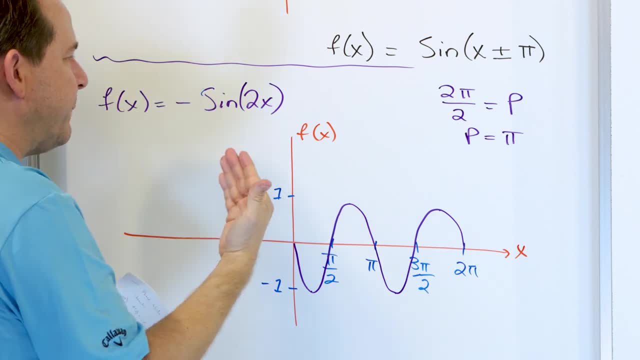 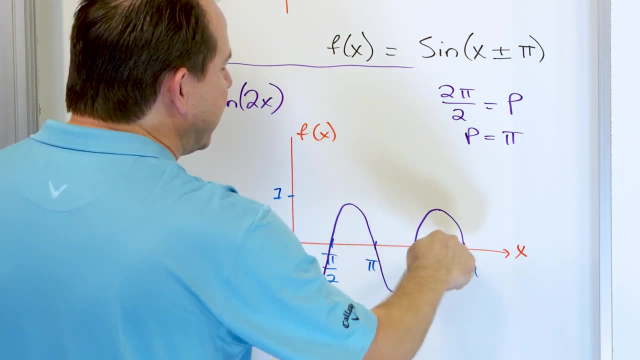 this. So here we have again. it's a multi-step process. The first thing you do is say: what does the two mean? We calculate the period. If it was a normal sign, it would go up, down, up and then up, down up, Two cycles in a two pi period. But 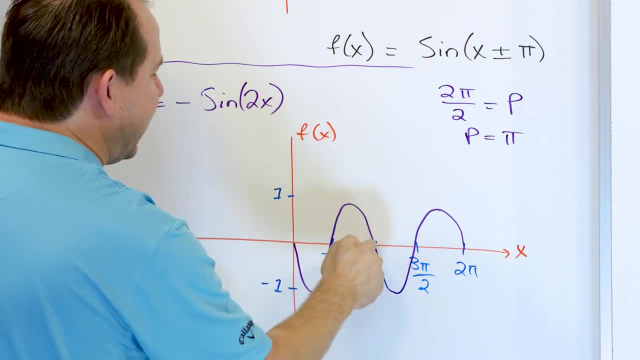 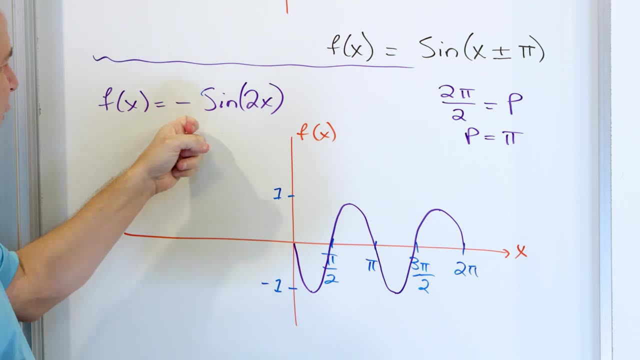 since we have a minus sign, it gets flipped upside down. So down up down, that's one cycle. Down up down, that's another cycle. Now, just to shed some more light on it, let's graph this thing and see if it does in fact look like this. So if we go over here, I have that second graph over here. 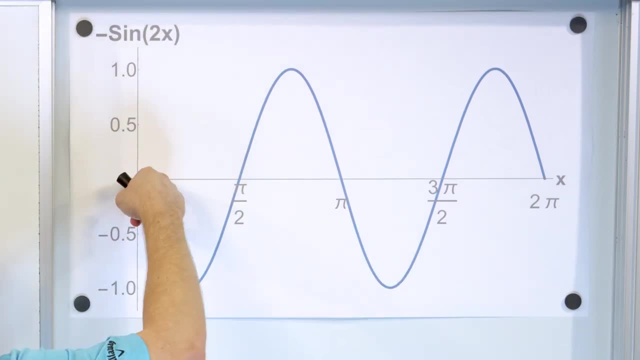 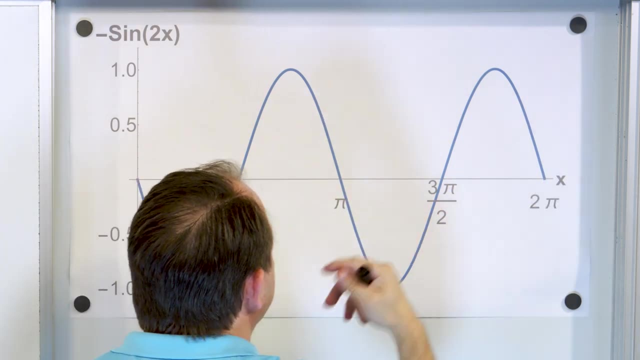 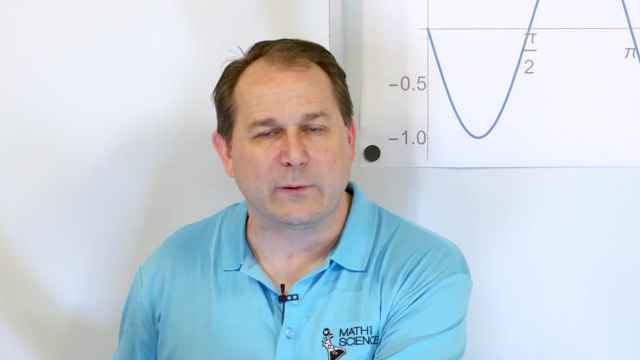 This is a graph of negative sine of 2x. It starts at the origin, It goes down, up down, one cycle over another cycle, So we have two cycles over a two pi period, and the thing is inverted. So now what I'd like to do is take some of these down, Erase what I have so far, Talk a little bit more about the 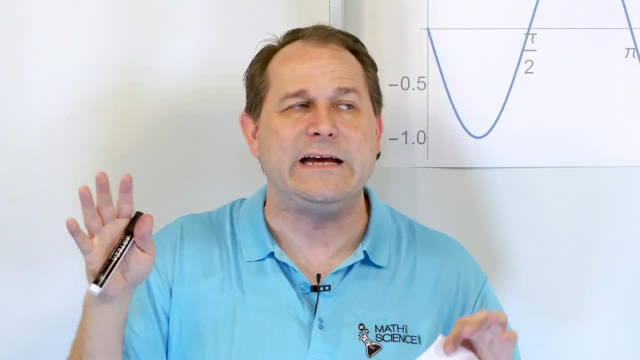 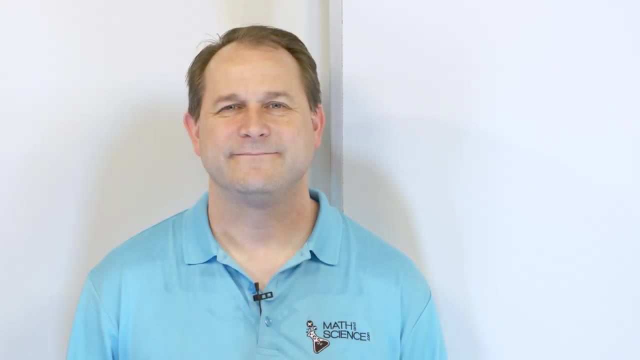 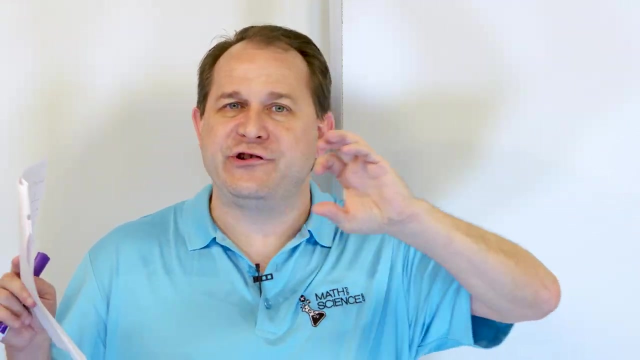 phase shift, Why the phase shift works. Why does it mathematically shift the function to the left or to the right? And then we'll do a couple of problems to wrap up this lesson. All right, now. the next thing we need to do is really understand, or maybe remind ourselves, why a phase shift like 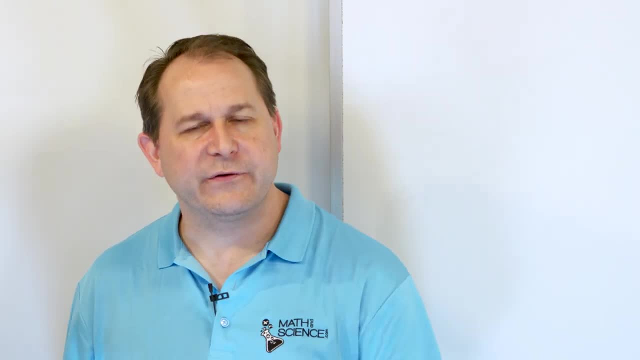 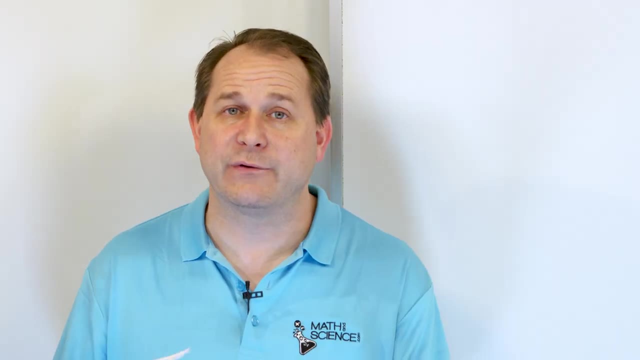 that actually shifts A cosine or a sine. The first thing for you to remember is that it's not just cosines and sines that we can do. We can shift these things. We can shift any function and we have learned it in the past. So it's something you already know. you just may not be aware of it. So if we take 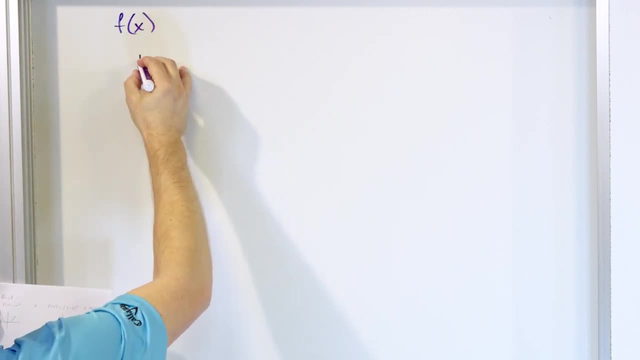 for instance the function. So let's pick something that's not a sinusoid, Let's pick a sine, just a regular function, Probably the easiest function that's not a straight line, is just a typical parabola. It goes down here, goes up like this: And so that's: f of x is equal to x squared right. 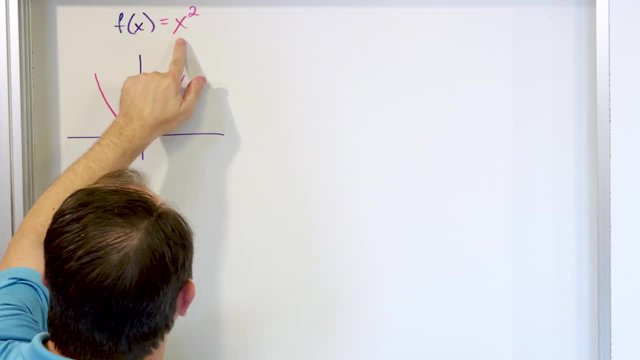 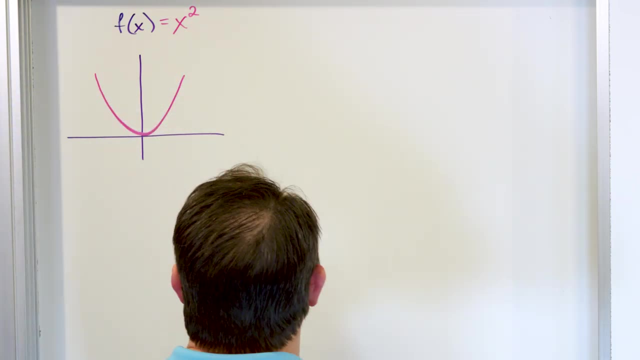 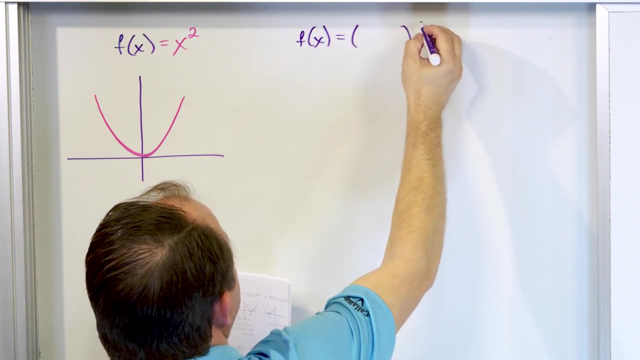 So what we're basically saying is that we can change, make a modification to the variable there to shift this graph to the right or to the left by however many units we want Right. So let's, for instance, take a look at the function. f of x is equal to, instead of x squared, we'll still have. 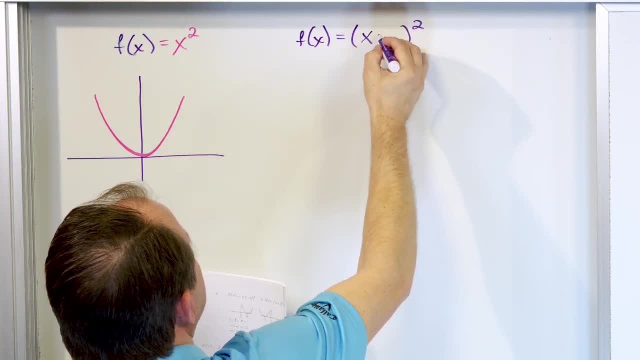 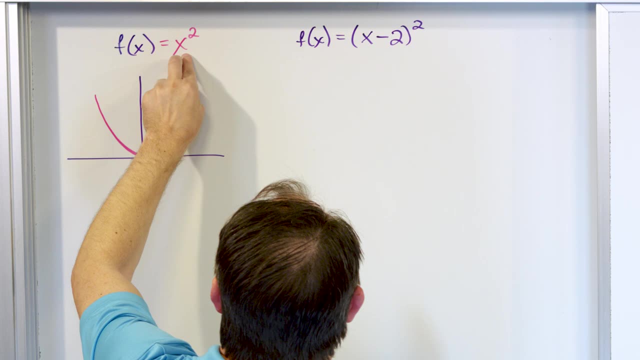 something squared, but we're going to replace the variable with x minus, let's call it minus two. So what you're doing is you still have a quantity squared, but what? the thing that you're squaring is not just the variable, it's a variable that's going to be squared. So we're going to change the 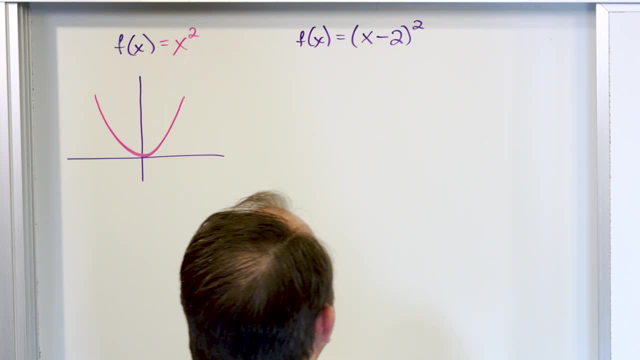 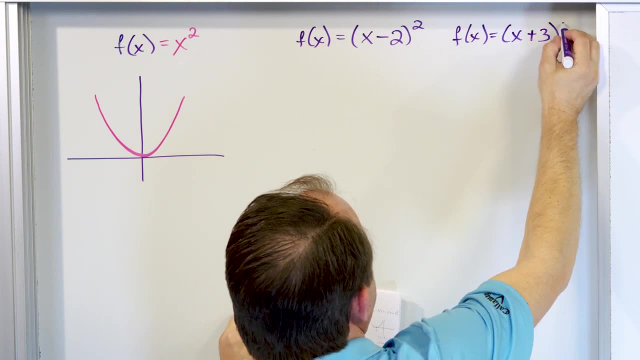 minus a number. And then we'll also do the same thing with variable plus a number. We'll do the same thing here. f of x is equal to x minus. call it minus three or plus three, sorry, squared, just for some variety, All right. So let's go and do that. The first one here I will draw. 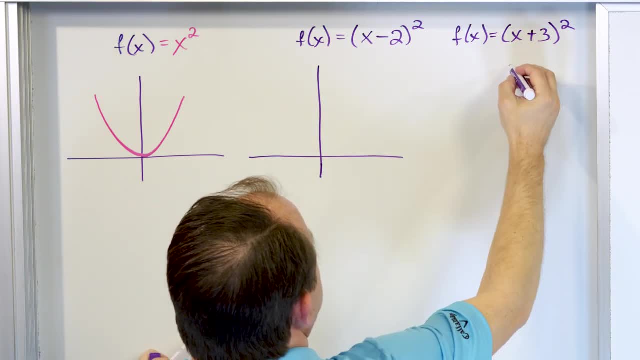 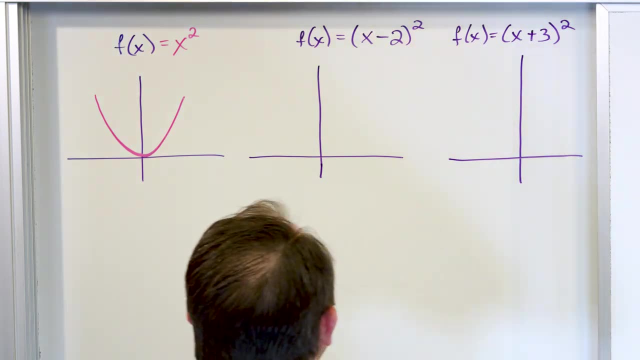 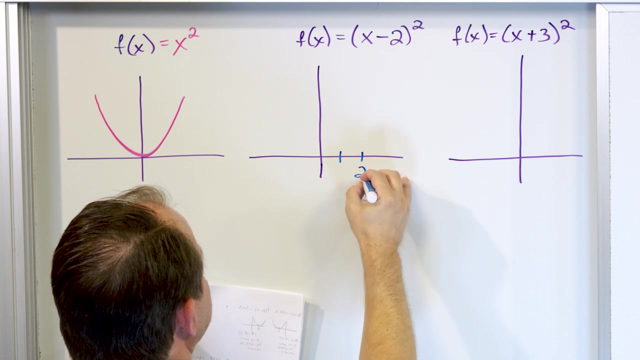 relatively close by and try to leave enough room to do this. one right here, Right. So this is the situation we have. So what I'm telling you is what this is going to do. this x minus two minus signs shift the base function to the right. So one, two, so this is a positive two, And then the 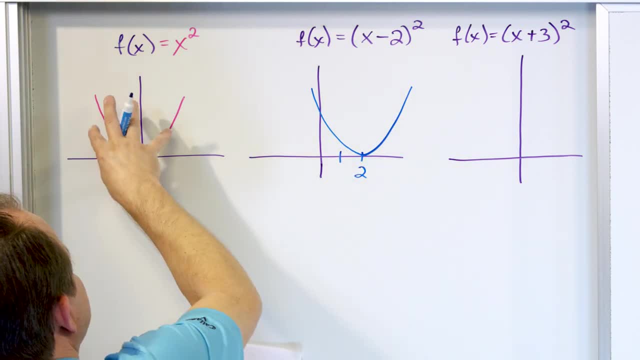 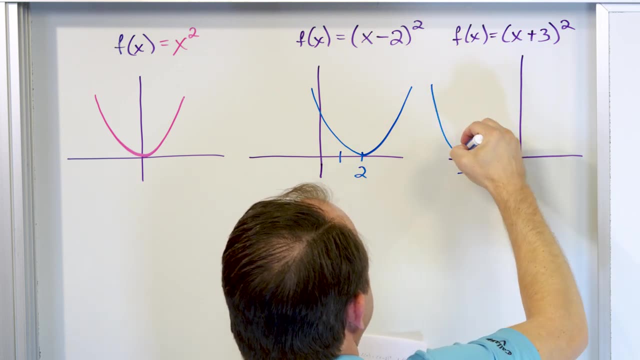 parabola is going to go down and touch basically right there and go up. the entire graph is shifted over and plus signs shifted: negative, one, negative, two negative, three units to the left, And so this one is going to go down like this. Now the question is: you can memorize that, But why is it that? 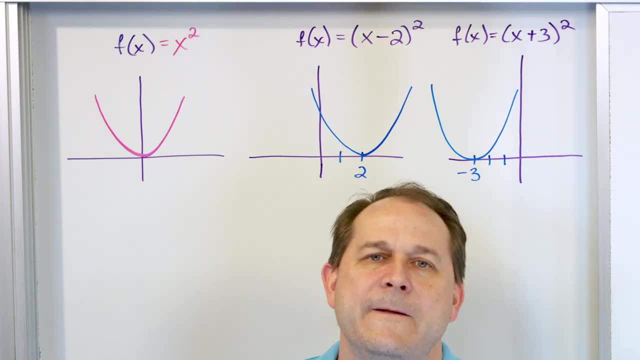 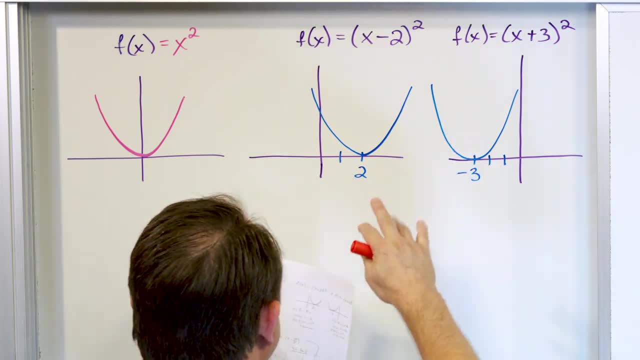 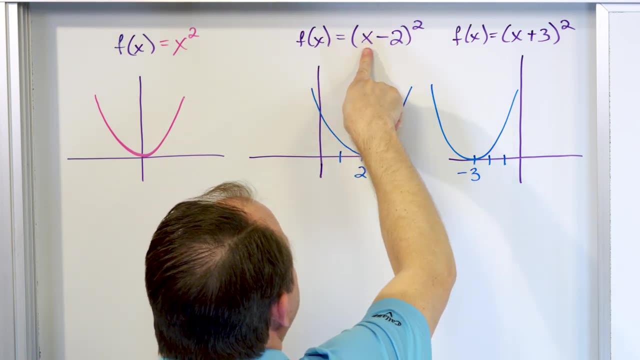 kind of think it should go that way. So the way you do this, the way you visualize this is what you do- is you say, okay, this is a new function, it's going to be graphed somewhere. what happens if I put a two into this function? if I put a two into this function for x, then it's two minus two. 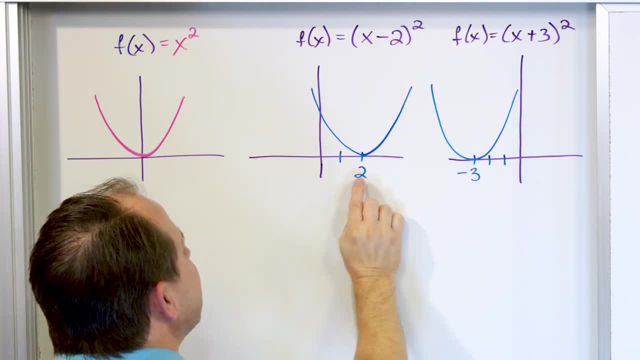 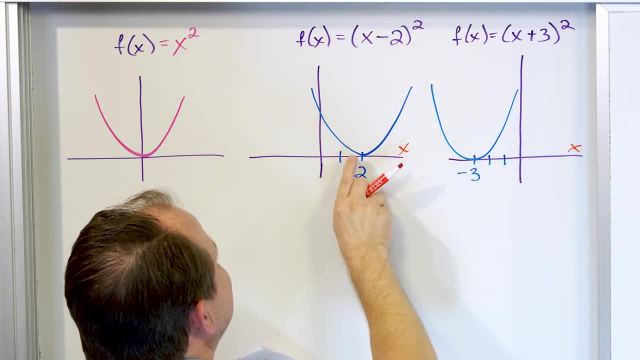 which is zero. zero squared is zero. So at the number for an input value of x is equal to two. this is the input, the x here, what it produces as an output is zero. So that means because the only point on this graph is: 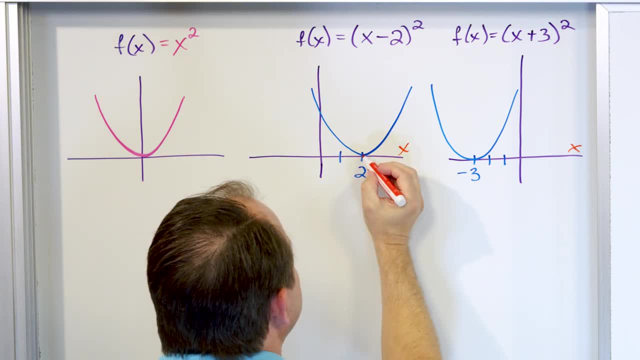 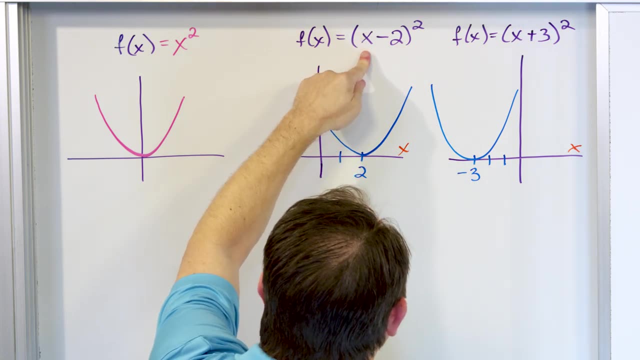 the only zero on this graph is right here at the very bottom. So if it's producing a zero, that has to be the bottom of the parabola, All right. and then if I put like three into this graph, then I'll get three minus two, which is one, and one squared is going to be like one unit. 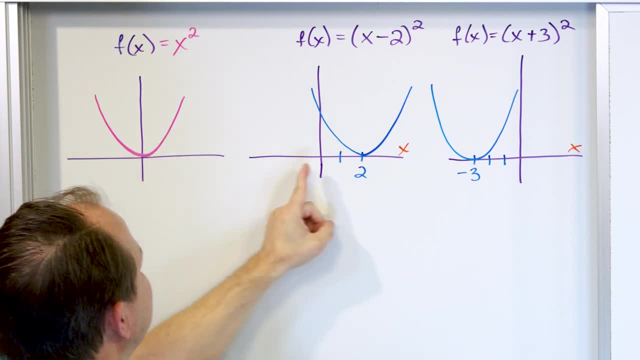 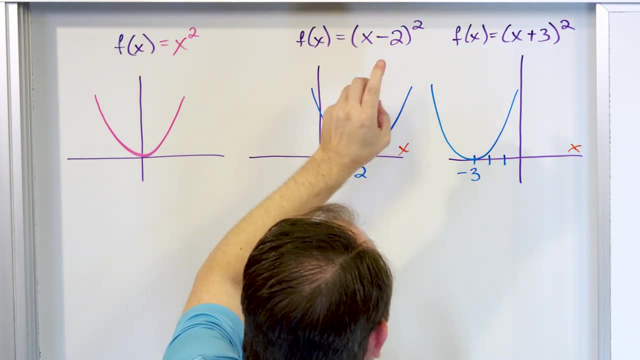 to the right of my zero point. it's going to be like returning this value, but it's going to be returning it one unit to the right of the number two. If I put four in here, then it's going to be four minus two, which is two, and two squared is four, So it's going to be like originally. 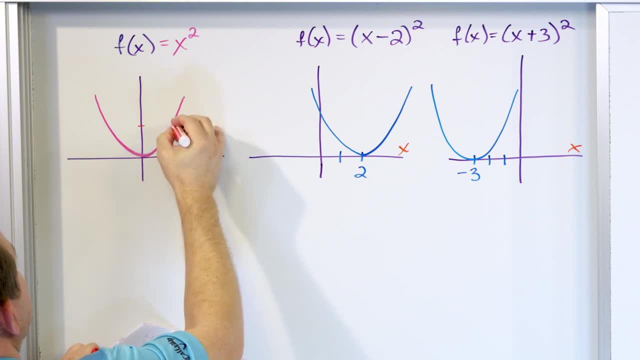 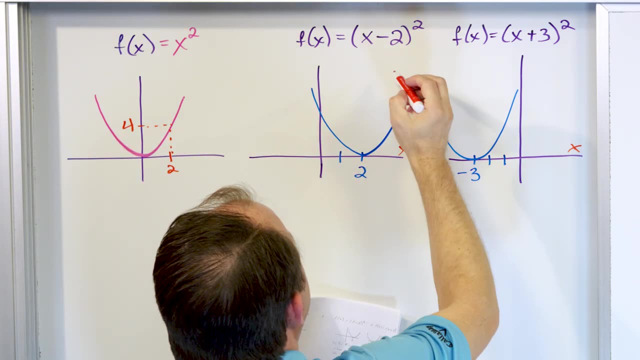 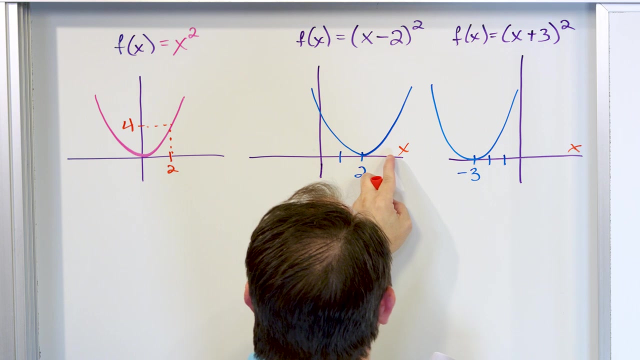 over here there was two and then there was over here four, because two squared is four like this. So at an input of two, an output comes a four. But over here I have to put an input of four in to get the two to square it, to get the four. So it's going to be two units to the right. 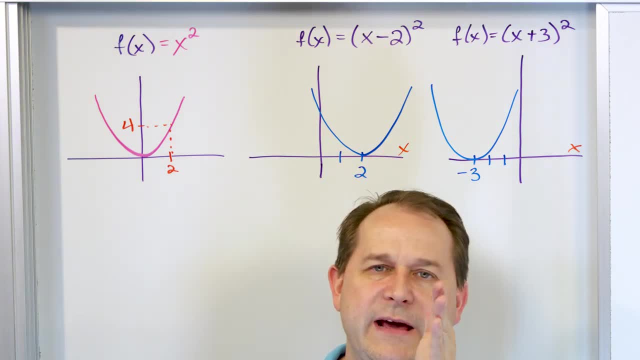 here. So you see what's happening. it's almost like for every function you need to pick like a zero point. just think of where the x- y axis crosses at zero- zero, where is the function there? And then that as you move it and shift it around, that's kind of your zero point of the function And that is. 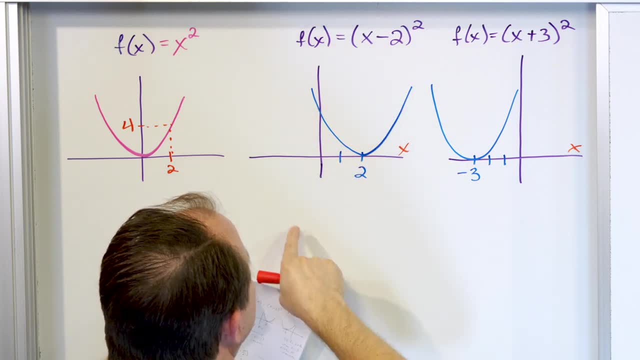 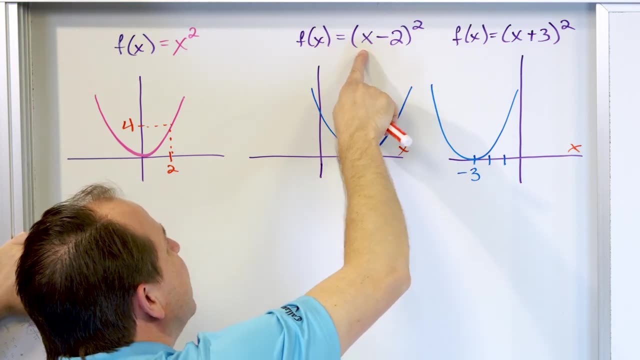 going to move with the shift. So we know that it has to shift two units to the right, because putting this x minus two here means that I have to put in bigger numbers for x to get zero here, which is my zero point of the function. the original zero point is down here at the origin. 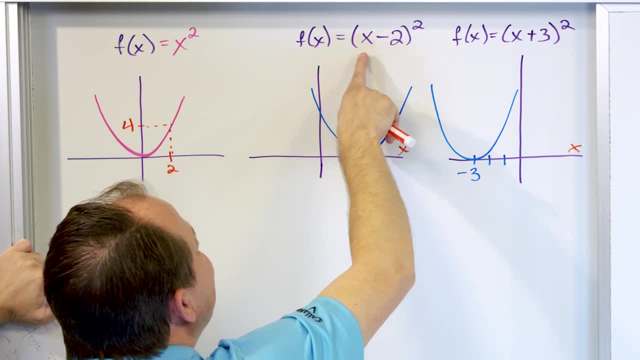 But here I have to put bigger values of x and I have to put two in just to get a zero to square it here, And then I have to put even bigger numbers in to get on the right side of the parabola. 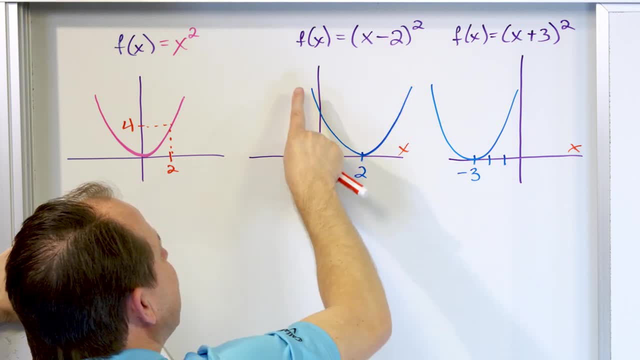 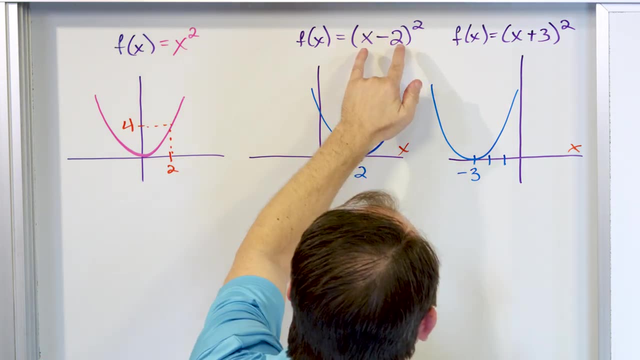 And then slightly smaller, lower values than the number two to get this. So it shifts every point to the right, because this is changing my zero point All right, meaning the value. to get a zero squared here I have to put a number in bigger than I did over there, because here I only have 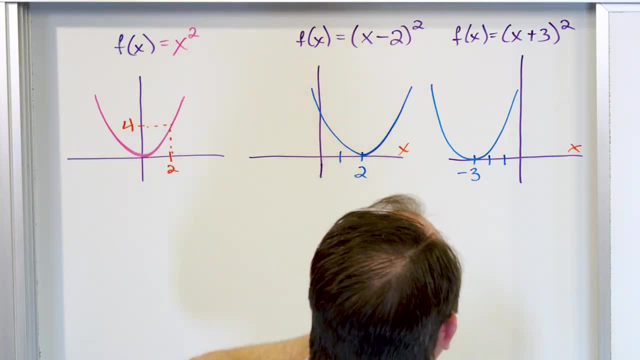 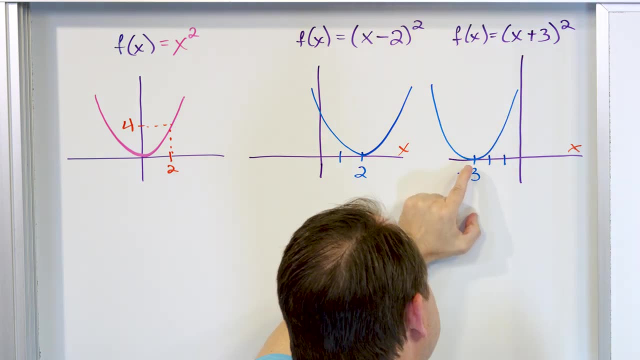 to put zero in. to get zero squared Here, I have to put two in. to get zero squared. What happens here? What do I have to put in here? to get zero squared, I have to put a negative three in. That's why the zero point is shifted to the left, Because putting x plus three means I have to put. 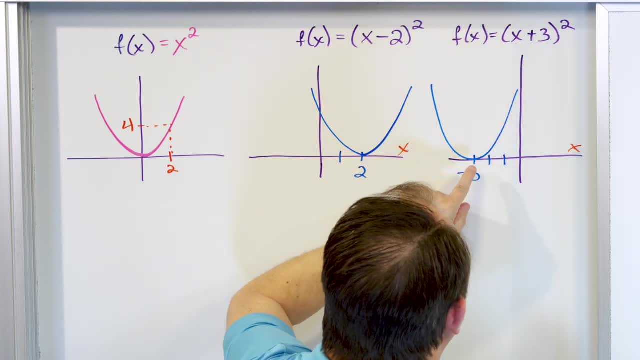 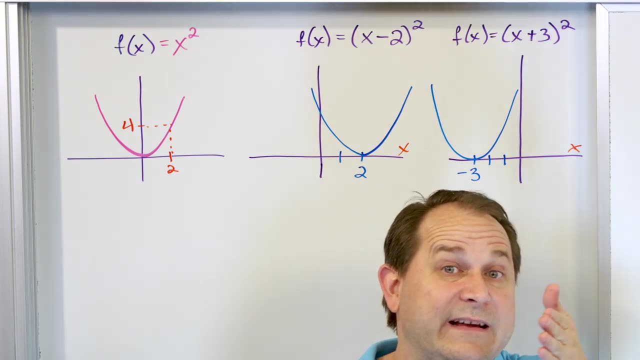 the negative three in in order to get zero squared, which is the bottom of my function here. So that's why the signs are flipped from where you normally think. The minus sign shifts the thing to the right because it makes me put larger values in for x. 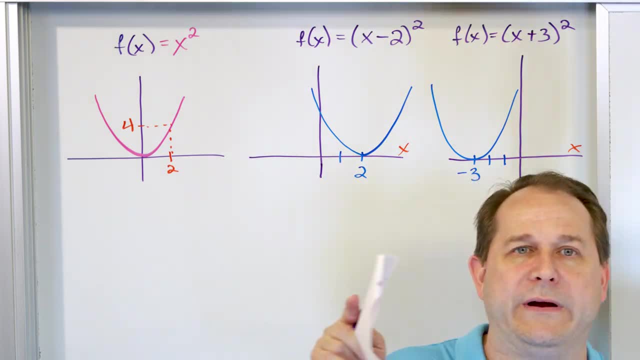 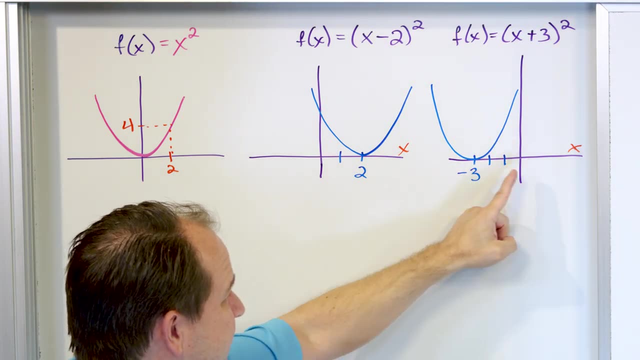 than I usually do for the base function And so. but that happens for all points, so it shifts it all to the right. And if I have x plus a number, then I have to put smaller numbers in, in this case, negative three. I have to put smaller numbers in in order to get to the zero. 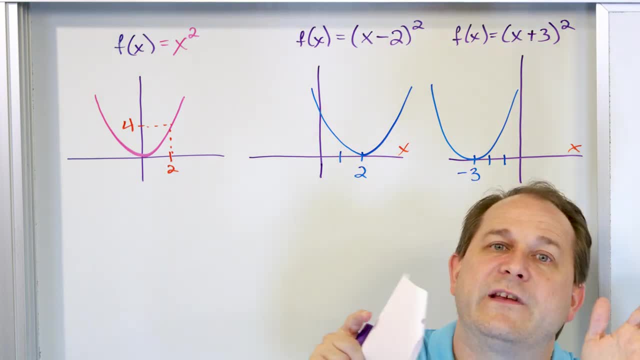 point of my function. And all of them are shifted that way, so it shifts it all of them to the left. So minus signs shift to the right, plus signs shift to the left. That is what you need to remember And the y of it. I hope you remember. but, honestly, if you just remember that, the rule 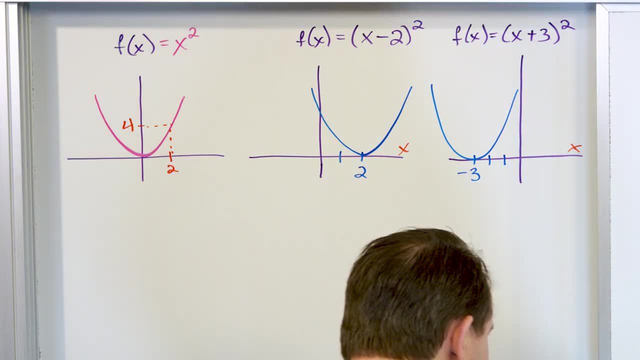 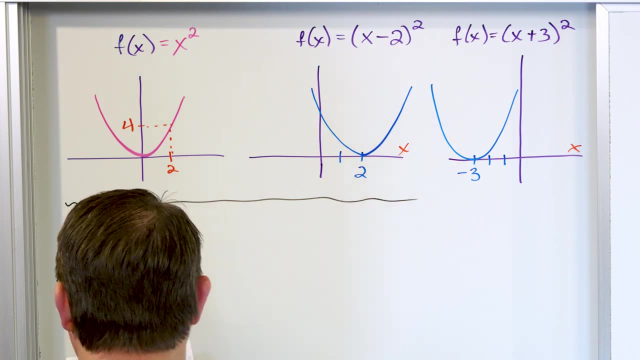 I'm okay with it All right now. what we want to do for our next problem is we want to actually shift and do an actual shift to generalize this, And we've actually done this before, but we're going to sketch it and then we'll look at it later, And then we'll look at it later. So 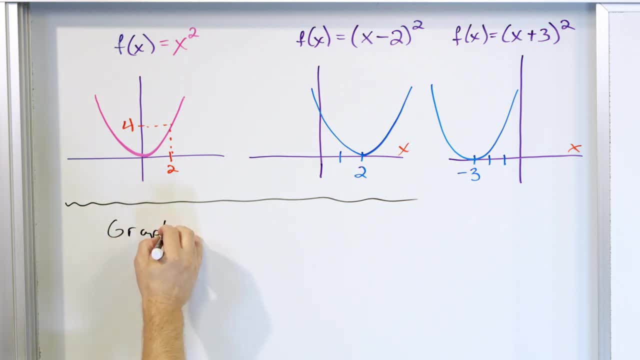 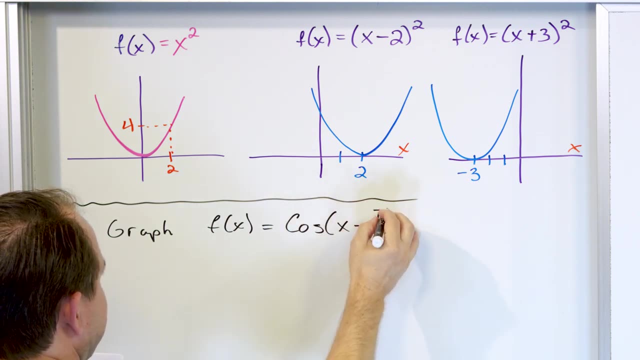 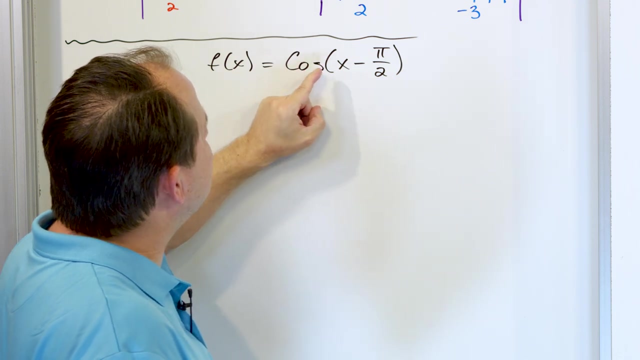 we'll look at a picture here. Let's graph or sketch f of x is equal to cosine x minus pi over two. x minus pi over two. So before you do anything, the way you read this is okay. I've replaced the cosine of x function. I've replaced the x value with something else. 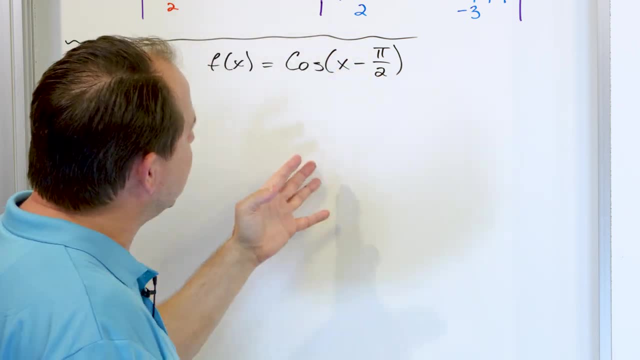 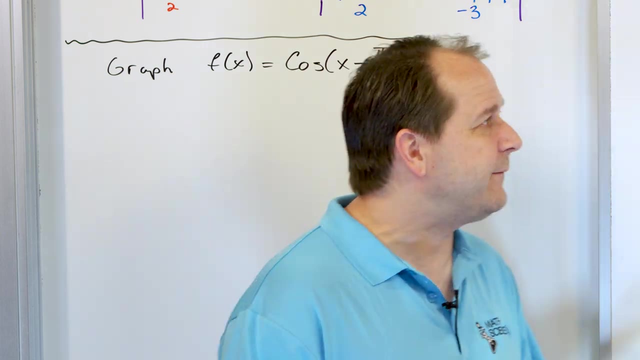 and it's x minus a number. Yeah, it's pi over two and it looks like an ugly number, but it's just x minus a number. So what this minus sign is going to do is shift the whole thing to the right. How much does it shift By the number pi over two? Pi is 3.14,, so pi over two. 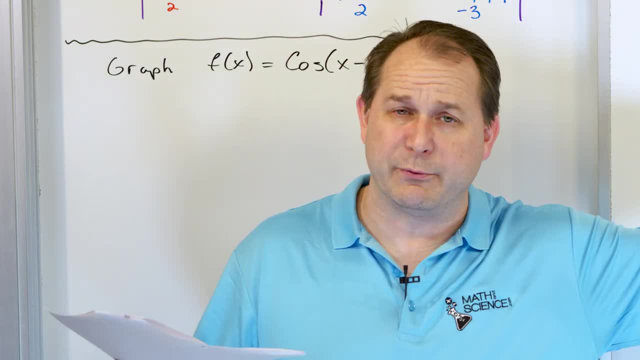 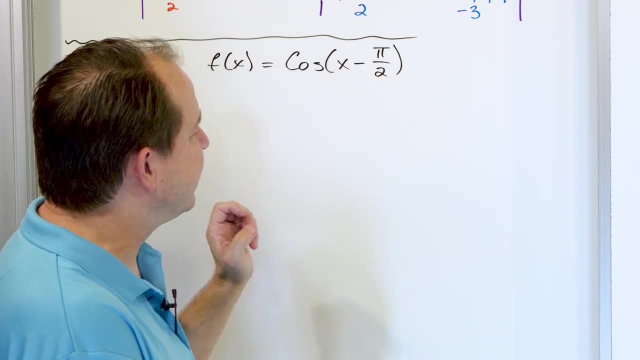 is like 1.57 or some place close to that, with decimals that go on forever. So it's shifting the cosine, entire cosine curve, to the right because of the minus sign by about 1.5,, a little bit more than 1.5, which is exactly equal to pi over two. So the way you draw these, 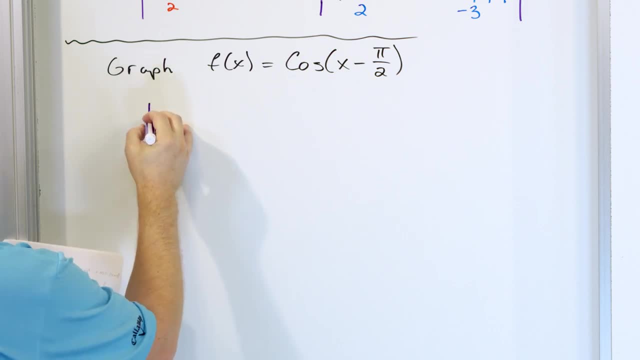 things is: first you need to shift the or draw the original function before you try to draw, in my opinion, the shifted version of it right, We know it's a cosine, so we know it can only go up to a positive one or a minimum of negative one, And we know that a regular cosine there's still. 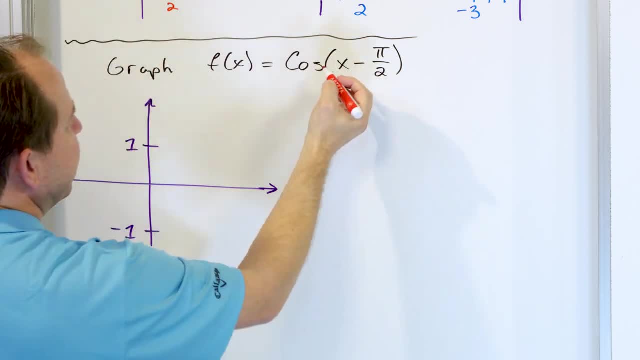 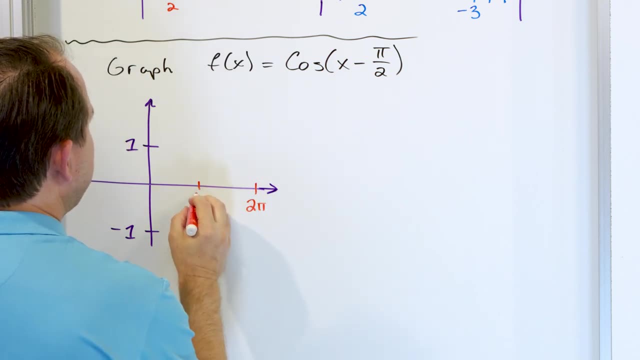 nothing in front of the x: the speed multiplier, the frequency. there's nothing in front of the x other than a one. So it's still going to have a two pi period, and this is pi right here, and this is pi over two, and this is three pi over two. Now I'm drawing the original. 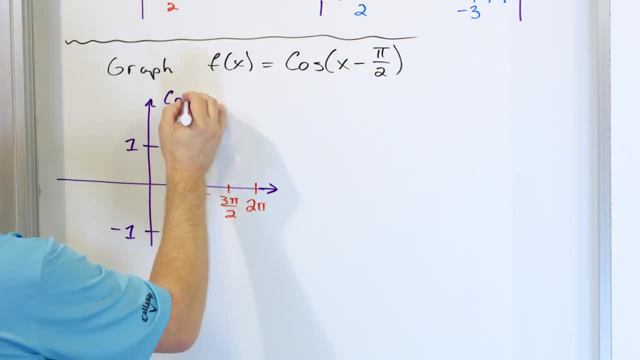 unshifted version to compare with. So cosine of x is what I'm drawing here. How would that work? Or how would that look like? We start at a maximum, we go down through here, we go to minimum at pi, then we go up through here and then a maximum at two pi. So that's one full cycle, right? 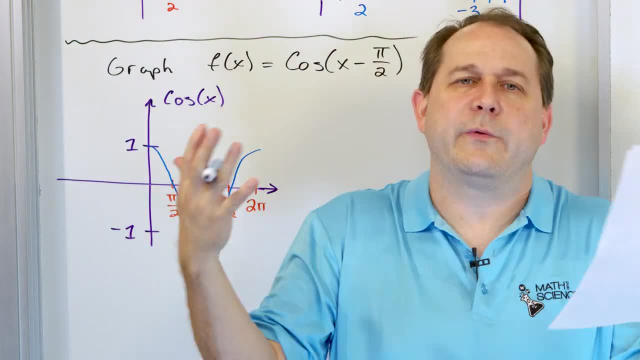 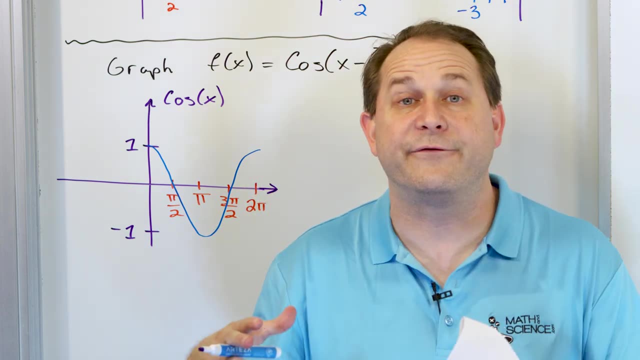 We want to draw usually the unadulterated version so that in our mind we can start applying changes to it. If you try to draw these functions without drawing the baseline function, it gets very confusing, especially if I start doing multiple things. 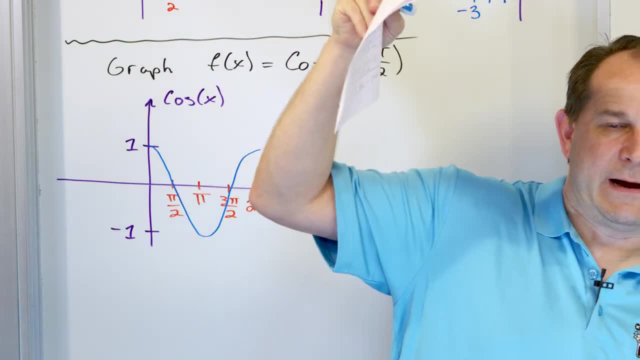 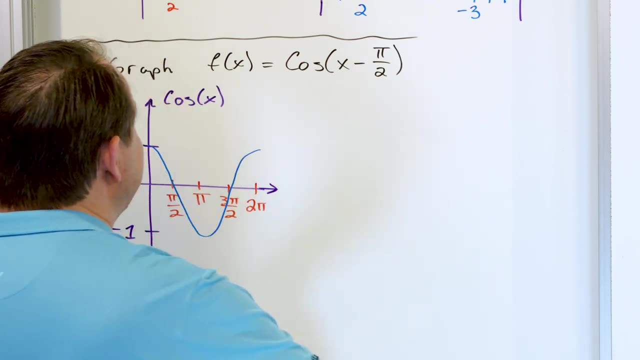 to. you know, if I shift it up, phase shift it to the right, change the amplitude, then everything gets very confusing. So you have to draw a baseline. This is the baseline cosine function. Now that we have that on paper and we can look at it, then we can more easily figure out what to do. 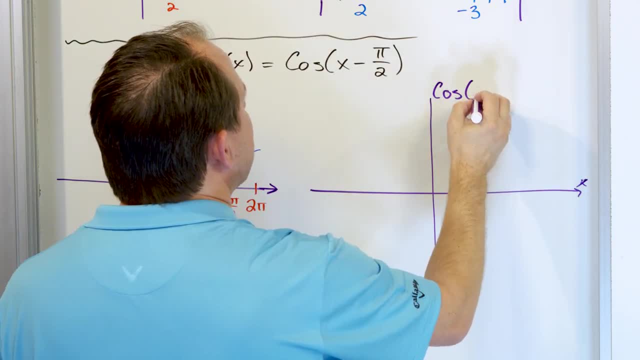 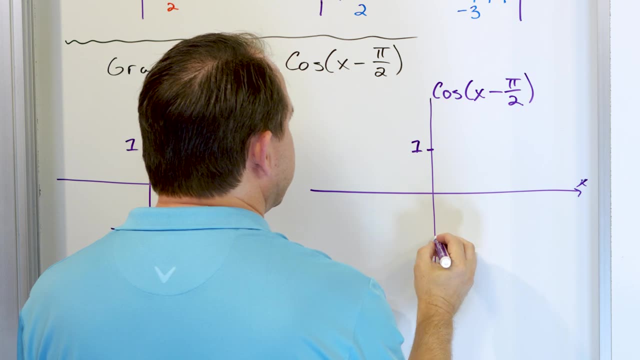 over here. And so here we're going to plot cosine of x minus pi over 2.. All right, So again, the first thing we know is that it can only go up to a positive 1 and a negative 1, because there's. 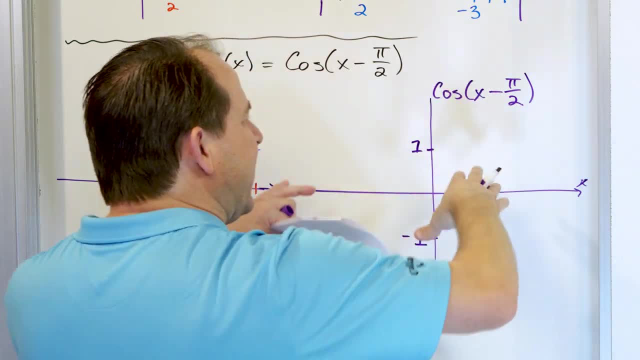 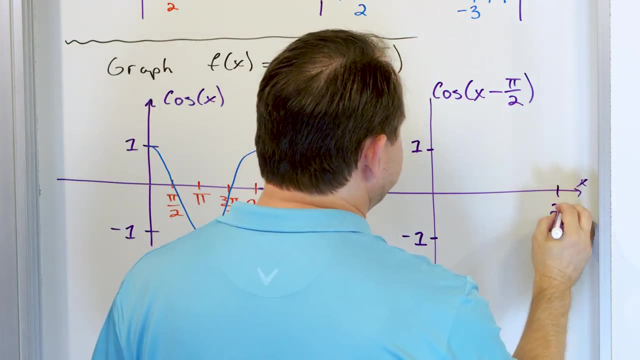 nothing in front of the cosine And we know that there's no shifting up or down, So we're not going to do anything like that. There's nothing in front of the x other than the 1.. So it's going to have a 2 pi, a 2 pi period, And so, again, this is pi, and this is pi over 2.. And this is 3 pi over 2.. 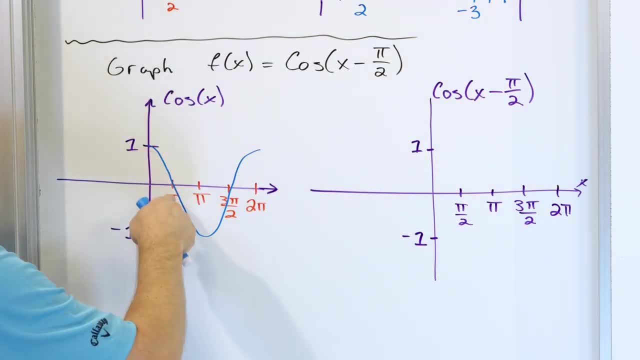 All right, Now what's it going to look like? Well, the original cosine function did this, So it's like taking this thing And also it's helpful to also kind of like continue this down Off to the left here. So I usually draw it like this: but this peak continues down here And since 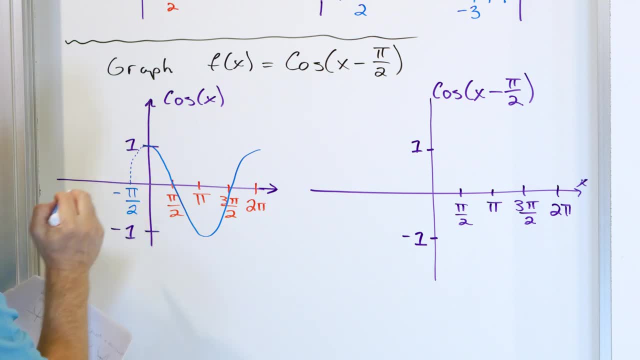 this is at pi over 2, this is going to be at negative pi over 2 right here, this crossing point. So if I grab this function, if I could just grab the blue curve and move it to the right by pi over 2, that's what my shift is- Then this bottom point is going to be here The crest will. 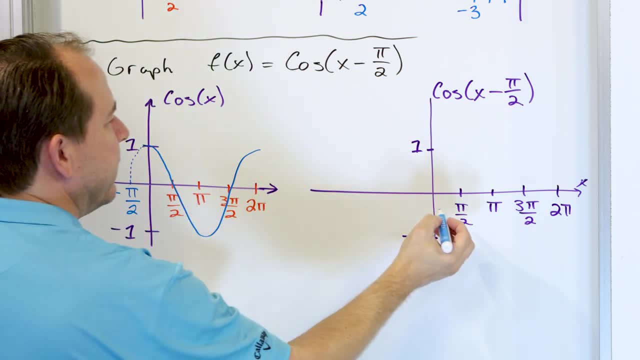 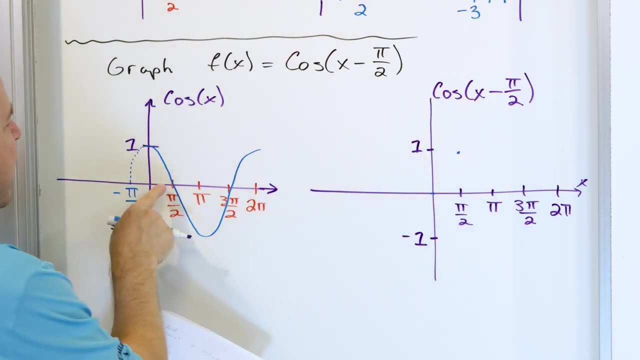 be up here and then every point will move. So the bottom will be at the origin. The peak of this thing, right here, where the top of the cosine is, is actually going to be at the bottom of the cosine. So this crossing point is actually going to be shifted to the right by pi over 2.. This crossing 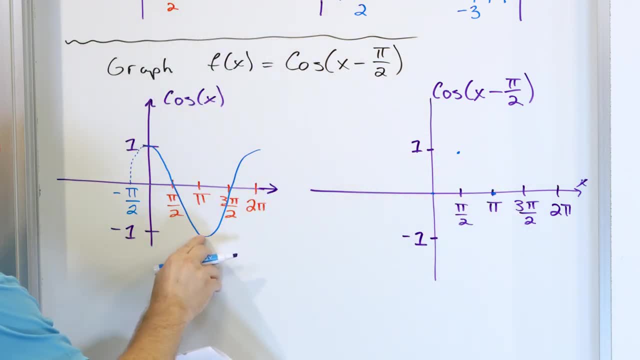 point will then go to pi. This trough which is at pi now is going to go pi over 2 to the right, which is right here. And then the- let's see right, where am I looking Here? And then this: 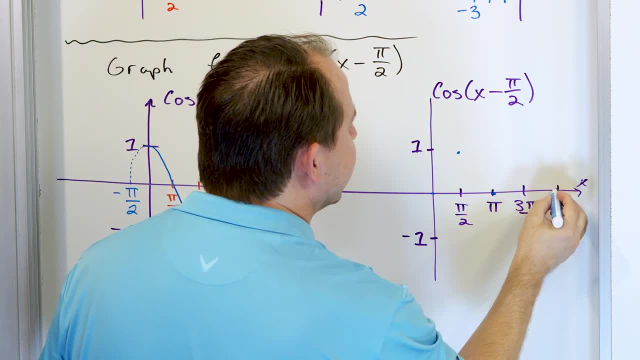 one here. this crossing point is going to now, then move to 2 pi right here. So let's see if we can draw it right. So what we have is it's going to look up, go up like this, Then it's going to cross. 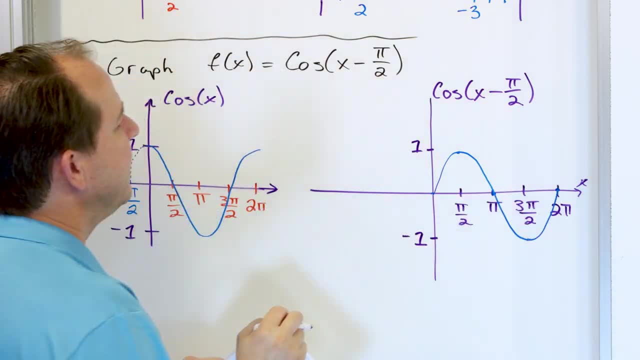 down through this point, Then it's going to go up through this and it's going to go up like this: So this is what cosine and cosine function is. So this is going to go up through this point And then we have x minus pi over 2 looks like. And what does it look like, ladies and gentlemen? It looks. 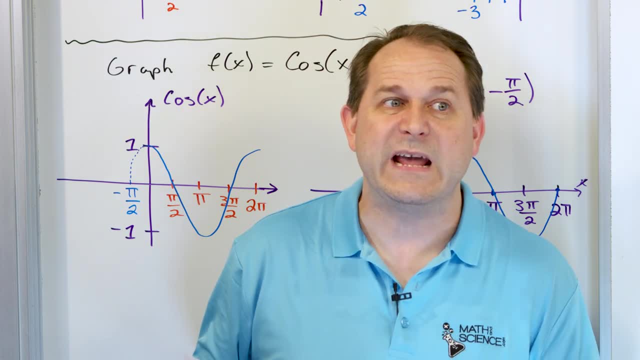 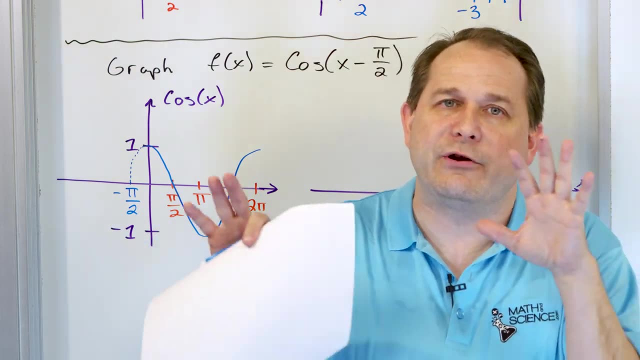 like a sine wave. Not only does it look like a sine wave, it is a sine wave Because all the points on the cosine curve are the same points as the points on the sine curve. They're all the same, They're just shifted relative to one another. Look at your table of trig values. 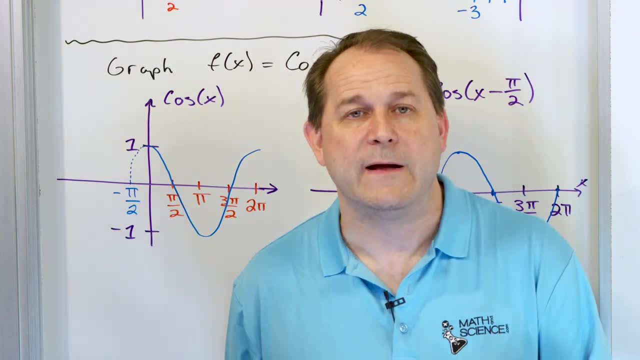 You know, sine can return one half. Cosine can return one half. Sine can return square root of 3 over 2.. Cosine can return square root of 3 over 2. And all the negatives they can both return. 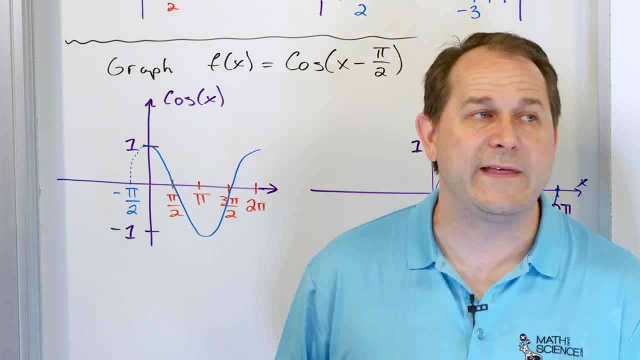 square root of 2 over 2.. And all the negatives: they can both return square root of 2 over 2.. They can both return 1.. They can both return minus 1.. They can both return 0.. They're all shifted. 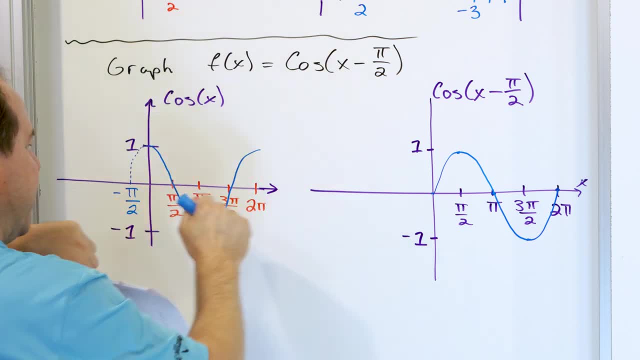 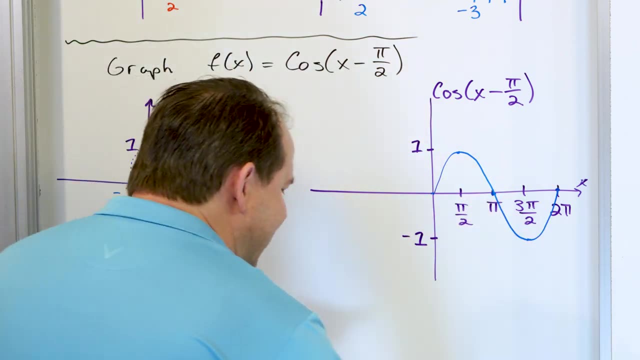 relative to another. And when we grab this function literally and move it by this much, by pi over 2,, then it literally becomes a sine function. All right, So I've got it written down here. I don't feel the need to write all the words, But what I wrote in my paper is exactly. 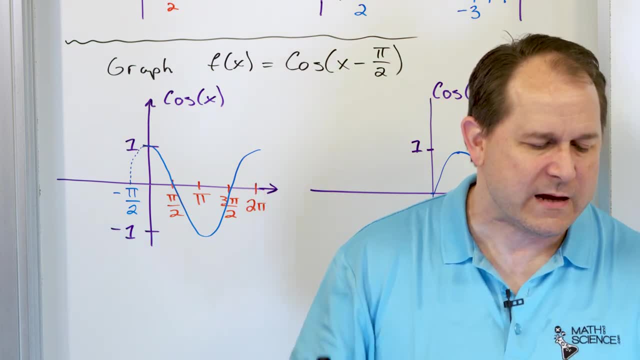 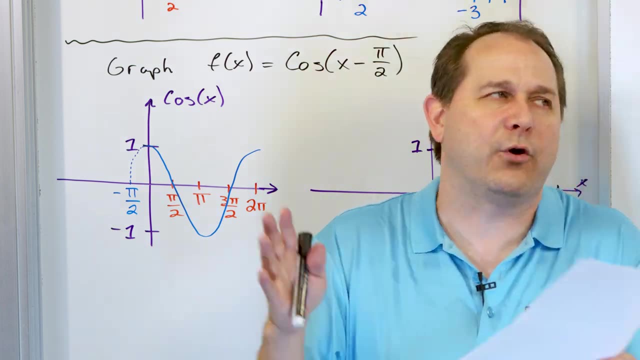 the following: Sine and cosine are identical shape. Sine is just a cosine that is shifted right by pi over 2 along the x-axis Or along the angle of the theta-axis, Because these are all the x variable we often rename. 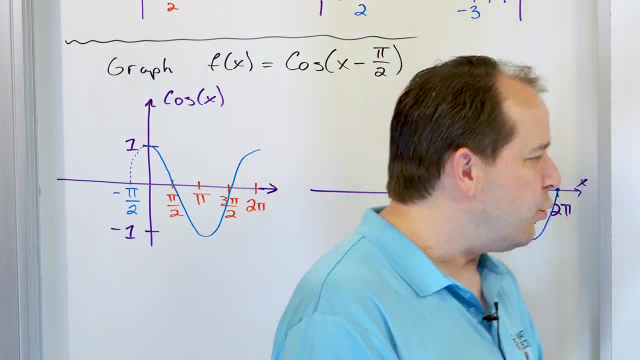 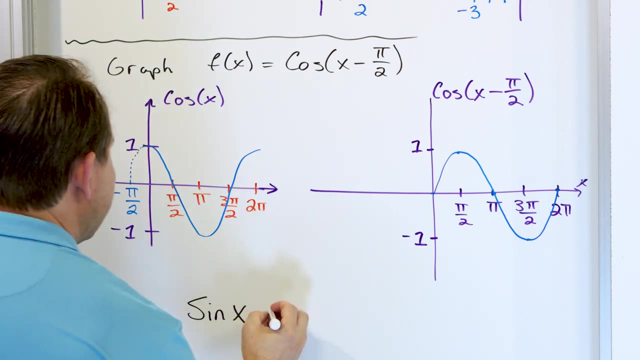 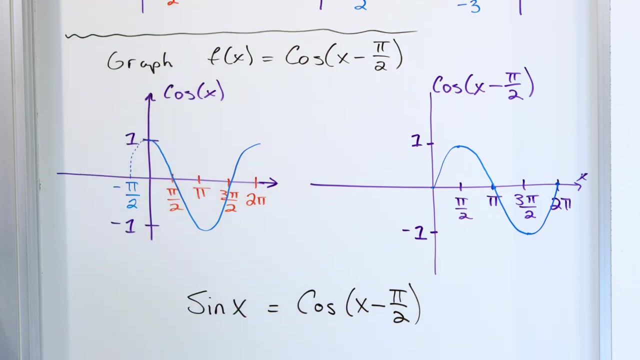 it to be theta, which is an angle measure, right, And so what you can then say with certainty is that the sine of any angle x or theta- whatever you want to put in there- is equal to the cosine function shifted by pi over 2 radians. This is a trig identity. 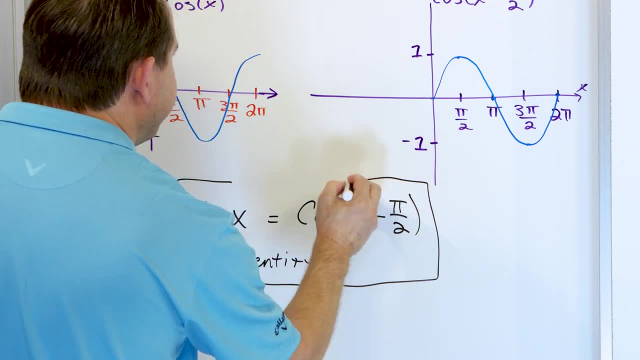 Now we're going to get into trig identities a lot more later. There's a lot more to it. But I'm going to get into trig identities a lot more later. There's a whole bunch of them, But this is the kind of thing you see in a book and you 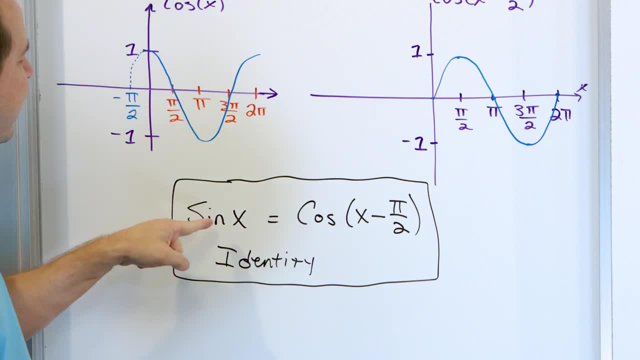 don't even know why it's there and you're just told to memorize it. What we're saying is that the sine curve, if you plot it, and the cosine of the curve, x minus pi over 2, if you plot that, if you overlay them on top of each other, every single point on the sine. 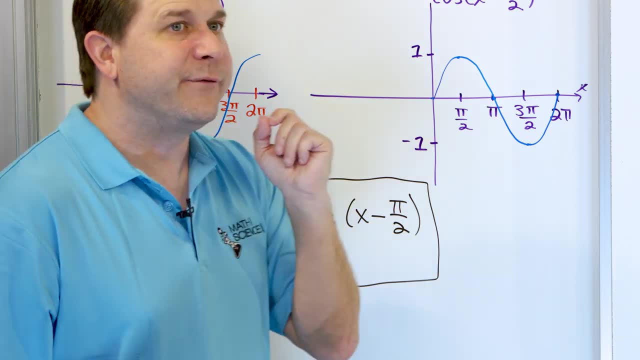 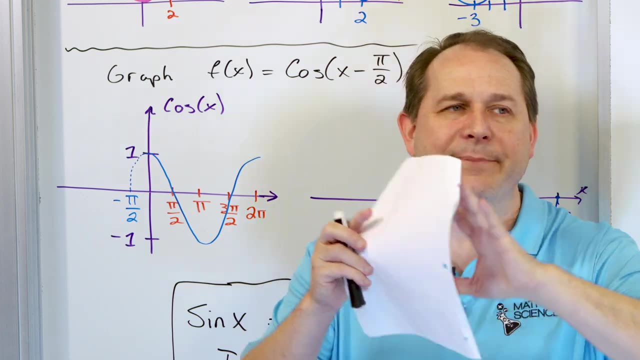 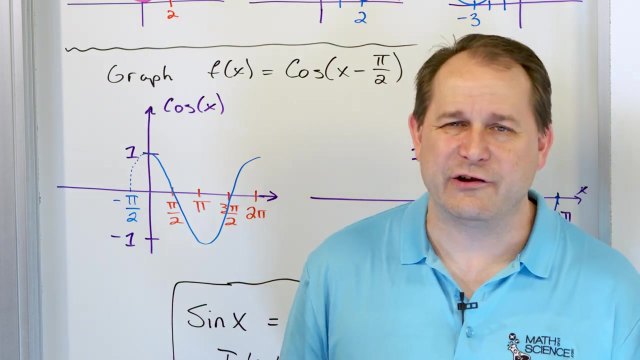 curve will line up with every single point on this curve. Therefore, both functions are identical, And when we say that there's an identity in math or in trig, it means there's an absolute equality between two things. All right, So it's kind of like. I don't want to give a general analogy, but there's just. 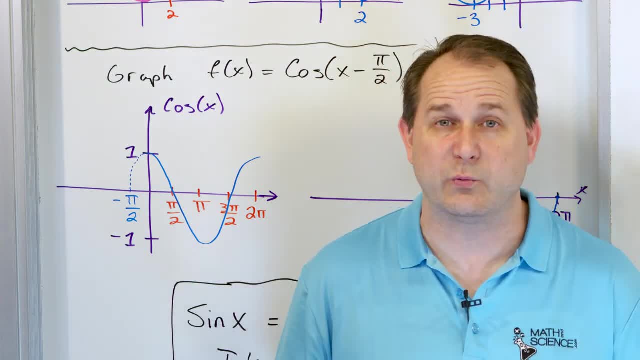 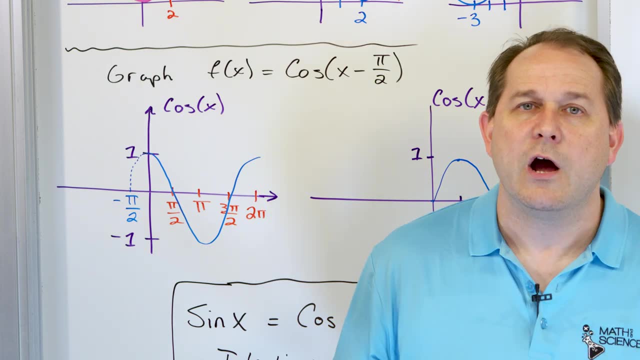 different ways of expressing things in math, like there's different ways of expressing things in real life. In real life, I might say it's sunny, or I might say it's no clouds in the sky. Okay, So if it's sunny and there's no clouds out in the sky- and of course it's- 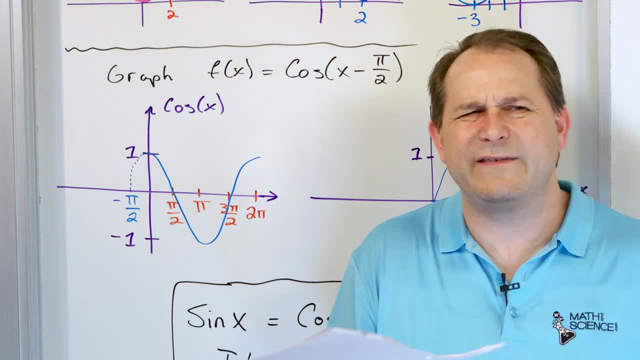 daytime, then you know that both of those are the same thing. They're identical, just different ways of saying the same thing. And what I'm saying is: this thing is exactly the same to the point where if I'm saying that there's no clouds in the sky, then I'm 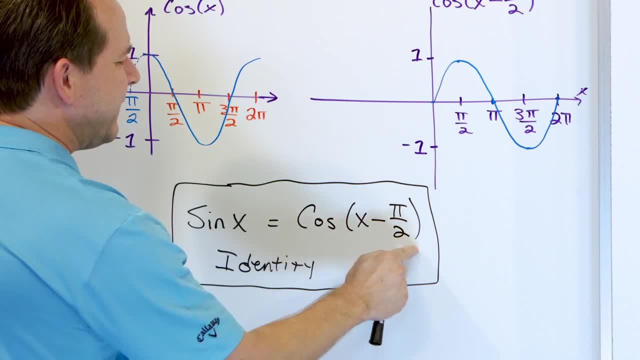 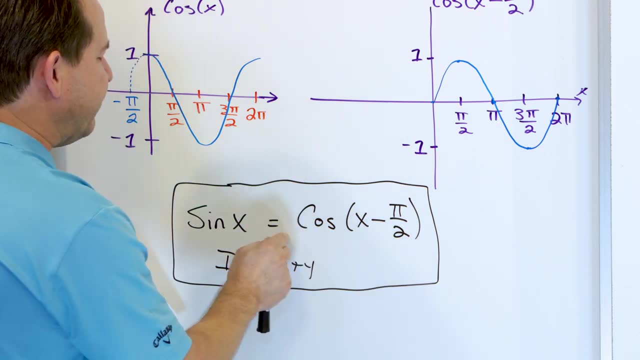 simplifying some equation that has this ugly thing in it and I'm like man, that's not going to be fun to play with. But then I remember: oh wait a minute, it's just equal to this. Then I can literally erase this from my equation and just replace it with this. 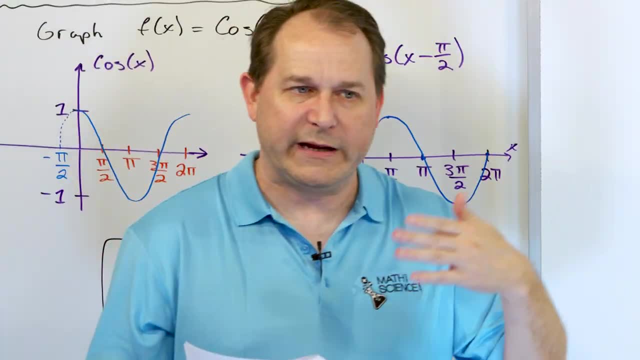 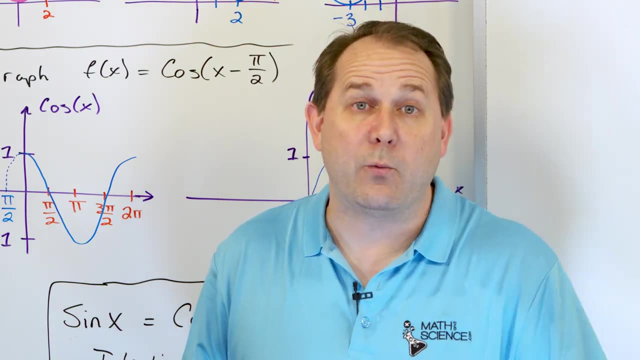 Because this and this are identical to each other, And in trig- and we'll get into it later- we're going to have entire tables of identities where one thing is equal to another, And this is one that I'm going out of my way to explain why it's true, because it has such 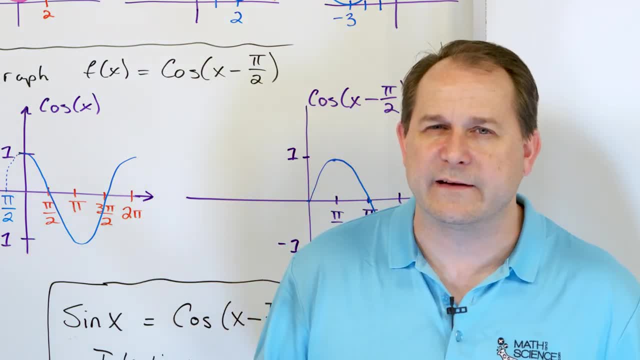 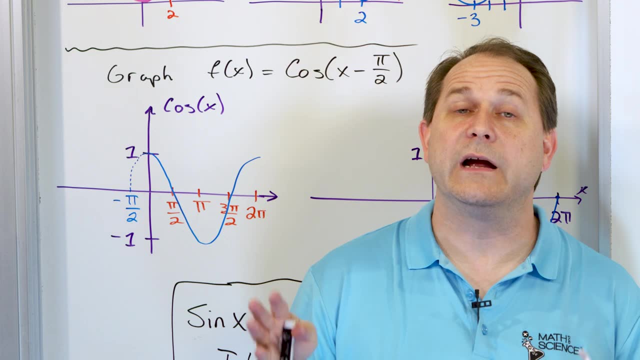 important consequences for studying sines and cosines and things like this. That's where it comes from, Because if you grab this guy, shift it by pi over 2, then you can get the other curve. So sines and cosines are identical, other than a pi over. 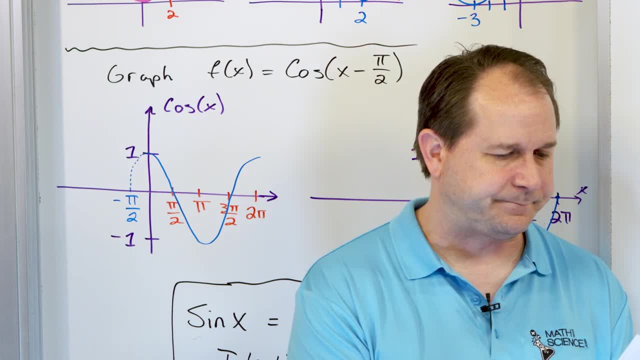 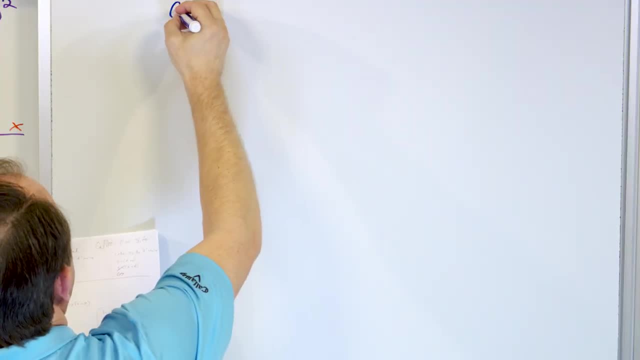 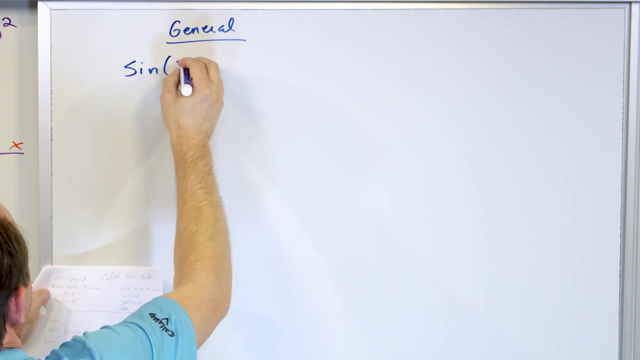 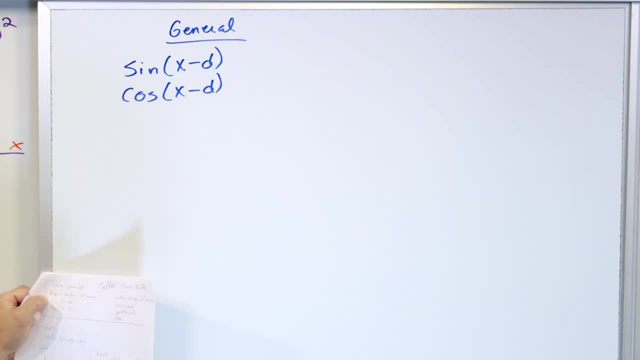 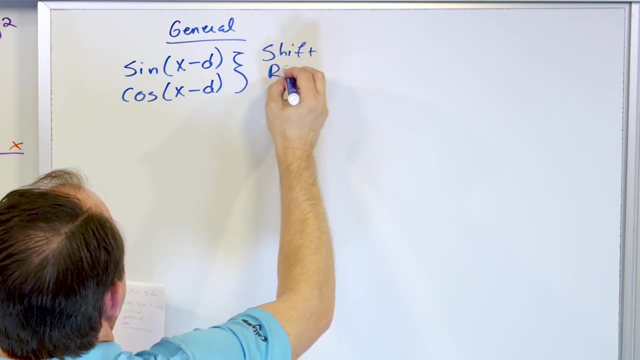 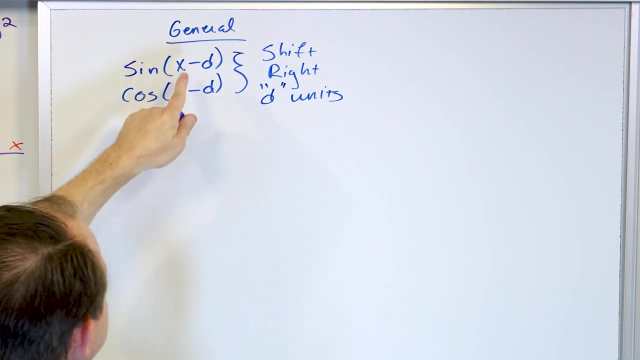 of x minus some shift, or cosine of x minus some shift, or cosine of x minus some shift, which d is just some number here. This is a. these two things are a shift, right d units, right d units. So if I shift it right by 5, then the whole thing gets moved to the 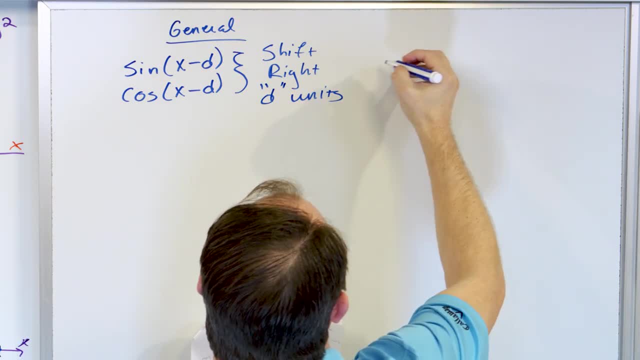 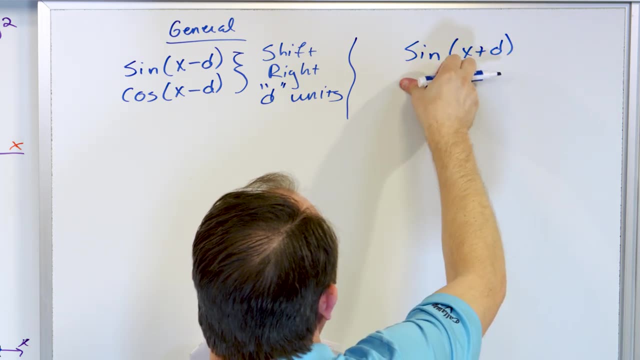 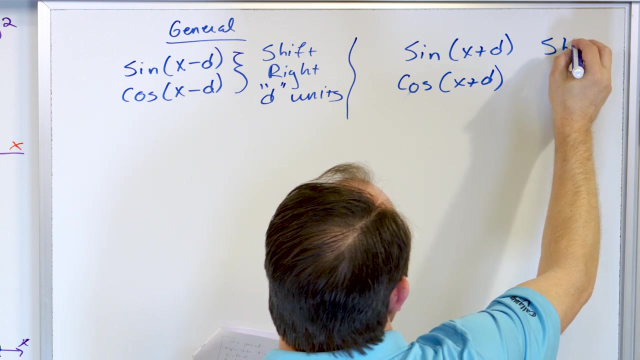 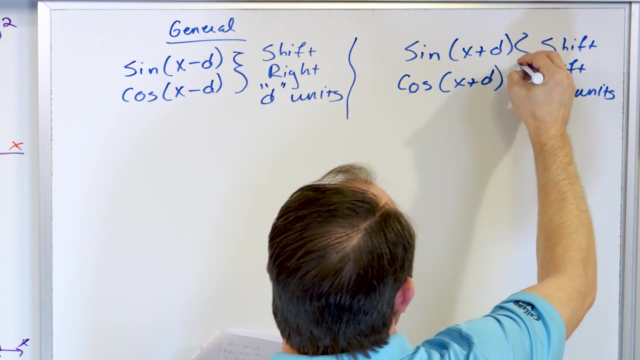 right by 5, or whatever it is, And you have the same thing of with a plus sign here. You could say sine of x plus some shift, You could say the cosine of x plus some shift, And this is a shift. left d units And we already went over y with the example there, with the 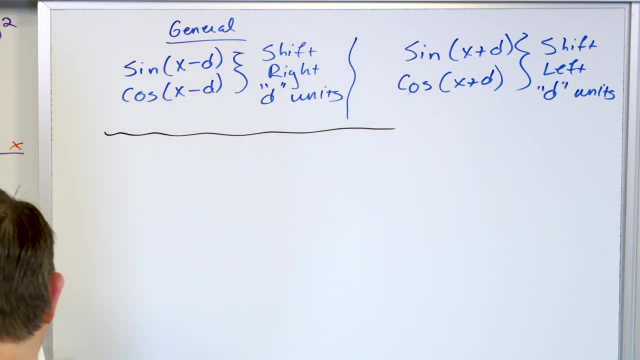 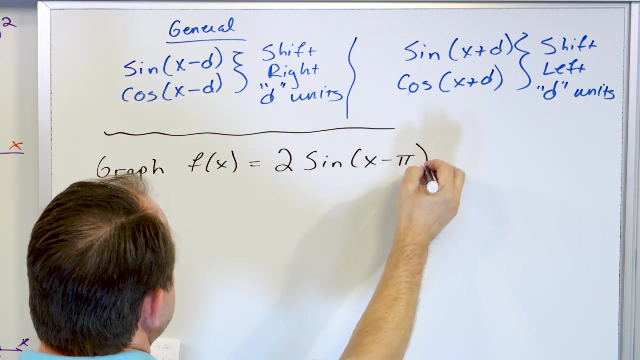 computer demo as well. All right, we're almost done. The next thing I want to point out, just to give you a little more practice with an actual problem, is the following: Let's graph f of x. f of x equals to 2 times the sine of x minus pi. Now you should start to look at these. 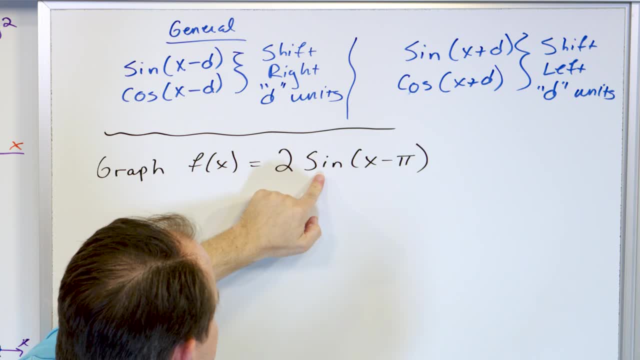 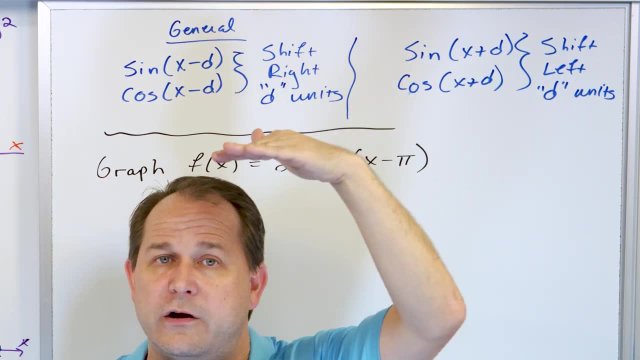 things and understand how to read them. The 2 means we take the basic sine shape and we change the amplitude. We make it go up to 2 and then down to negative 2.. We change its amplitude, make it taller, right. 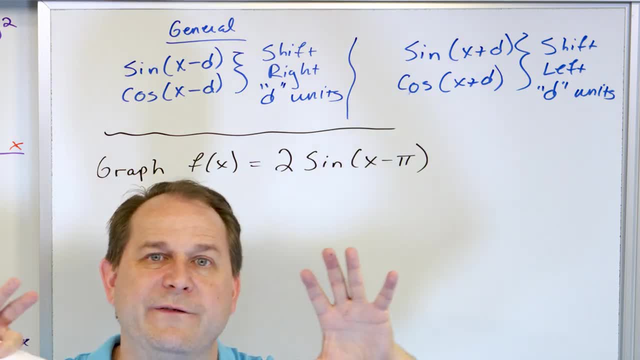 And then the x minus pi means, after we do that first step, we shift the whole thing to the right by pi units, And pi units is half of a period because all these sinusoids, the base period is 2pi. So we're going to shift it to the right one half of a period, which is pi units, And we're 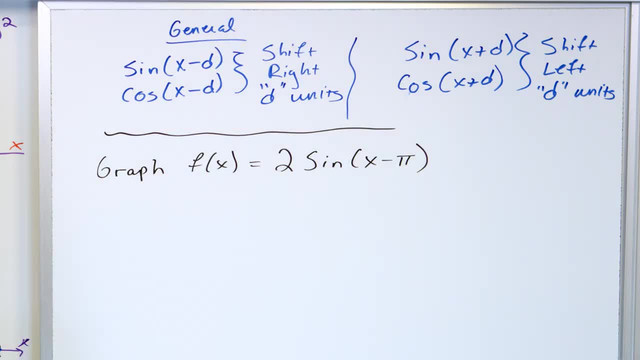 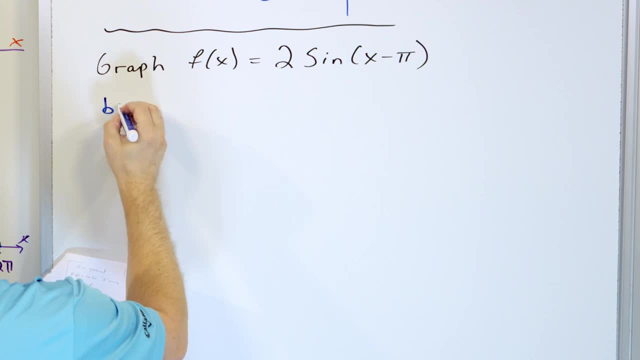 also going to stretch it vertically. Let's sketch this guy and then I will show you a nice picture of it to make sure you understand. So the first thing you want to do is you want to graph the base function. So we'll say the. 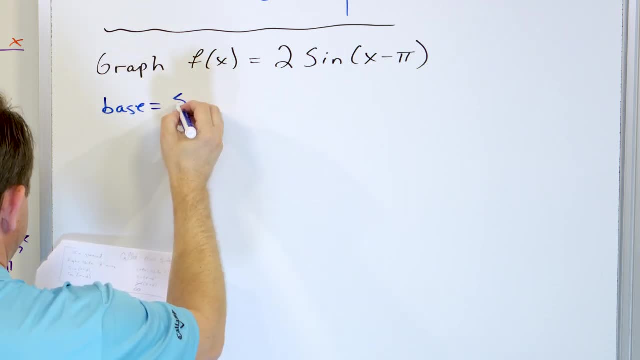 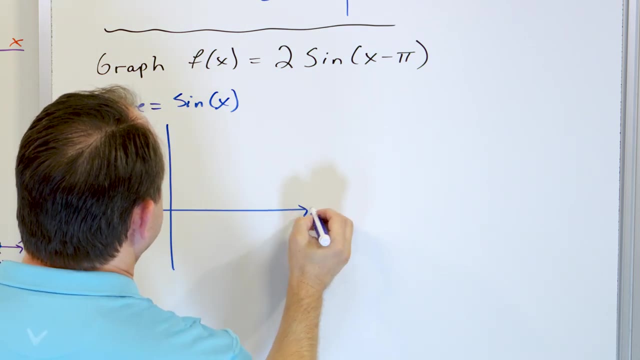 base is equal to sine of x without any real changes to it, right, And then we will put our changes to it to see if we can do it. So here we have x and here we have this graph of sine of x, And we. 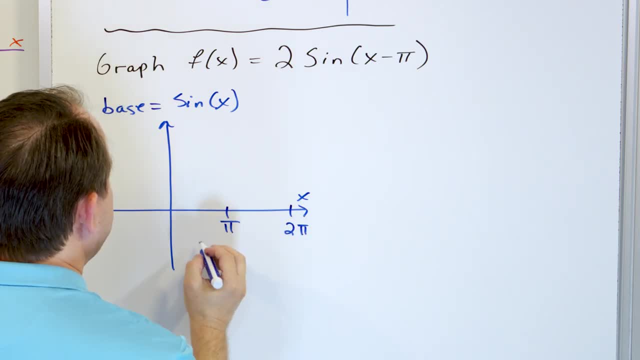 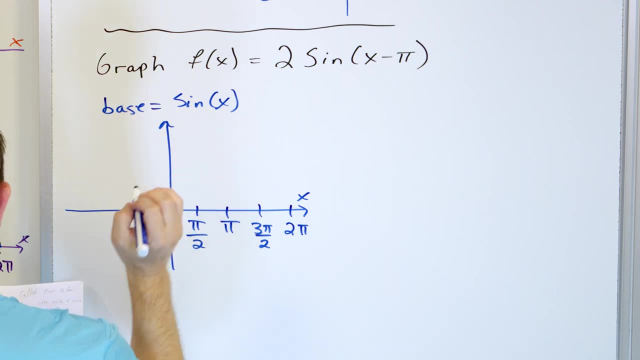 have done this so many times. You know, 2pi is a period And this is pi right here, This is pi over 2.. And this is 3pi over 2, like this. And then it goes up to here's 1, here's: 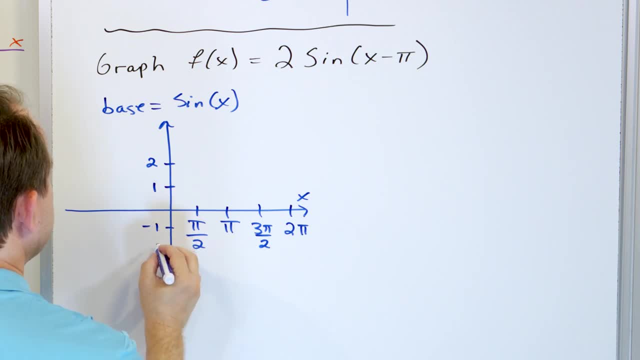 2, 1, 2.. And then negative 1, negative 2.. So negative 1, negative 2.. Now what I could do is I could just literally draw the base sine. It goes up to 1 and so on, But just. 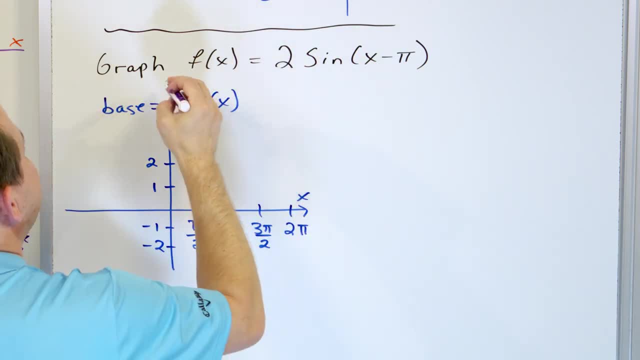 to, because we're learning about phase shifts. let's just graph, Let's call the base function 2 times sine of x, So we can see what 2 times the sine of x looks like. And then we'll handle the phase shift in the last step, Because the sine is going to go up to its maximum. But the maximum is: 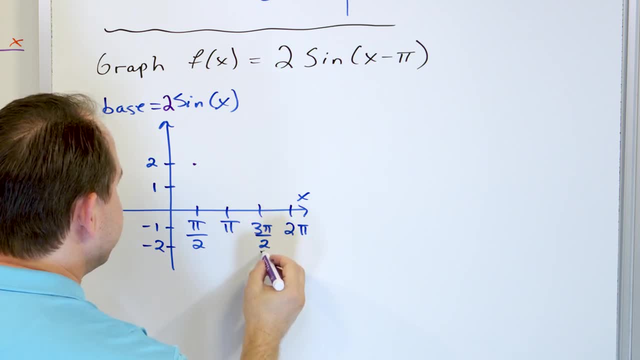 now going to be 2.. And it's going to go down through here And the minimum is going to be negative 2.. So it's going to go up to a maximum, down through here to a minimum and then back up, like this: 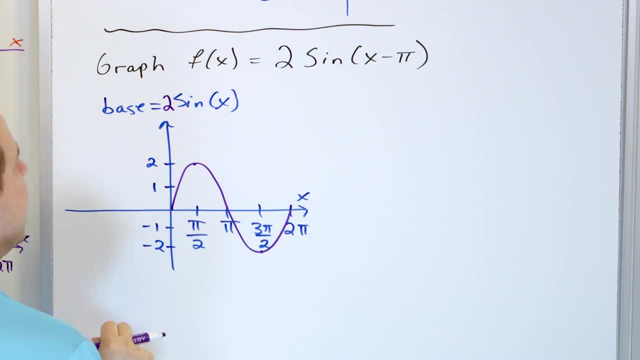 It's a sine, so it starts at 0.. Minimum, a maximum Minimum, And then back around to its starting point. in 2pi. There's nothing in front of the x to increase the frequency or change the period. The period is the normal period of a sine function. 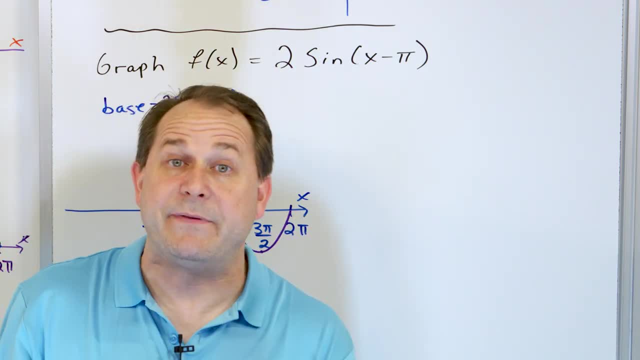 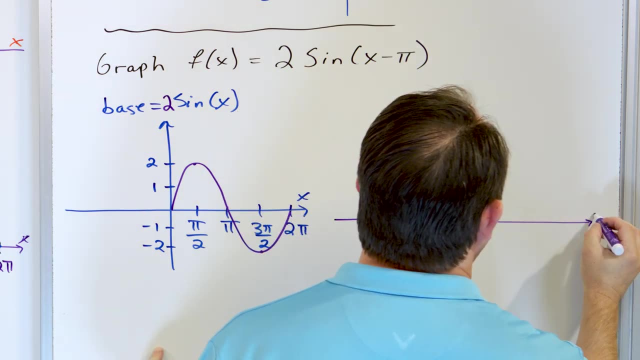 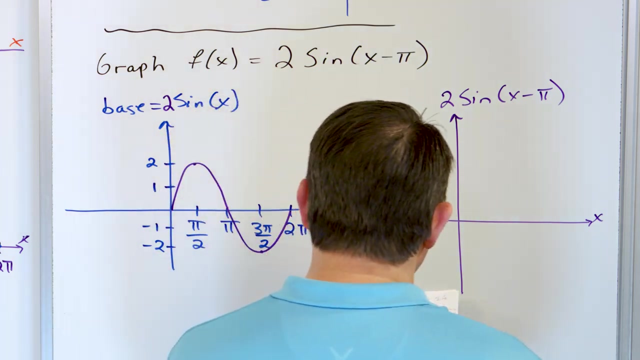 So I'm going to call this the base. What I mean by that is everything except the phase shift. Now let's go on and draw what the actual full blown function looks like and see how close we can get. So x. and here's f of x, which is 2 times the sine of x minus pi. 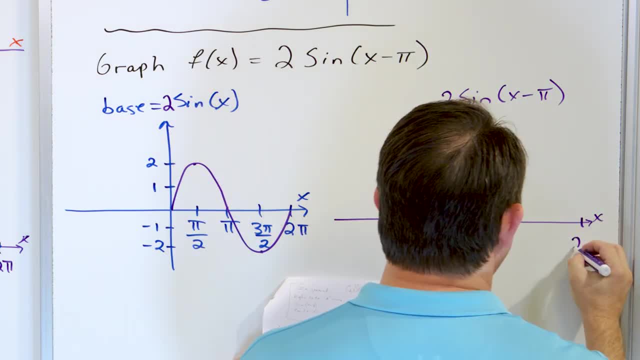 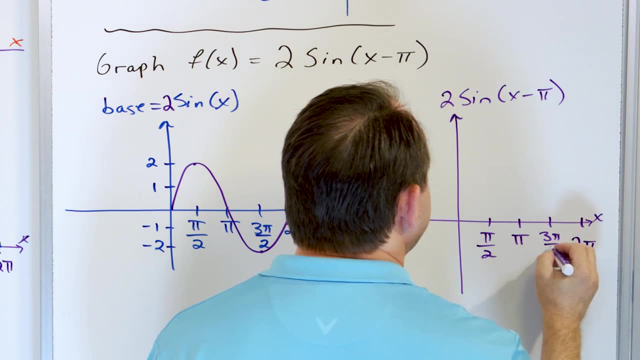 So what we can say here is we have 2 pi, and then we have pi right here, and then we have pi over 2, and then we have 3 pi over 2.. Now we know this thing is going to go up to 2.. 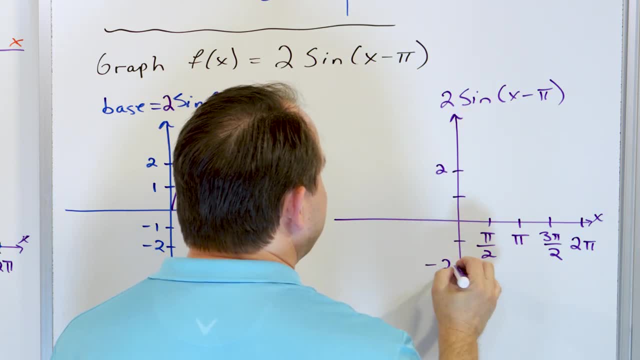 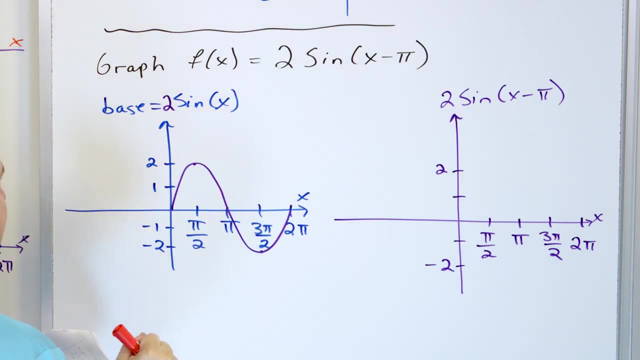 So here's 1,, here's 2, and here's negative 1,, here's negative 2, like this Now the normal function, we already drew it right here- it starts and it goes up like this: So shifting by pi is basically going to be the same as grabbing this purple curve and 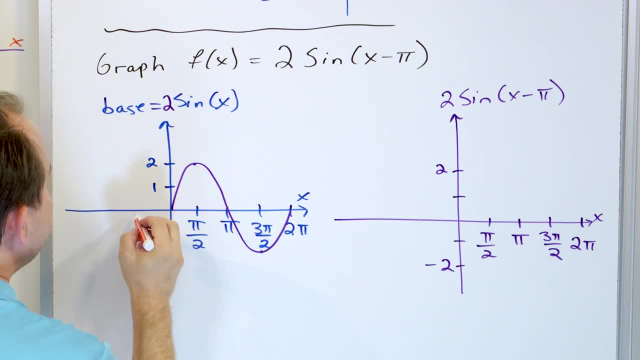 moving it to the right Now again, because we're moving it to the right. it would be nice if you have negative pi over 2, you have negative pi right here, if you just kind of remember that this is going to go on the negative side up like this right. 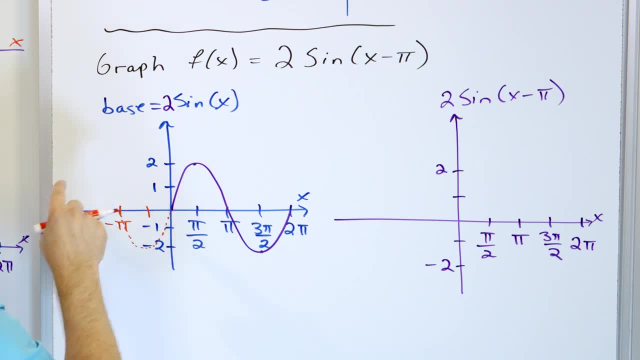 Because when you grab it and move it to the right, it's kind of helpful to have what's over here kind of in your mind. So what's going to happen is when you grab this thing and move it pi units, this point is going to be here, this crest is going to be pi units over here. this entire kind of 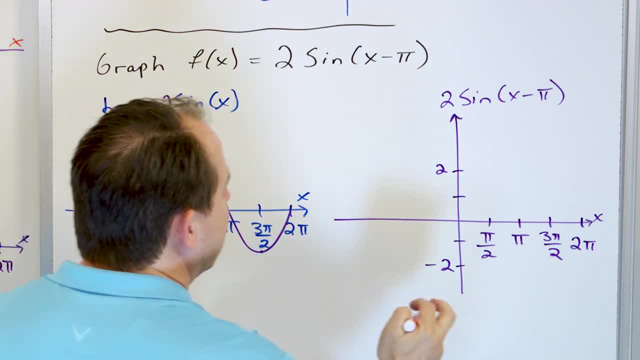 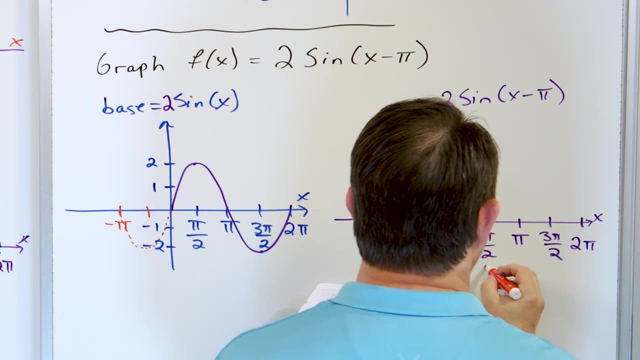 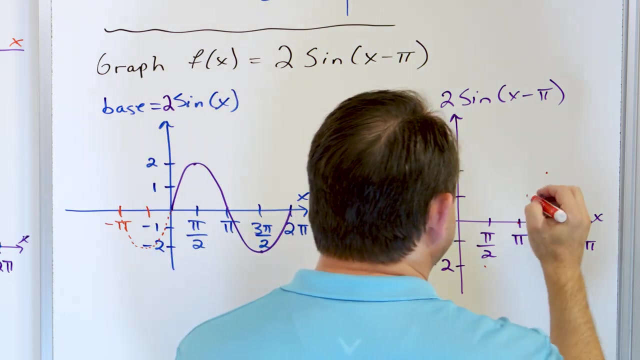 upside down. part is going to be moved, pi units, which means it's going to be over there. So what it's going to do is it's going to go down and then up through pi, like this, like this, and then over here is going to be a maximum over here, and then it's going 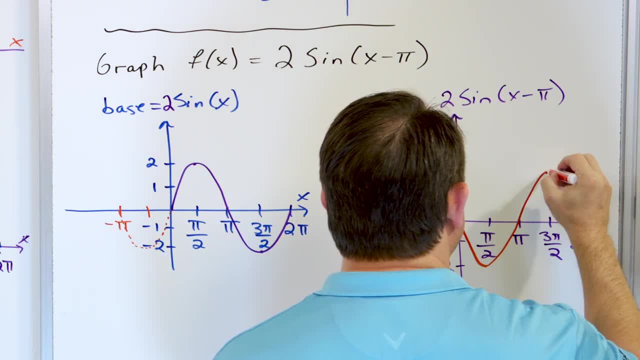 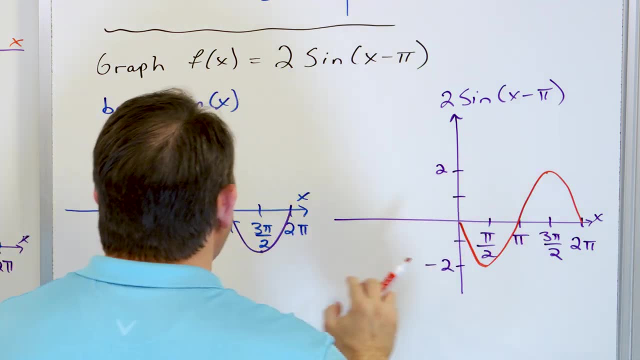 to go down. So it's going to go down here, then up here, then down here, like this right Why? Because we grab this and we shift it, so we know it's going to be like this. we got this and then this one is going to be moved again- pi units over here, so it's going to go and 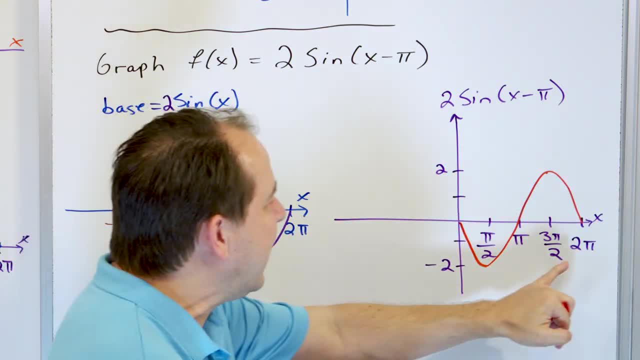 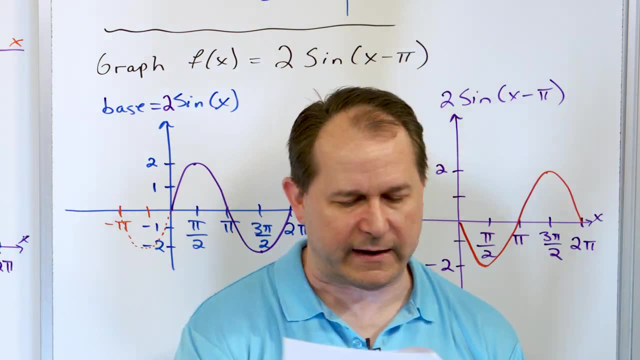 continue like this. So it's going to go down, then up, then down, And of course I stopped it here at 2pi. but I could go to 4pi and just give me. I could give another cycle, I could give it a minus 2 or carry it as far as I want to in the um, in the, in the x direction. 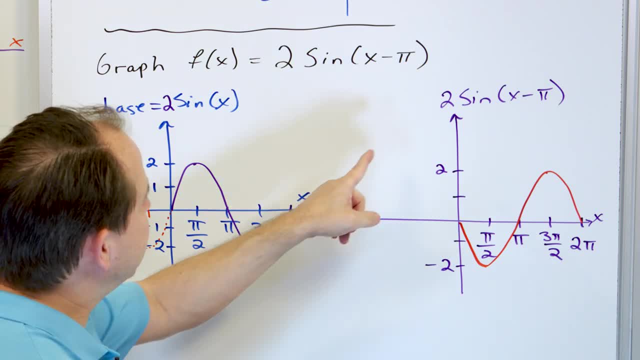 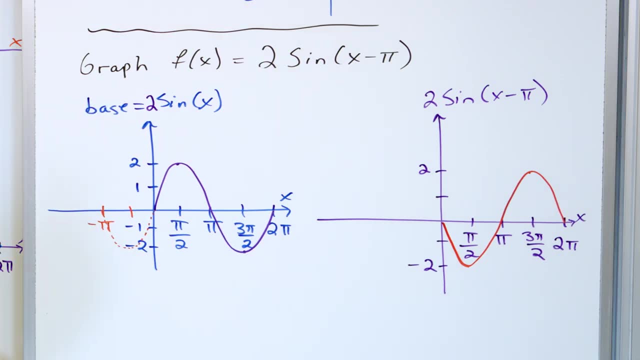 here. Okay. So let's just double check and see if this is correct. The shifted version: here, uh, is shifted to the right by pi and also is multiplied by 2, so it goes uh to plus or minus 2.. 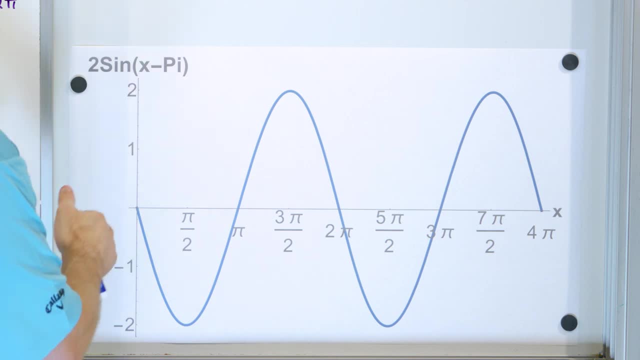 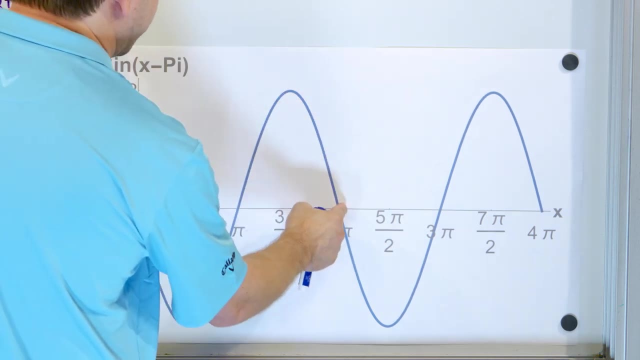 Let us see if that is correct here. So here is the graph: 2 times the sine of x minus pi, And so it goes down and up through pi and then to 2pi, And then here I took the graph to 4pi. 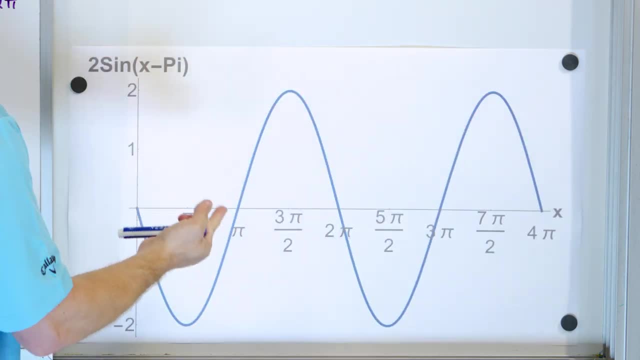 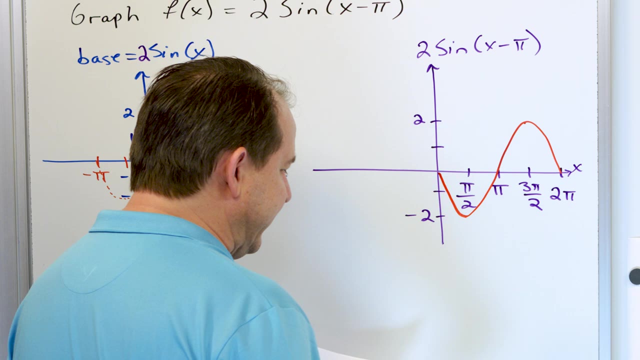 pi. so I gave myself another cycle just to kind of see what it looks like. But you see, it's the same thing, down, up, down like this. So let me point out something that we've mentioned many times before, and that is that when we 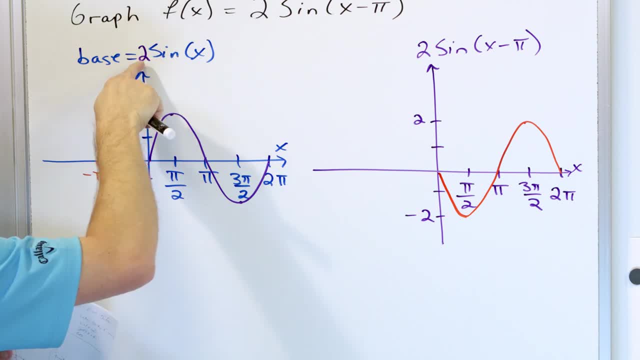 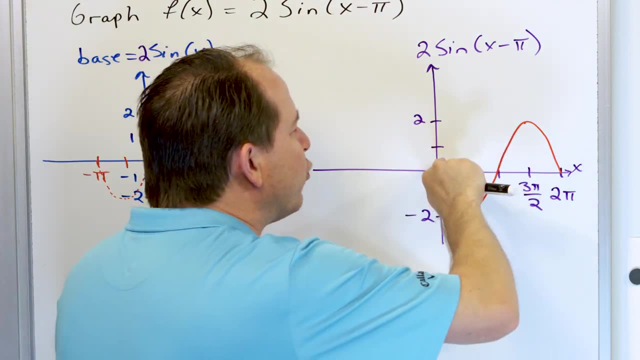 take a notice: what we've done is we have taken two times the sine of x and we shifted it to the right and what we end up getting is an inverted sine Because, remember, the regular sine goes up. I mean, you can see it right here. it goes up like this, but after: 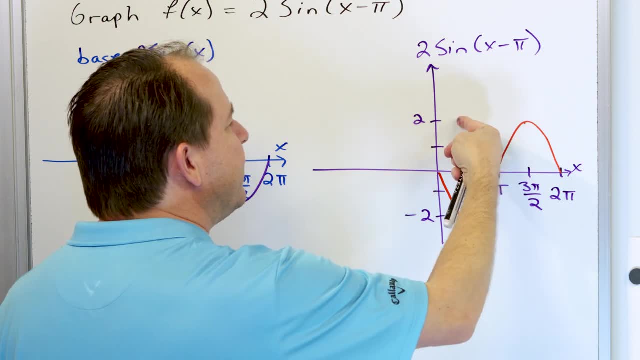 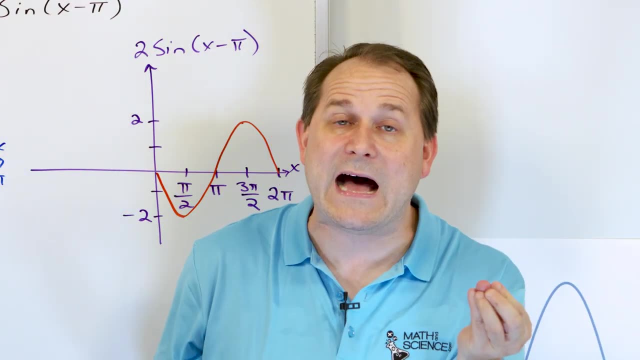 we do a phase shift of pi, it goes down, up, down, so it's like mirror image, reflecting everything that we had right. It's like flipping it upside down, And any time you shift a sinusoid by pi, you get the same function back, but flipped upside down right, Because you're 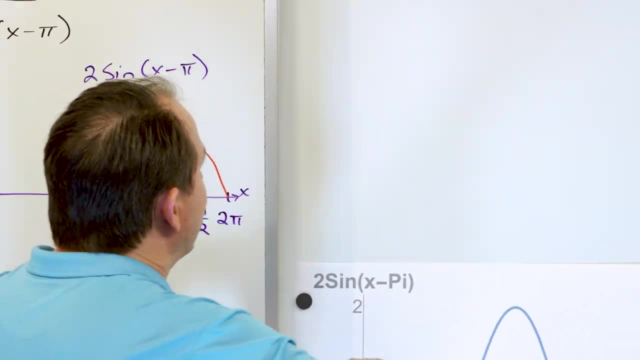 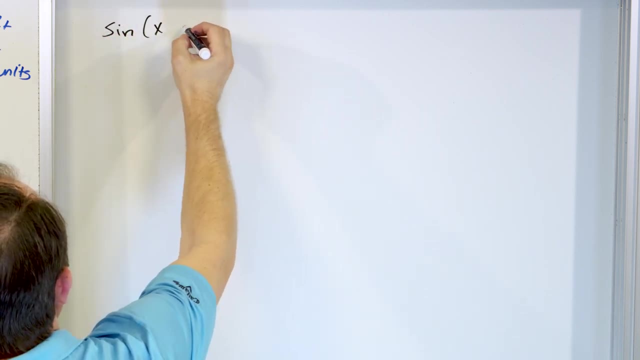 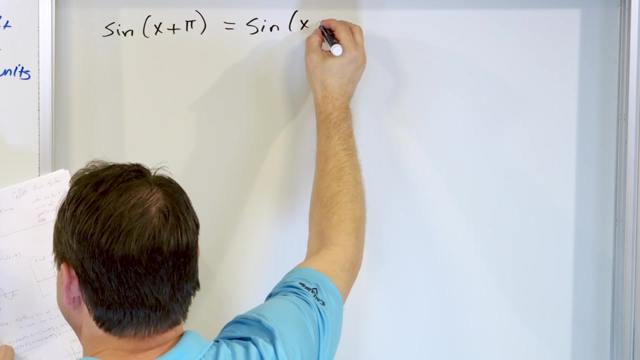 shifting it by half of a period. So basically, what we have learned by doing this is if we take the sine, and if we take it and shift it to the left with a plus sign by pi, we're going to get the same thing as if we take the sine function and if we shift it to the right by pi, which what we're 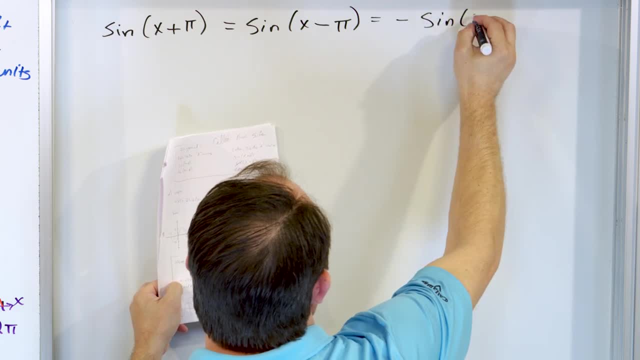 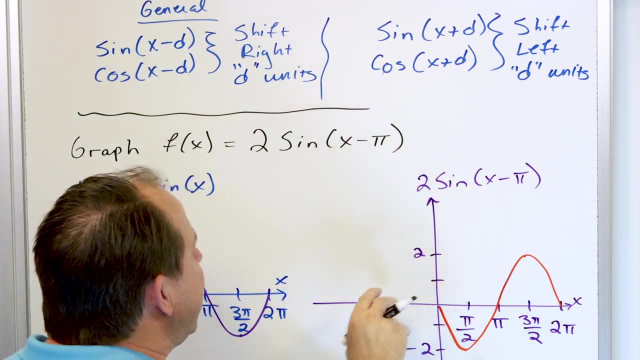 going to get back from. it is going to be negative sine of x. We just take the original function and flip it over with a negative one. You can see that we've taken this and shifted it to the right by pi, which is exactly the same thing as flipping it over And the same 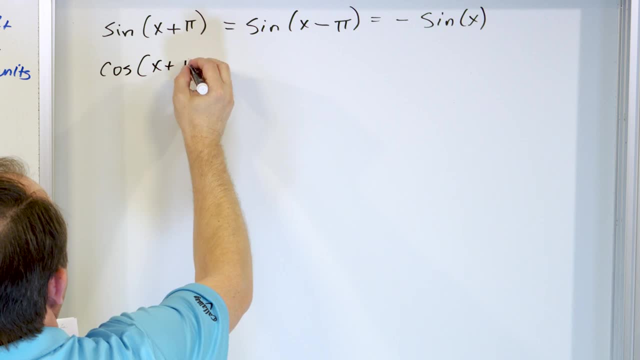 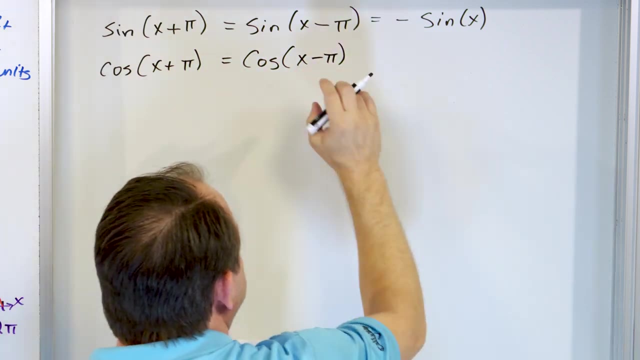 thing is true of cosine. So cosine of x plus pi is exactly the same thing as cosine of x minus pi as a phase shift. So a phase shift of plus or a minus pi gives you the exact same thing, which is negative cosine of x. 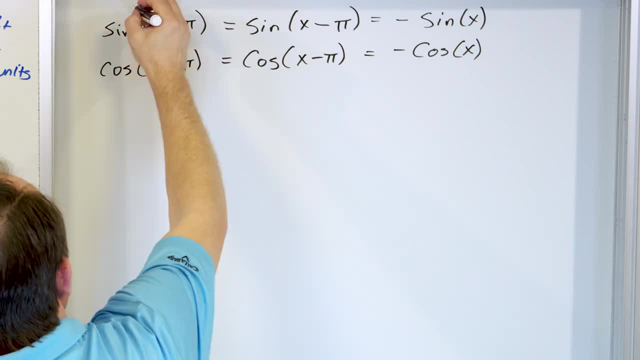 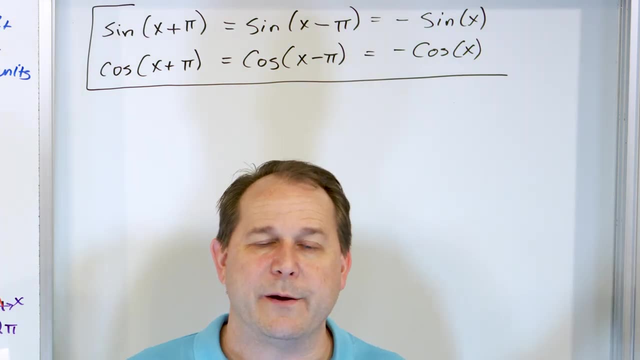 So if you take a sine and you shift it and these are another set of identities. I told you there's a lot of identities you learn in trig, But most students, including me, when I learned it, I didn't know where it comes from. I was like, OK, thanks, I really appreciate. 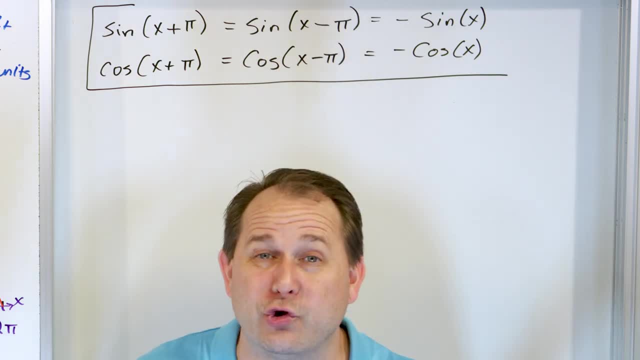 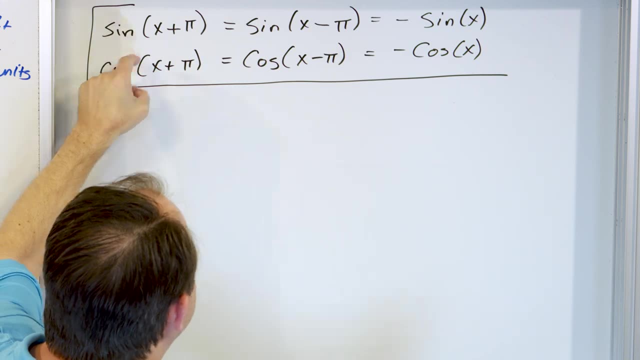 it, But I don't remember or know where. maybe I never learned where they came from. They come from the fact that these are phase shifts And the regular period of a sine function is 2 pi. So if I shift it by pi, I get a negative cosine of x plus pi. So if I shift it by pi, I get 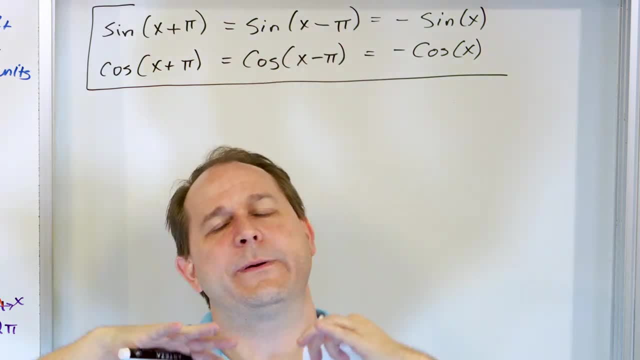 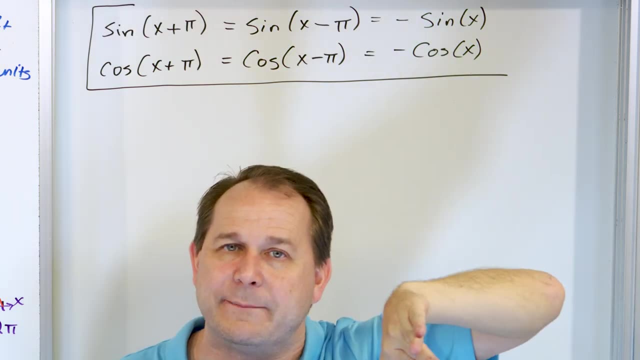 by half of that, Then all the crests are just going to become troughs, which means I just multiply by negative 1 on the sine, because that I already know from before is what flips it upside down. But because the period is 2 pi, if I shift by half of a period one way, 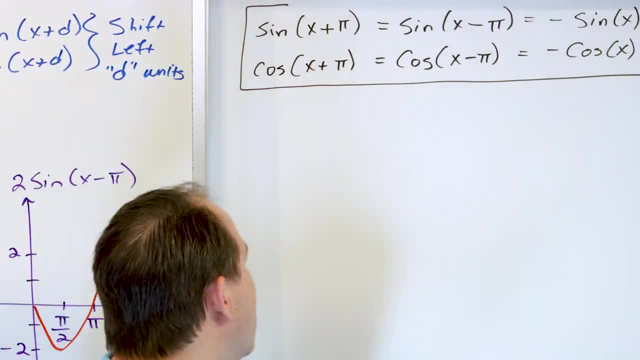 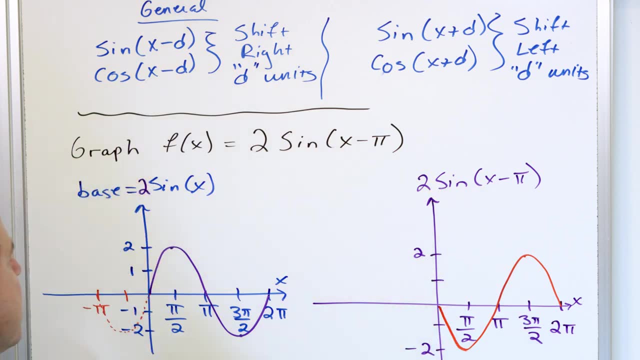 it's the same thing as shifting by half of a period the other way. I showed you that on the computer Here. I grabbed this guy and moved it half of a period to the right, And this is what I got. But if, instead of moving it to the right, I move it to the left, 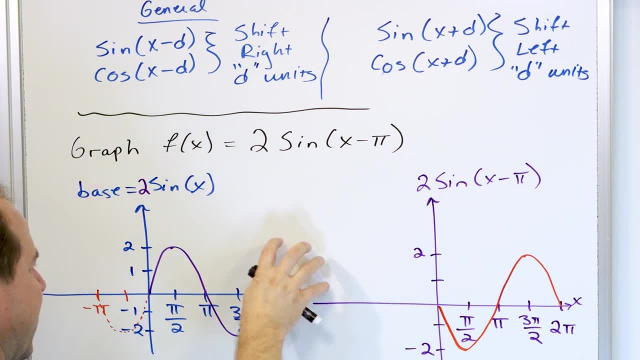 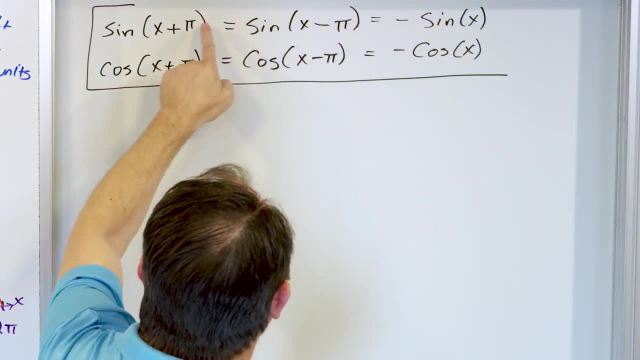 it would become over here, And what was over here would become over here, And I would get exactly the same thing. So this is the first one here. Shifting to the right by pi or to the left by pi, which is half of a period, just flips the sine upside down. That's how. 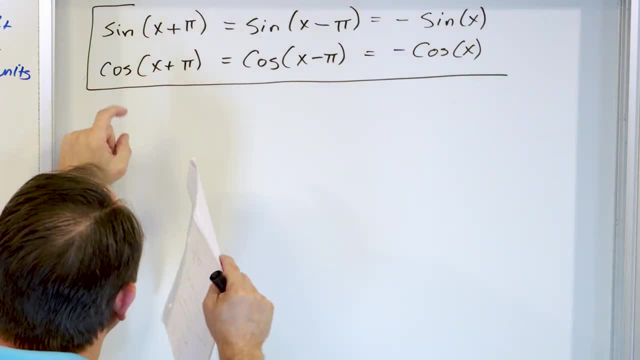 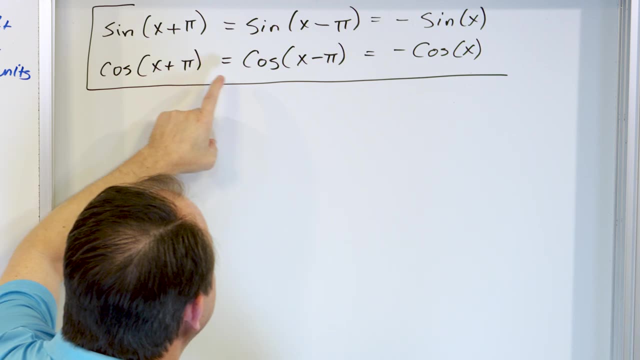 you translate the math into words. If I take a cosine function and I shift it to the right by pi, which is half a period, or to the left by pi, which is half a period, then I get the same cosine curve back. but 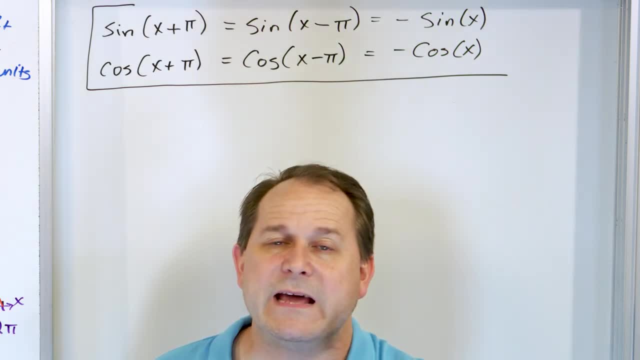 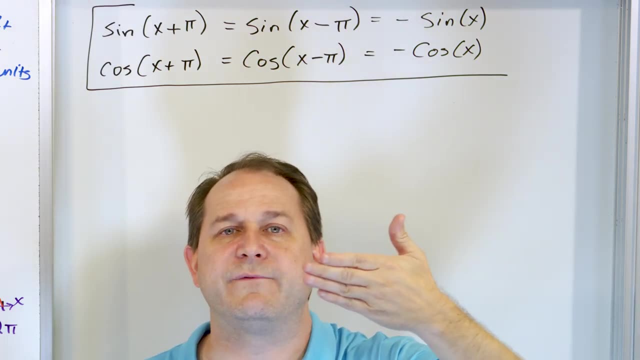 just inverted, Flipped upside down. So the point here is that you can shift a cosine or a sine half of a period, And when you do that, it's the same as taking an original cosine function and just flipping it upside down. That's what it means. 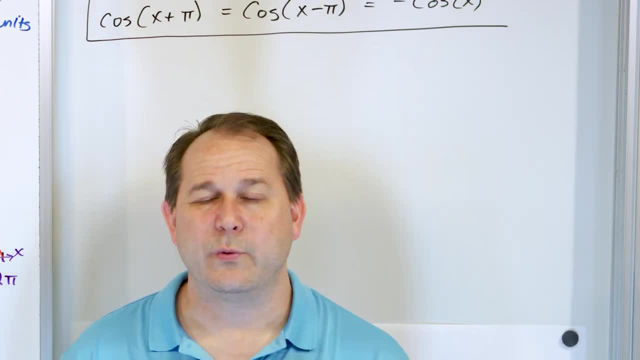 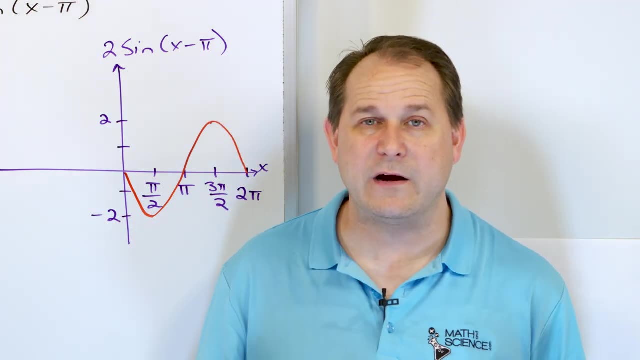 So we're done with this lesson, And in this lesson we have learned a lot. We have learned why shifting to the right and shifting to the left works. I showed you that with parabola, f of x equals x squared. We did the computer demo to show you how it works right And 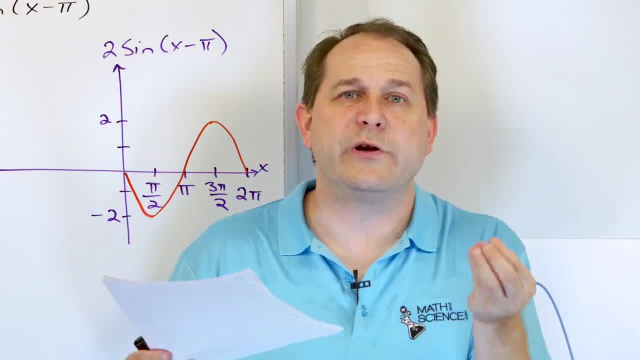 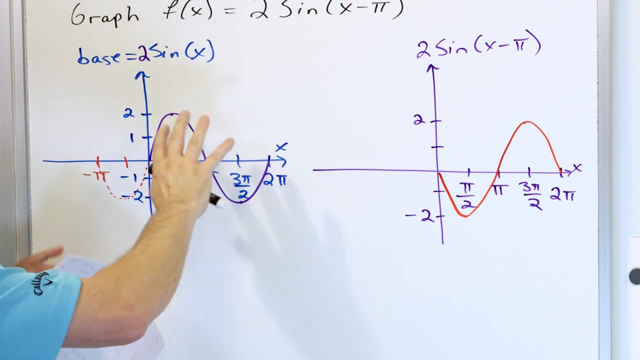 then here on the board, we get into the nitty gritty and really sketching them and just showing you how you would do it from a blank sheet of paper, without knowing what the answer is. And for all of these examples I sort of drew and sketched a baseline before I applied a. 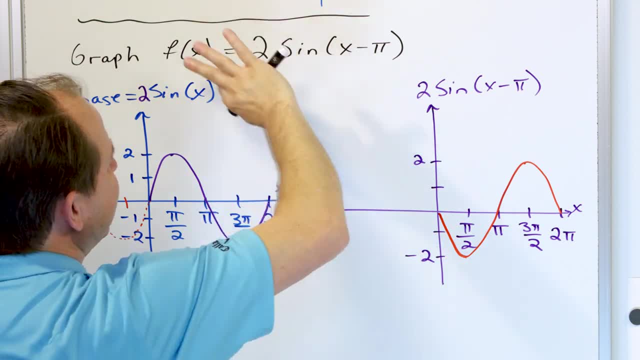 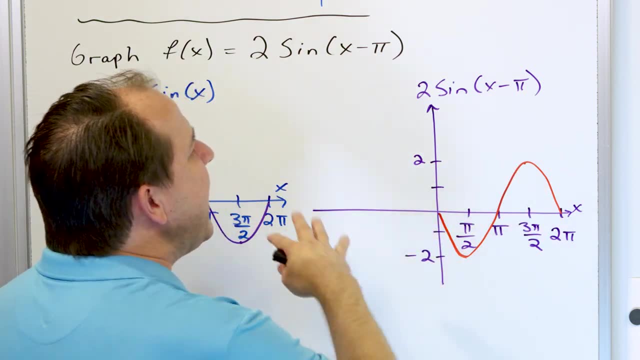 phase shift, Because if I try to shift while increasing this or maybe inverting it or something, it's very hard to do. So draw a base, visualize where everything's going to go and what direction, and then draw it, And then we learned some identities. 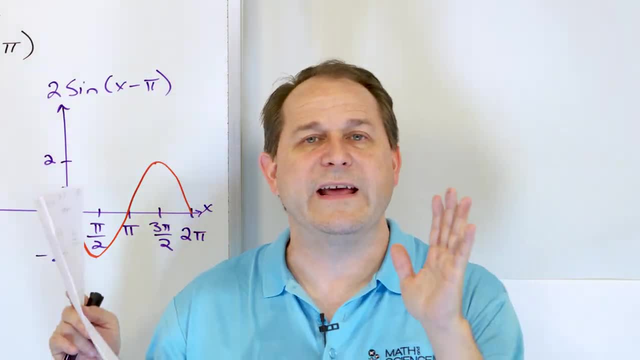 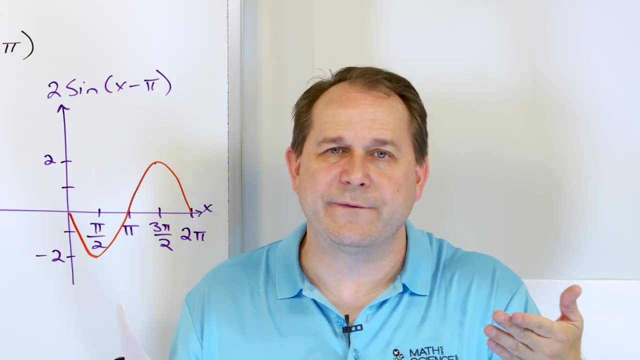 And the identities we learned. the main two ones that we learned here are as follows: If we take a sine or a cosine, shift it by half of a period, which is plus or minus pi. in either direction, we get the original function back, but flipped upside down with. 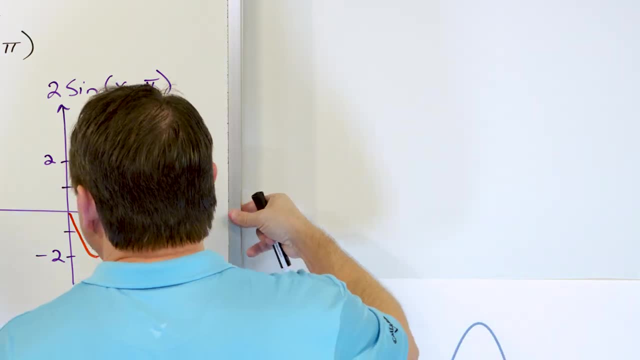 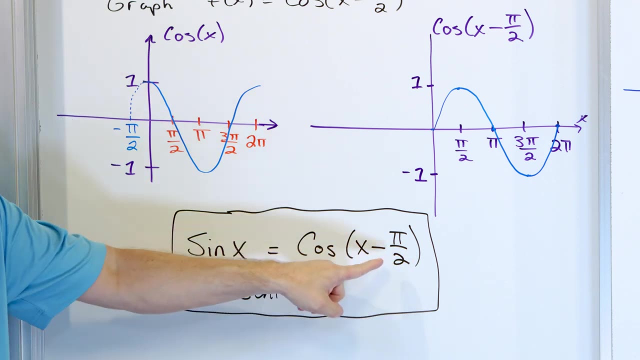 a negative sine. That is what these identities tell us. The other identities that we said is that instead of shifting by pi- if I shift by pi over 2, I can turn a cosine into a sine. And I showed you on the computer how you can turn a sine into a cosine either. You just